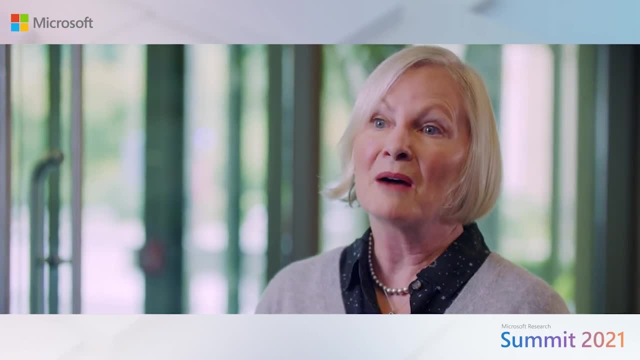 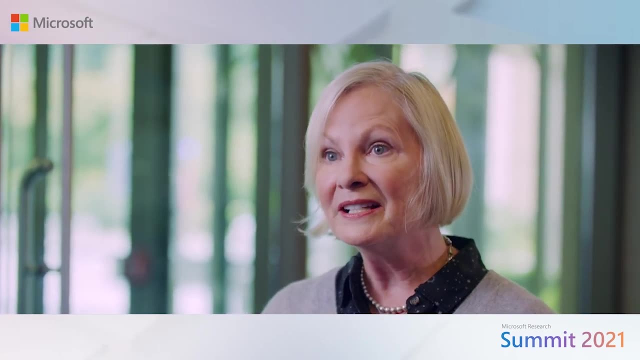 design, execution and assessment of computer systems and related phenomenon that are for human use. The goal of the discipline is to make sure that the technologies we develop are useful, usable, safe and enjoyable to interact with for all people, so that humans can achieve their tasks, whether that's to get work done. 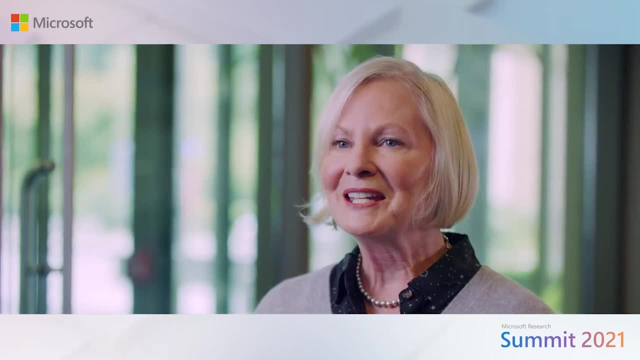 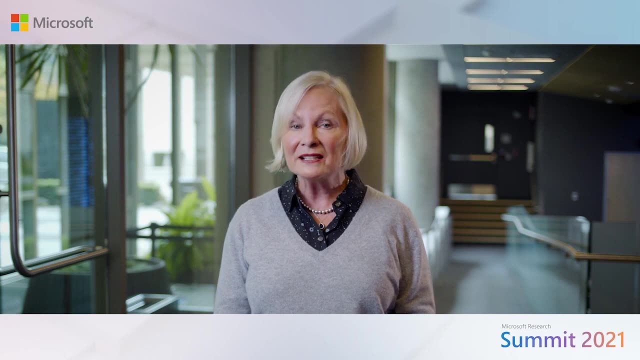 learn, be creative, communicate or just play. In order to fulfill these goals, tech companies must attempt to understand how people use technologies and build systems based on that knowledge, design or invent efficient, effective and safe interaction techniques for using new systems and put people first. 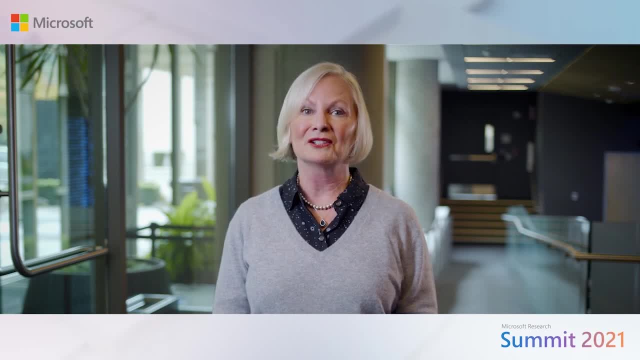 People's needs, capabilities and preferences should come before the technology. The new technology invented should be designed to meet users' needs and requirements first, not the other way around. Why is this important? A good user interface can improve financial outcomes because the experience can increase users' loyalty, trust and make users happy. 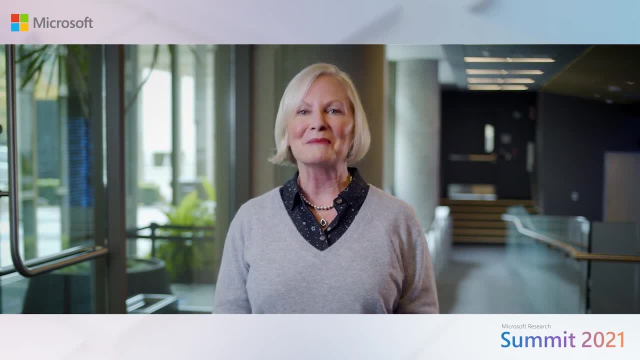 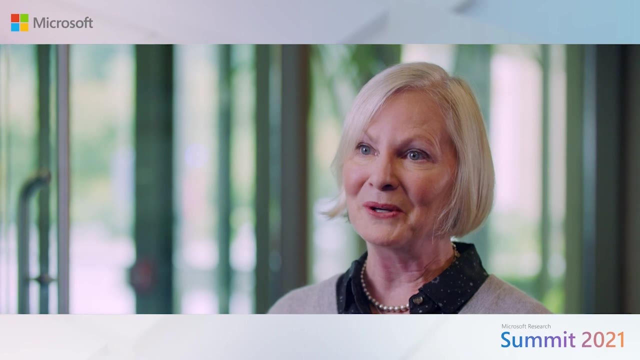 ensuring continued interaction with the system. We know this firsthand on my team because we study user emotion and we can see happiness go up when interactions with software allows users to get their work done more effectively. For example, we've seen evidence that users smile significantly more often when good search results come back quickly and users don't. 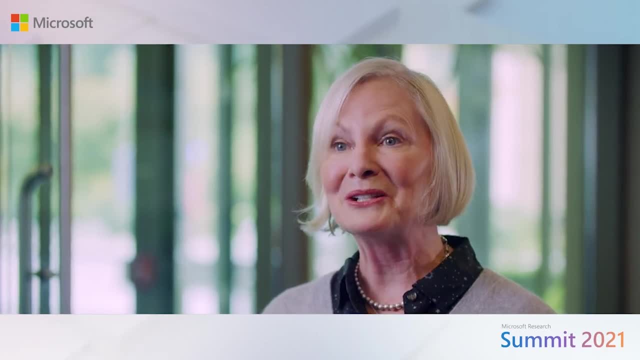 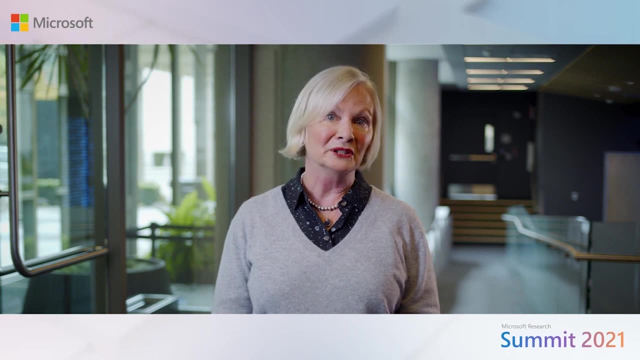 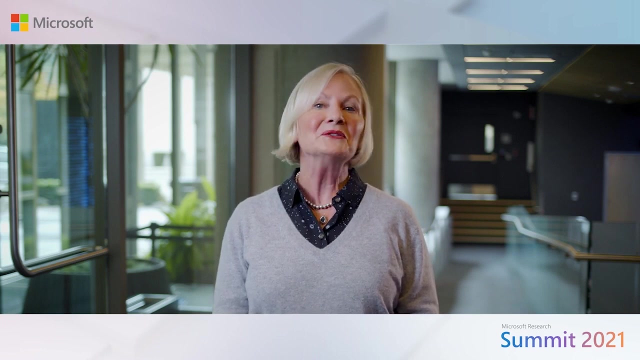 have to reformulate their search queries. Happy users come back to use software that pleases them. Most HCI researchers come from a varied background of multidisciplinary training, including computer science, obviously. psychology, because it studies people and the application of theories and methods, sociology, for understanding computer-mediated technology and, of course, 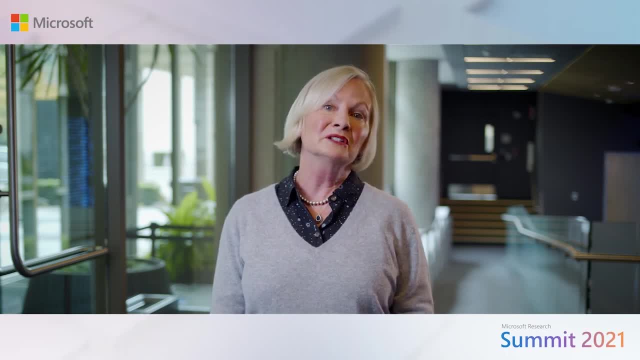 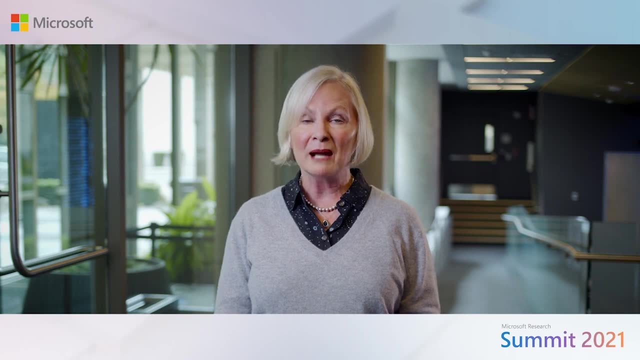 human organizations and even industrial design for the design of interactive products like cars, laptops, mobile phones, etc. As technology evolves ever more rapidly, human cognition remains relatively stable. It's important, now more than ever, to ensure that humans can use and understand the design of new systems as they emerge, especially with 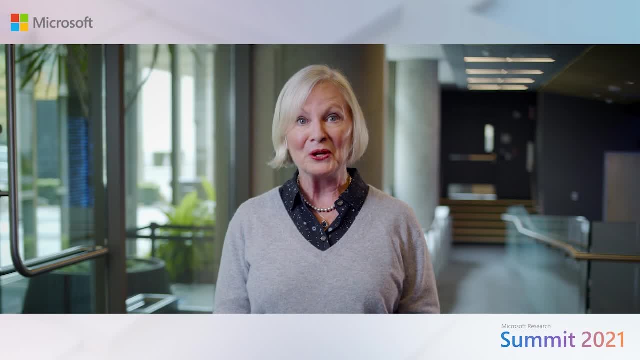 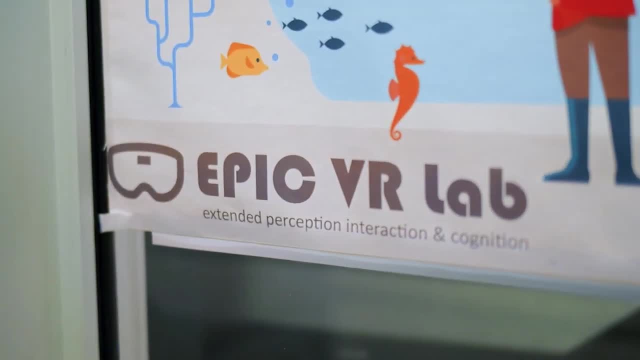 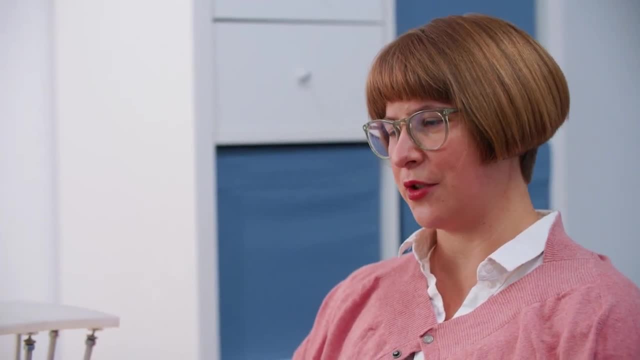 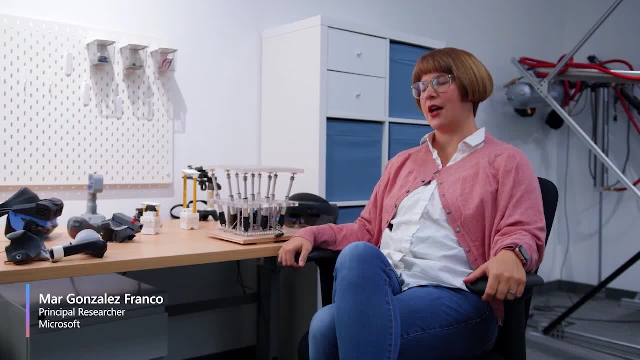 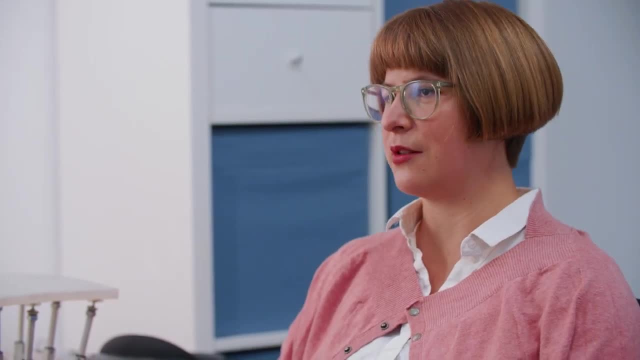 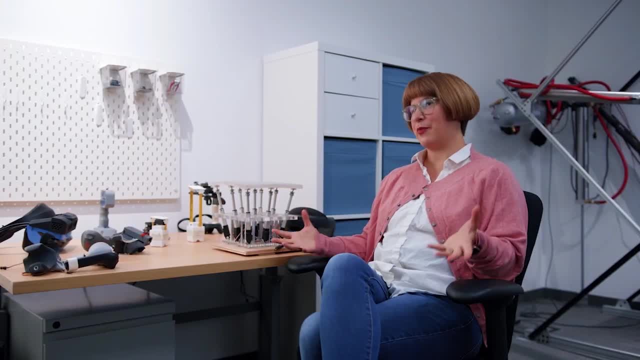 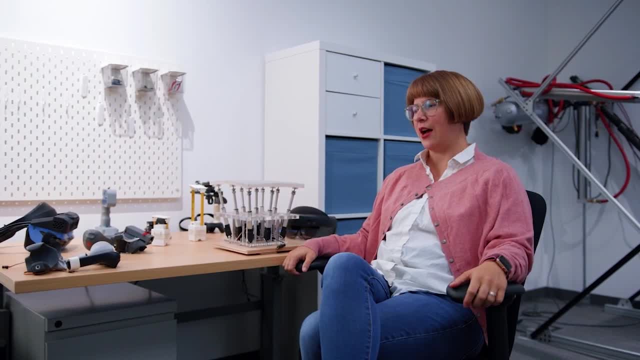 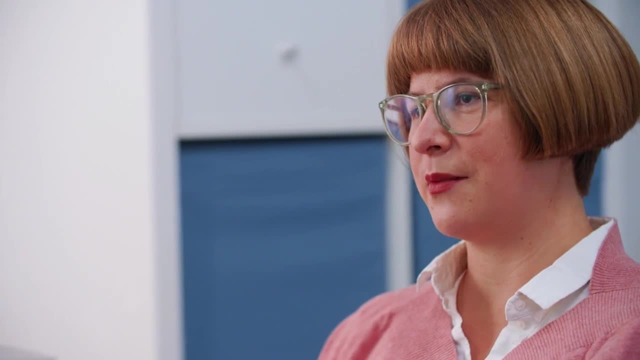 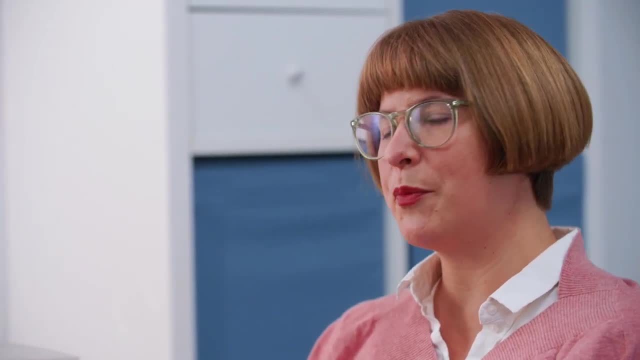 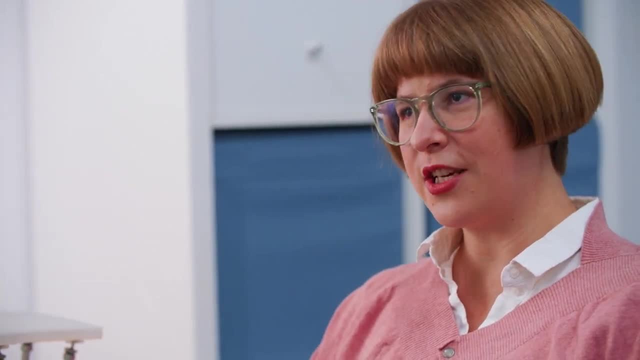 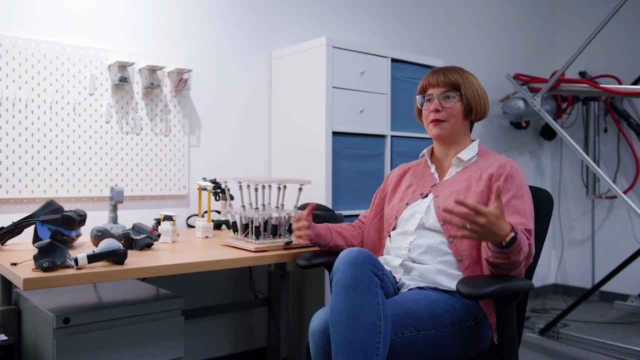 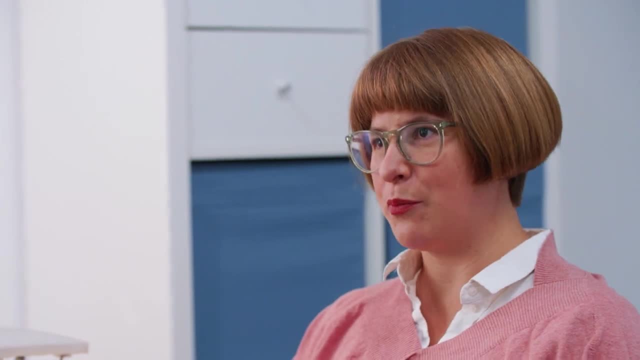 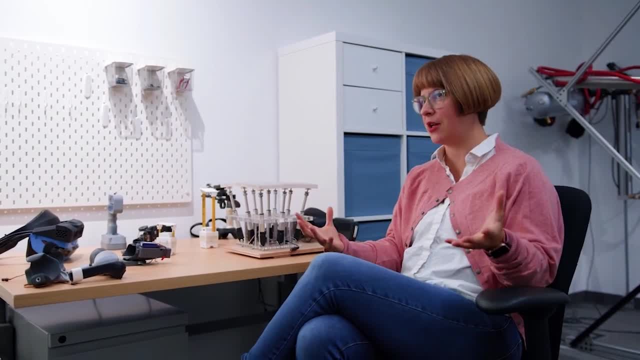 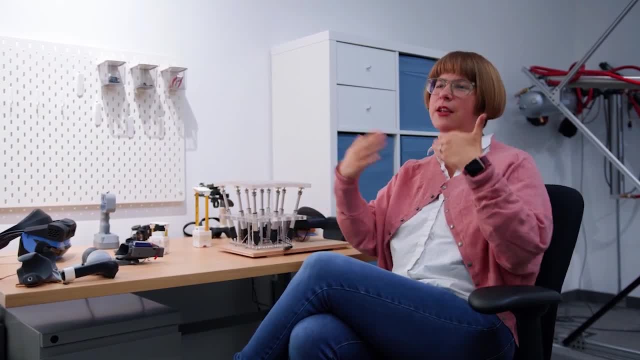 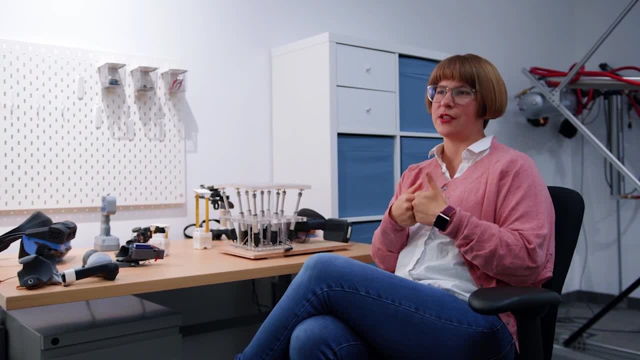 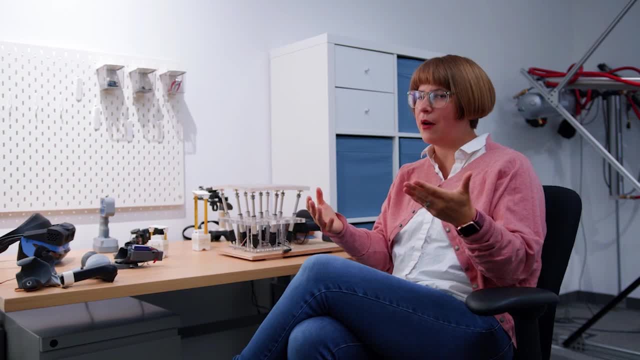 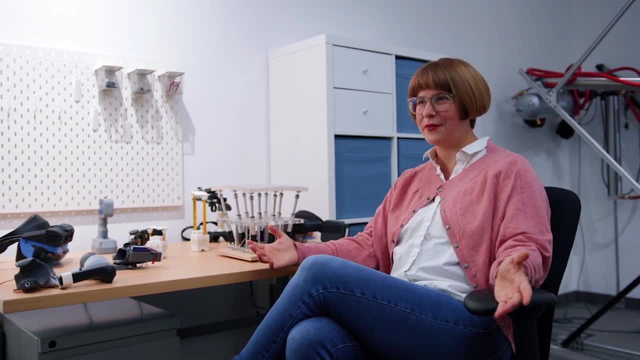 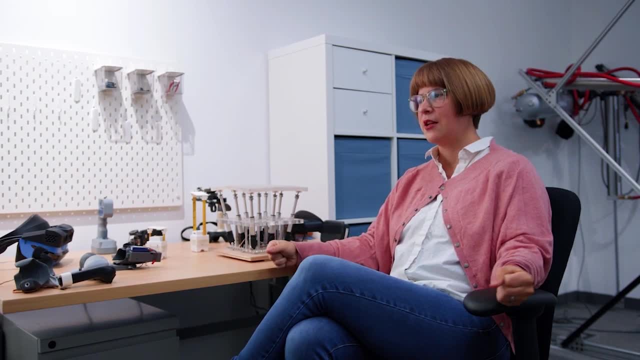 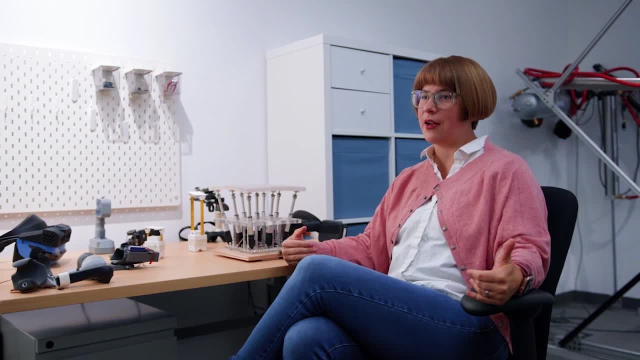 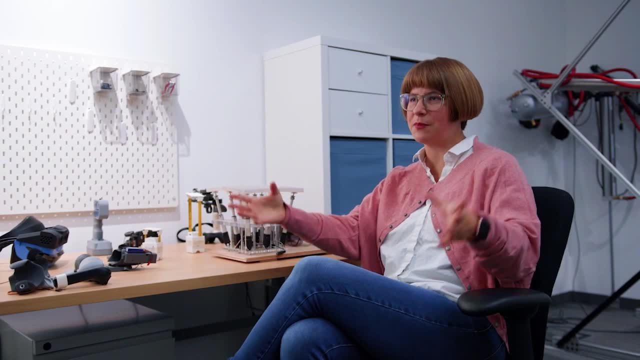 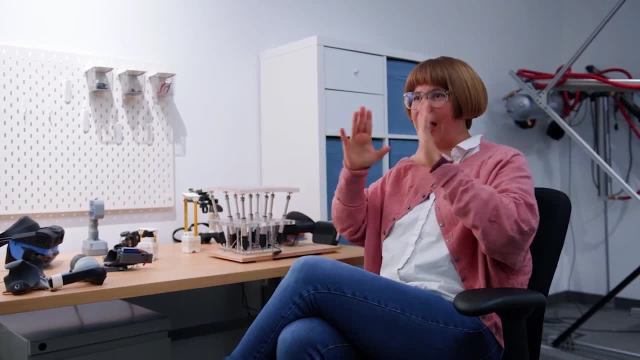 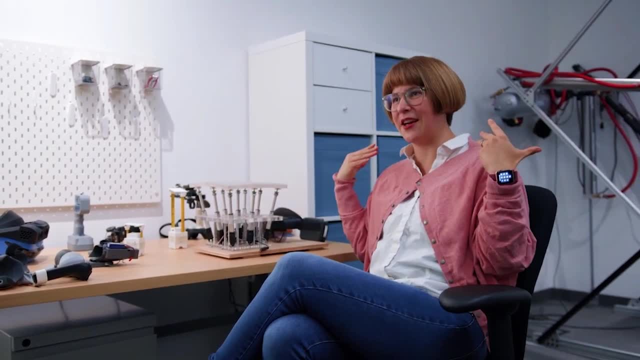 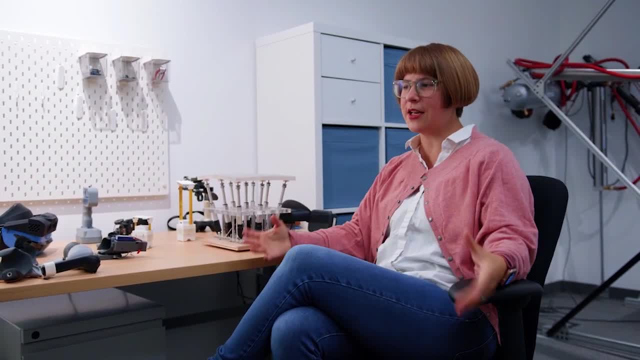 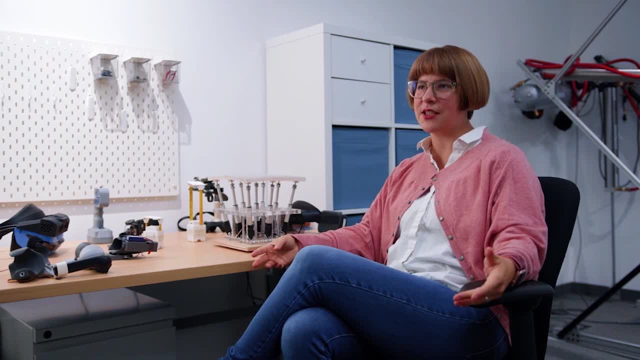 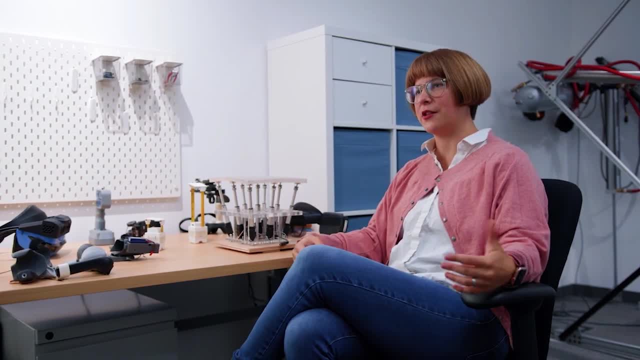 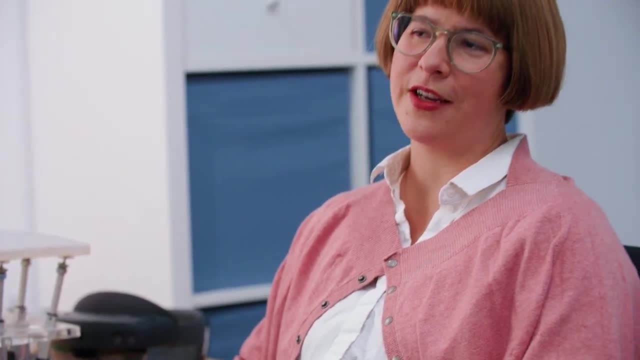 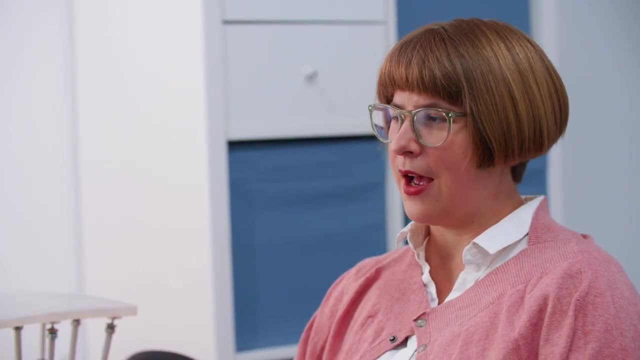 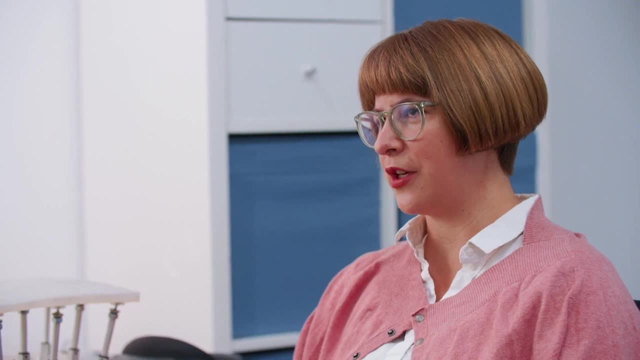 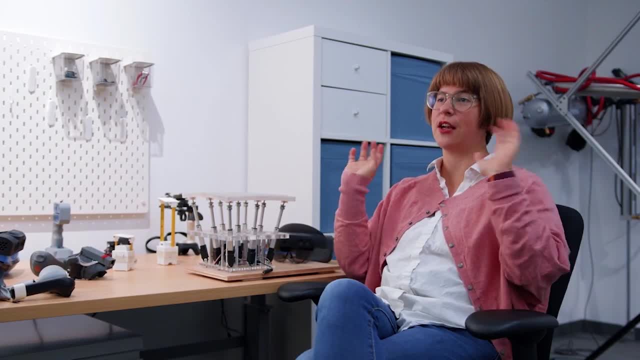 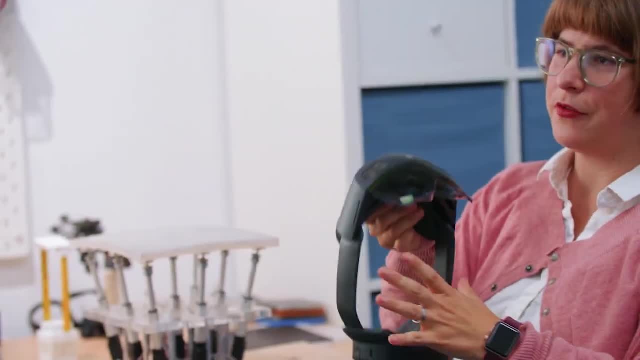 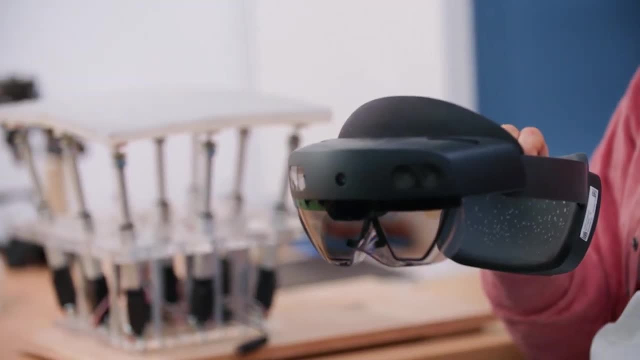 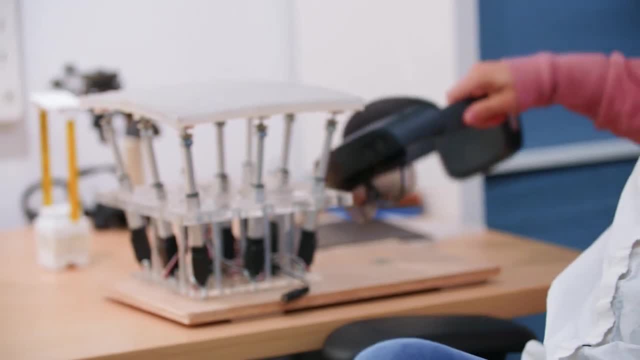 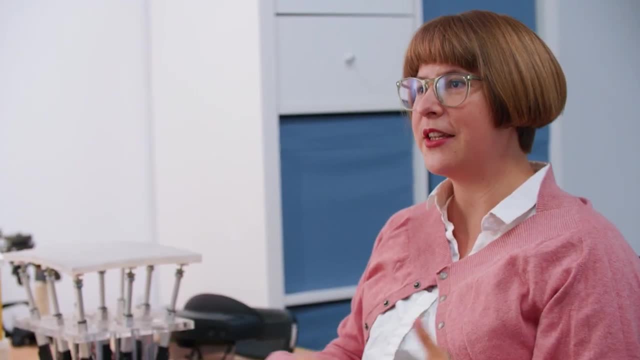 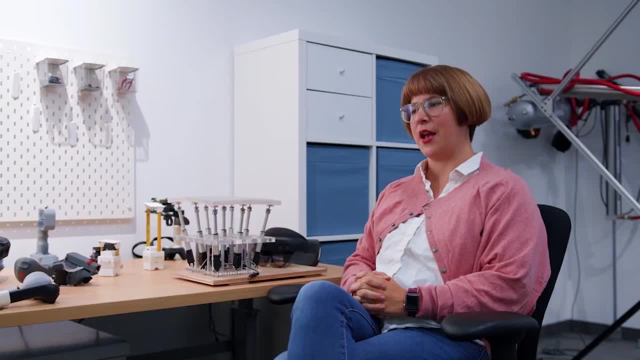 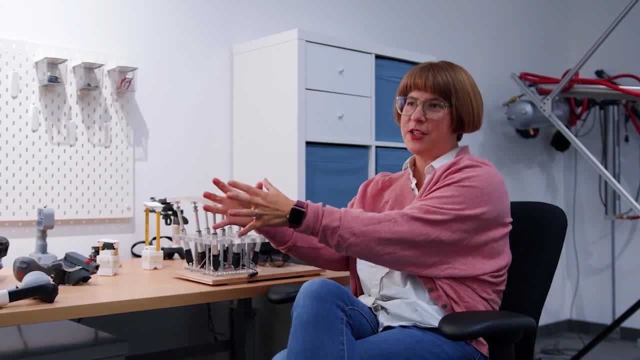 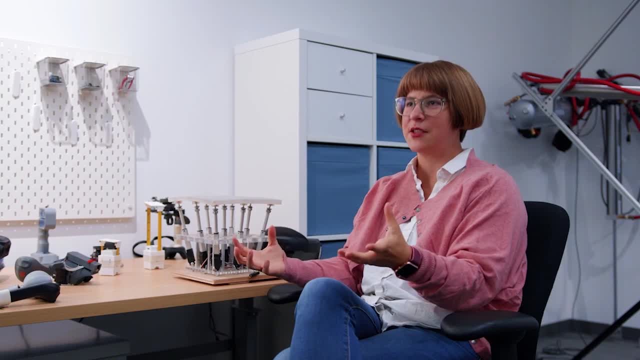 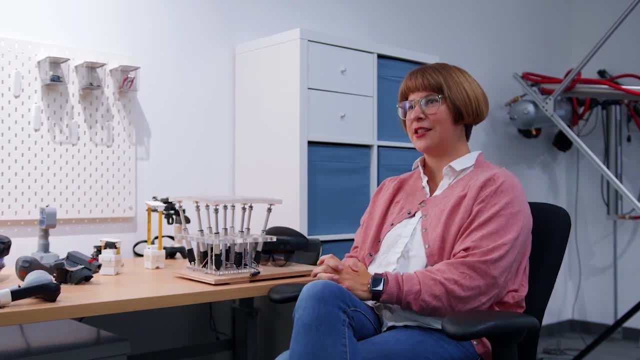 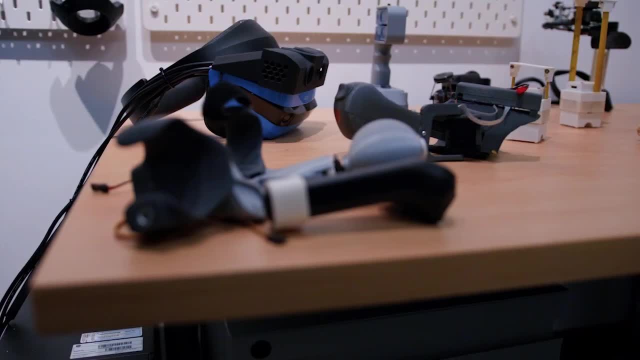 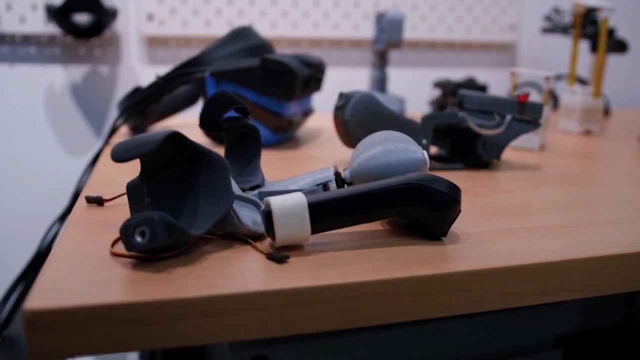 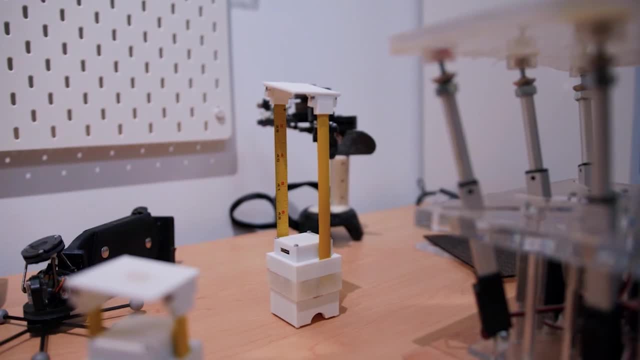 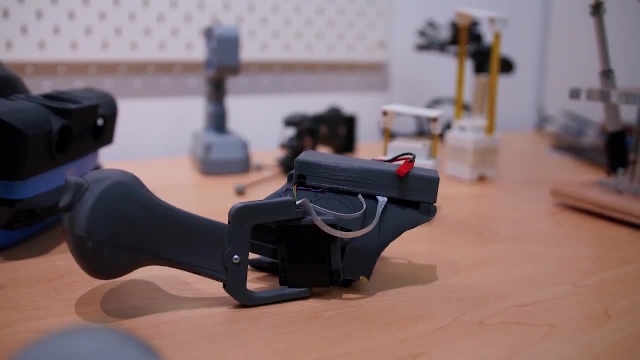 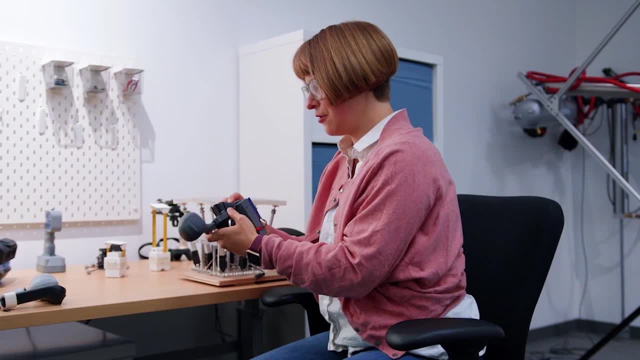 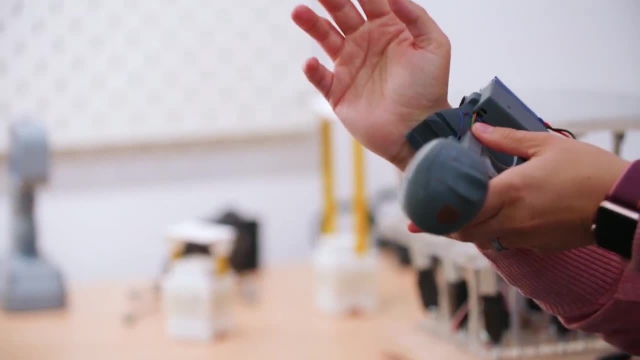 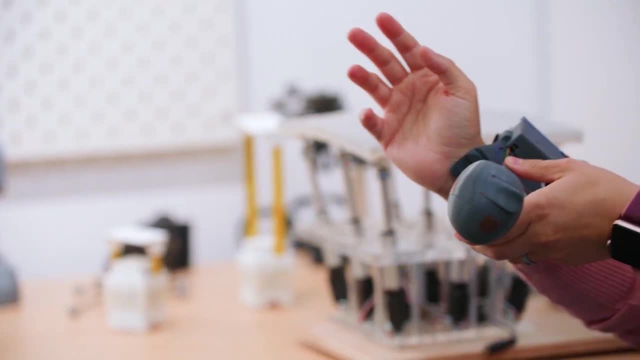 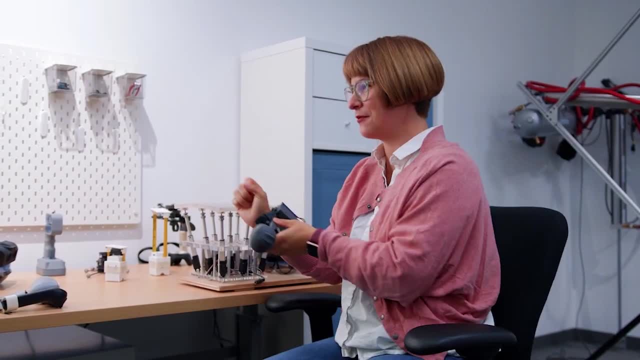 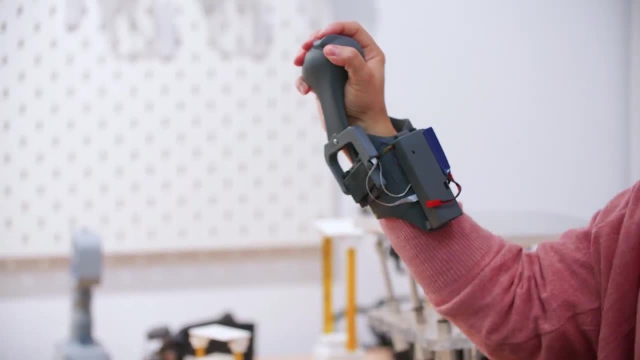 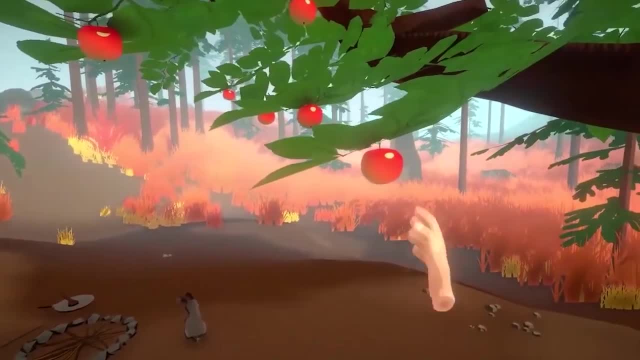 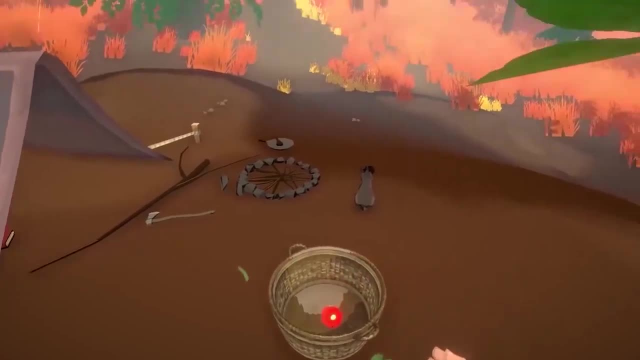 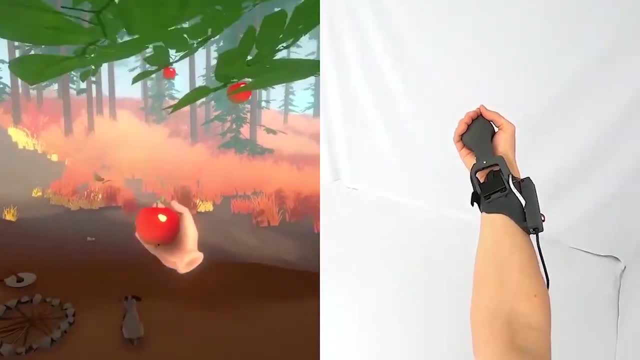 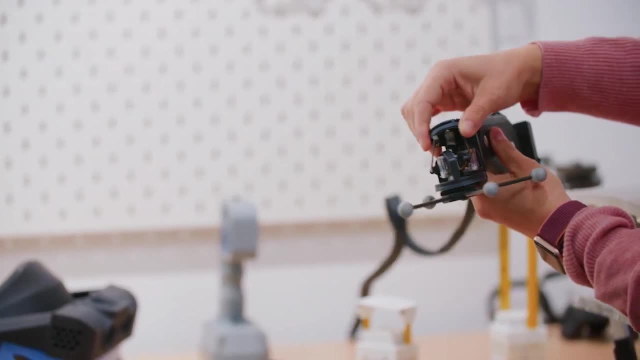 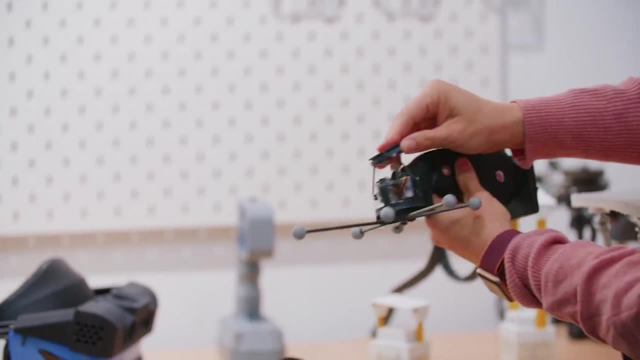 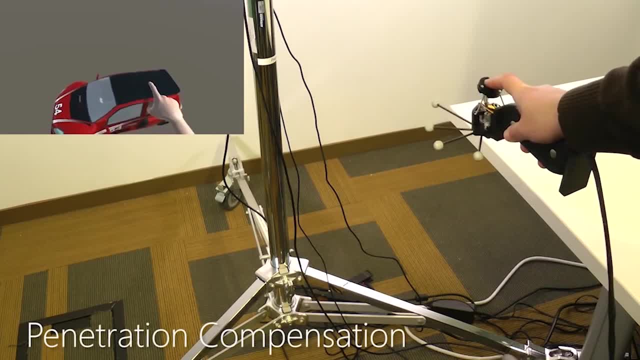 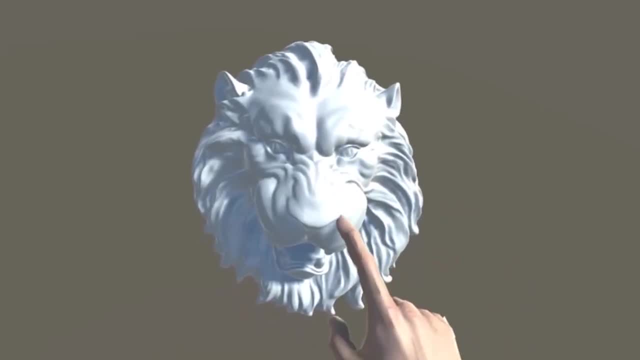 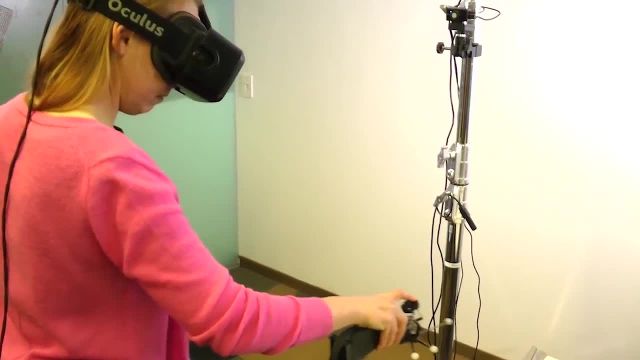 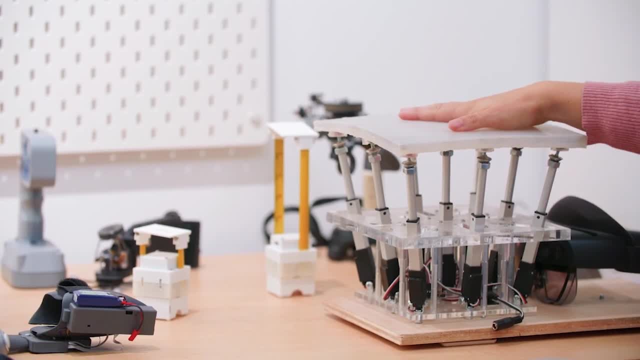 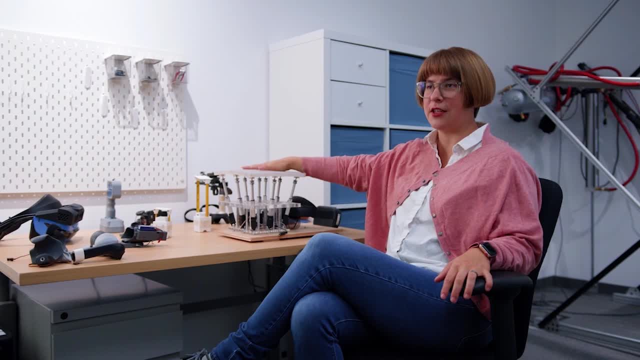 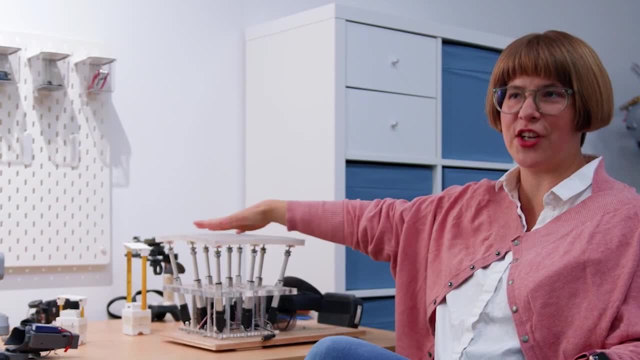 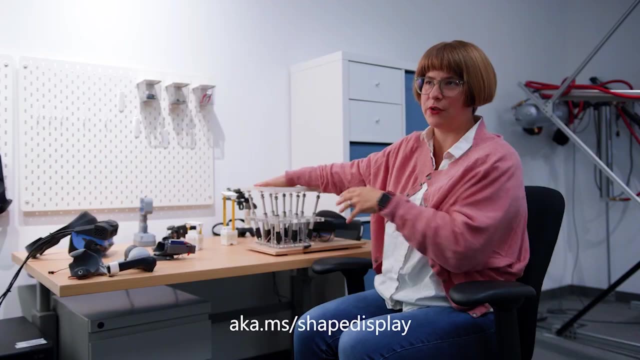 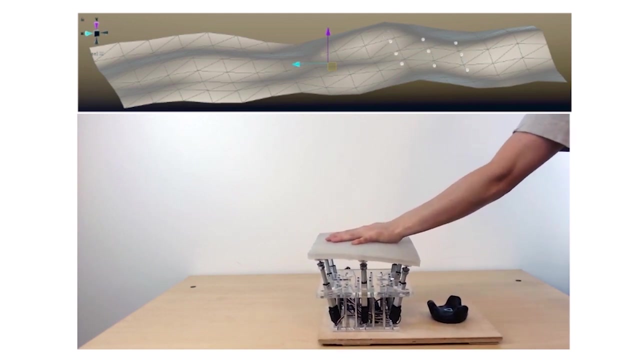 cognition. How do we, as a society, leverage HCI's new technology to improve human communication? We're able to reduce a shape display into nine actuators only by changing how we fabricate the materials on top of it. right, so you, you will touch, for example, a shape and move around and be able to experience a whole. 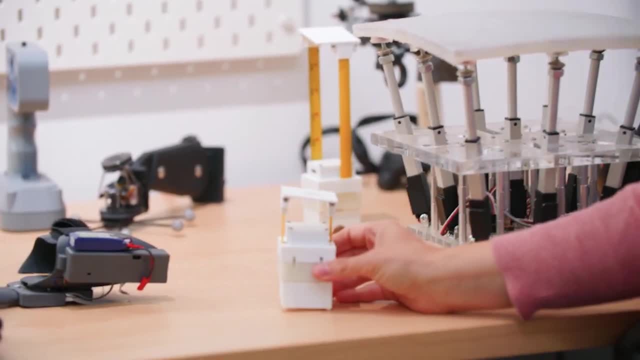 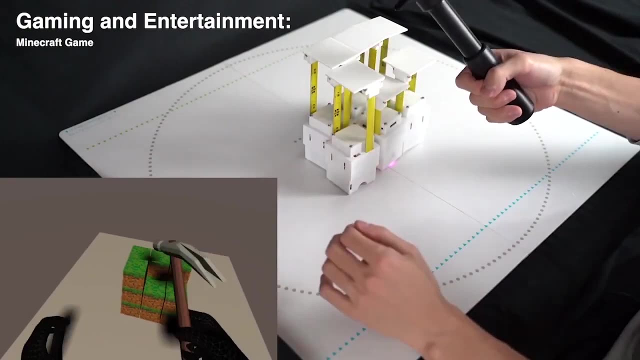 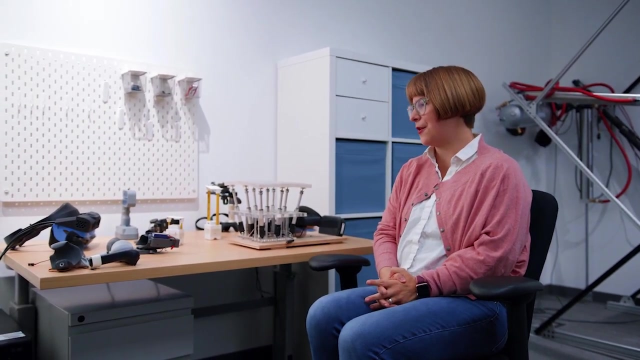 shape, and we have also these very cute ones, which are mini robots that come just in time for whatever you want to touch. So all of this is a nice set of prototypes, but there is science behind it, right. There are things we found, for example, like the uncanny valley of haptics, that you can go deep into this. 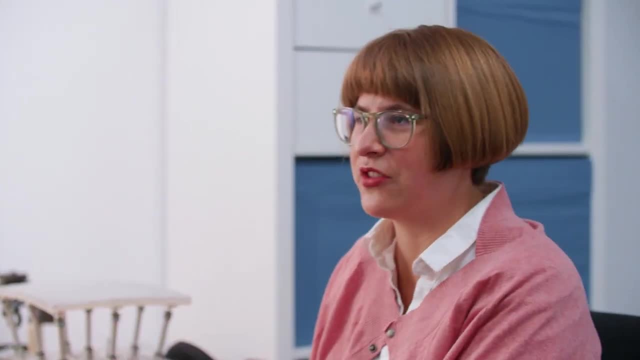 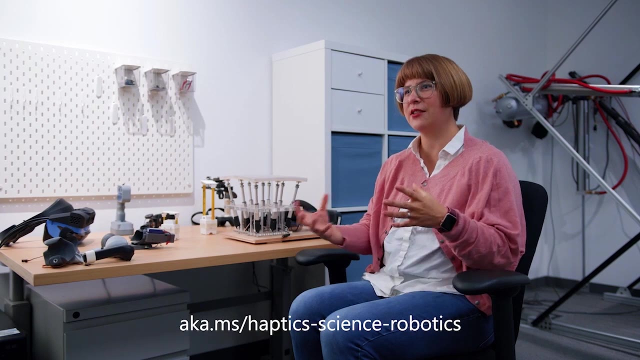 sensation that you break the illusion because the haptics don't match correctly what you're expecting. We publish that in Science, Robotics, and I think it's hard sometimes to find the right way to do it, Sometimes to detach theory from practice, because if you don't learn the theory, 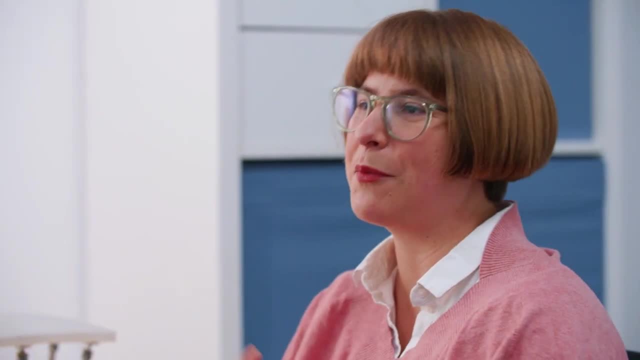 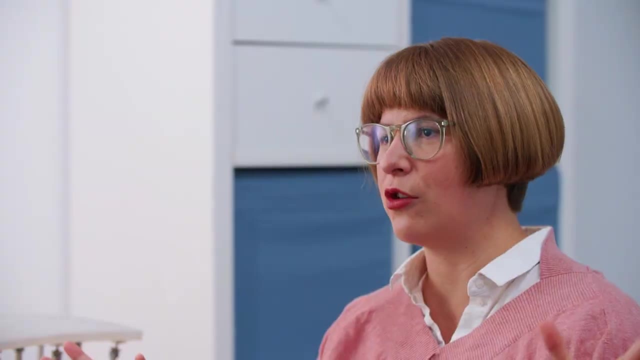 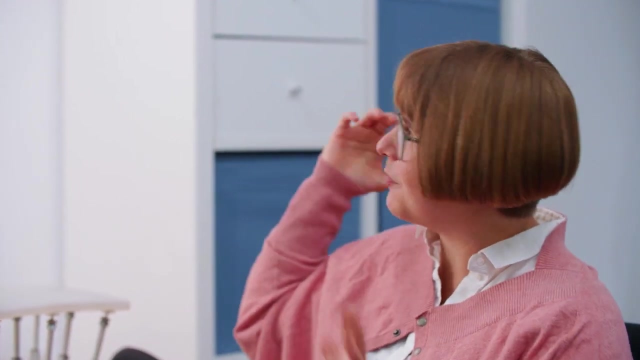 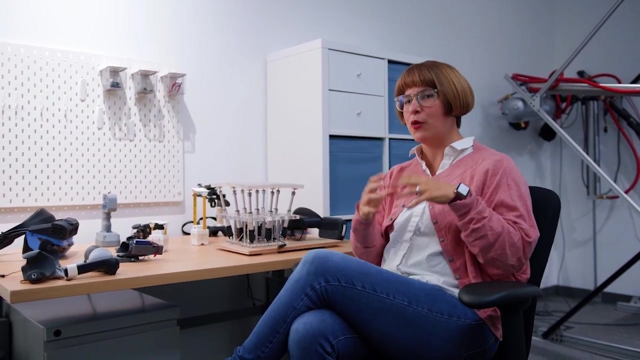 behind it. you will not be able to replicate right. So many days were inside. but we also go outside, right? we want to see how these technologies go on the wild and we study beyond, touch all sort of perception. behind me you see a bit of a vestibulator which will, you know, we just as on a vestibular system, but we 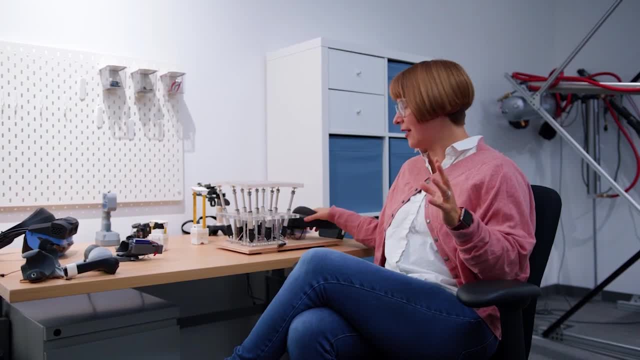 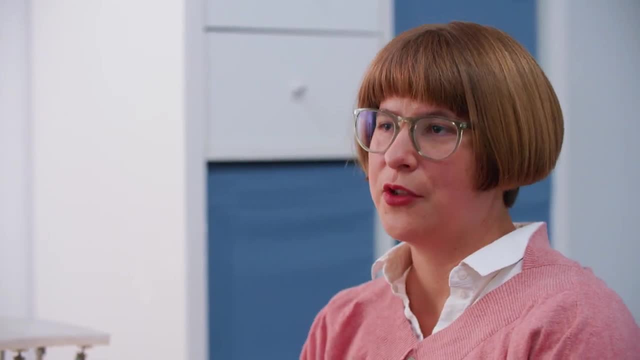 just as on a vestibular system, but we- just as on a vestibular system, but we- We also study a lot of sound, because once you are inside the content, sound is spatial, like in real life, which is also a very big change in paradigm compared to using screens. 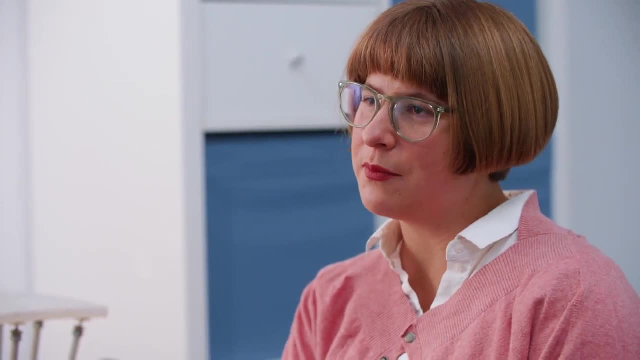 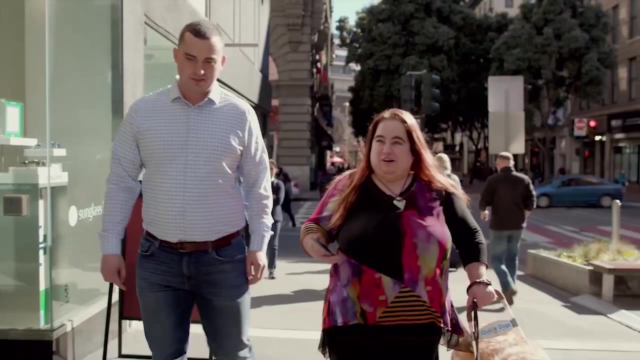 And so in that area, I'm working a lot with the team of Soundscape, Microsoft Soundscape. They are enabling blind and low vision people to go around the world and travel with a different form of GPS which is based on beacons. 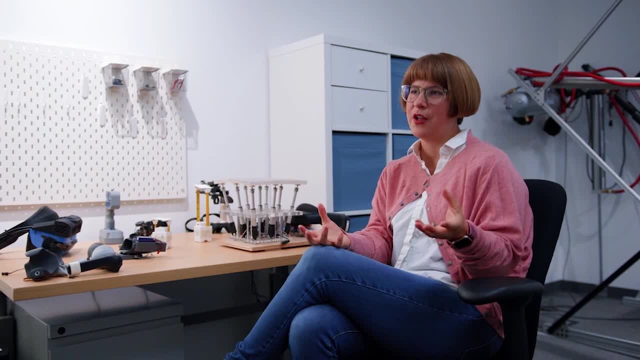 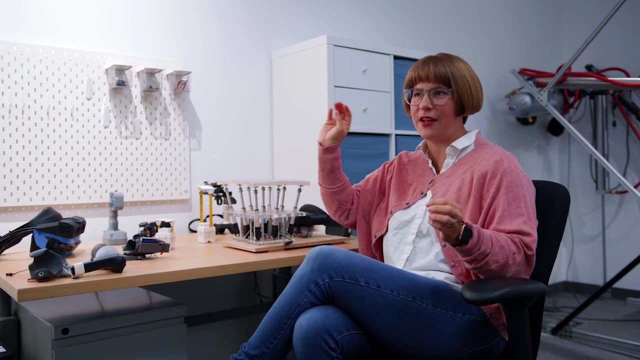 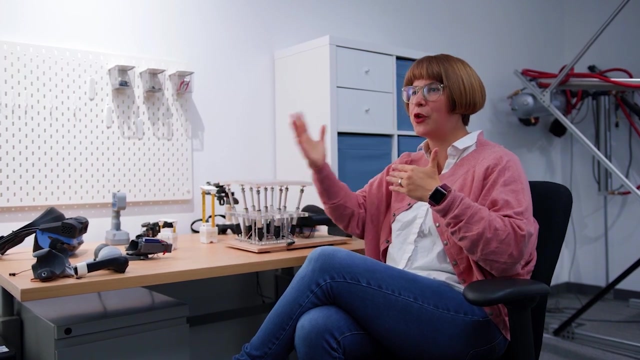 It's a different form of navigation. If you think of the human, you know we were living in forests. we would hear sounds travel towards a source of water. we would hear and you know that would create a mental map as we were going there so we could return to the origin. 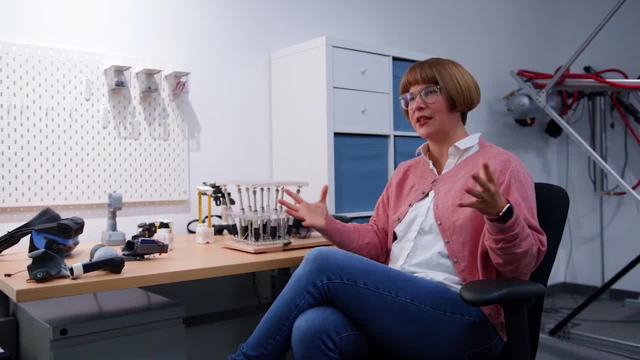 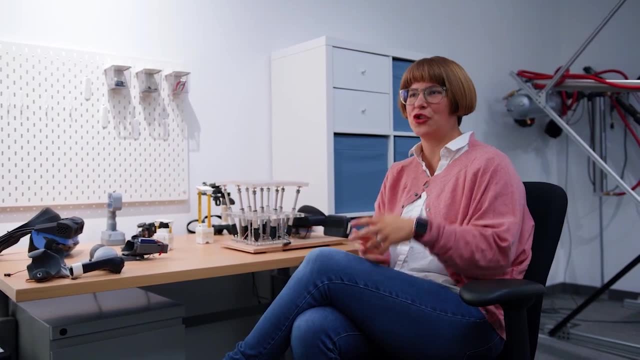 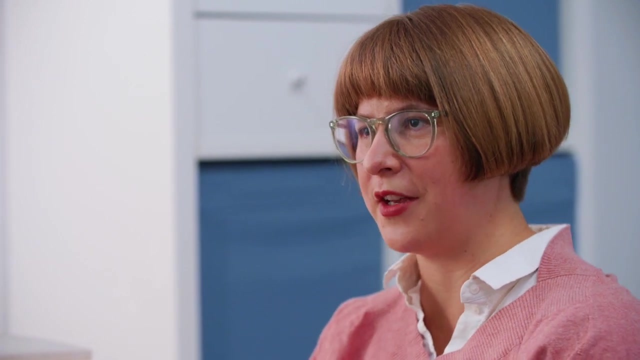 And more recently, you know, this idea of sound emitting systems has been used in modern society. right Churches, minarets and mosques produce sound for people to know and locate where they are. So we're trying to do that, but with digital content all around us. 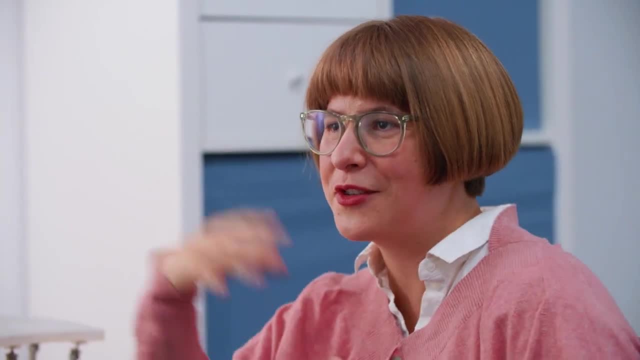 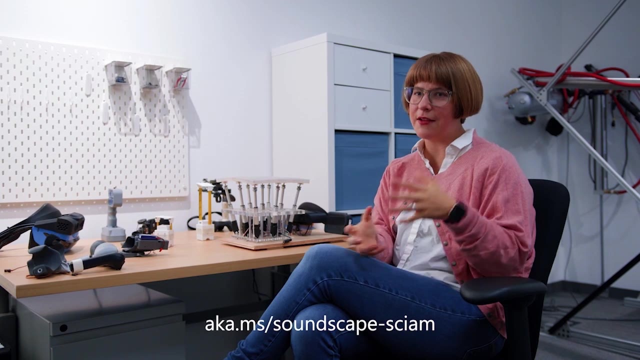 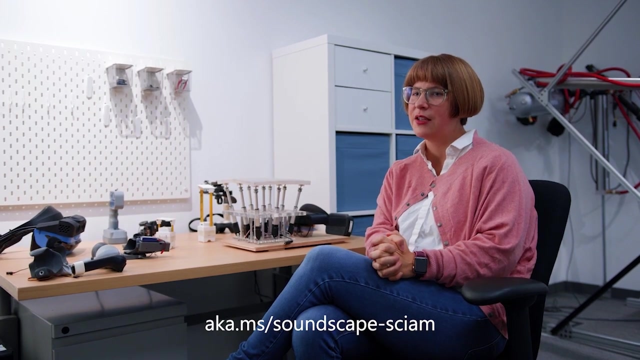 It would be great if the pharmacy made noise so I could go there and find where the pharmacy is. So we're trying to create that type of experience. In particular, I recommend reading this piece we put out in Scientific American just a couple of weeks ago. 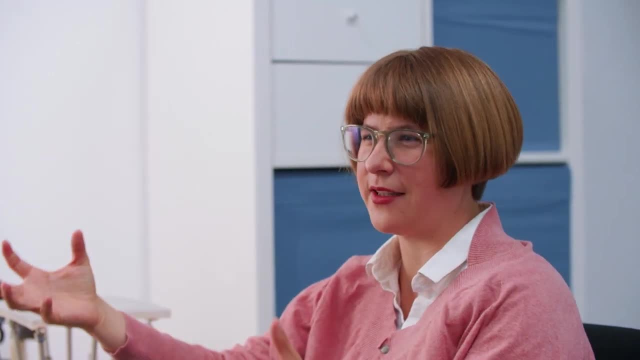 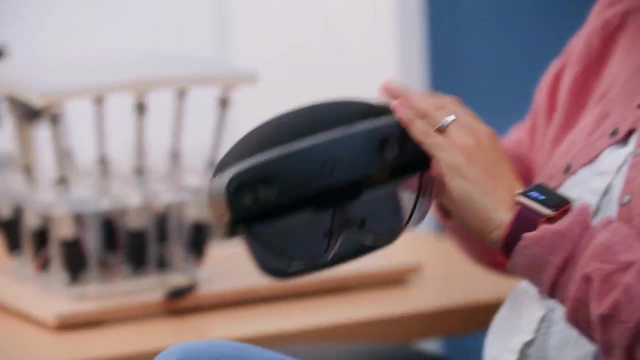 So there are many of these subjects. we're thinking like apples that are static, right, But the truth is, once you put this on, you might be talking to an avatar, for example. So we work a lot on avatars and we are trying to figure out how people behave with a virtual 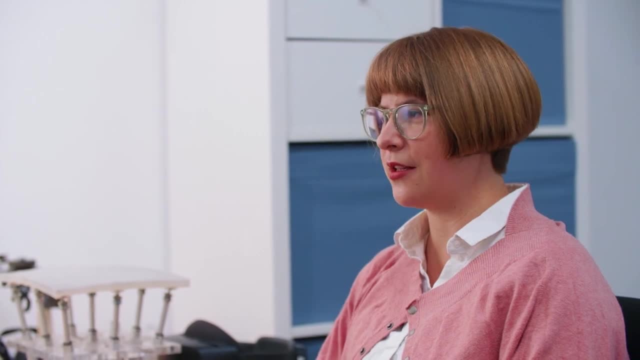 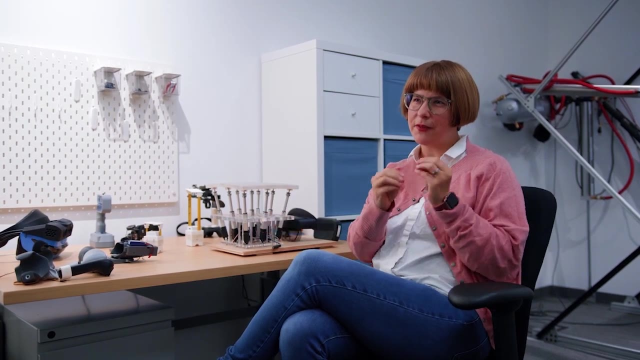 avatar And there are so many possible applications that it's even beyond what we can do For the particular case. you know all these applications of avatars, but for the particular case of AI, I think we have a duty there, right. 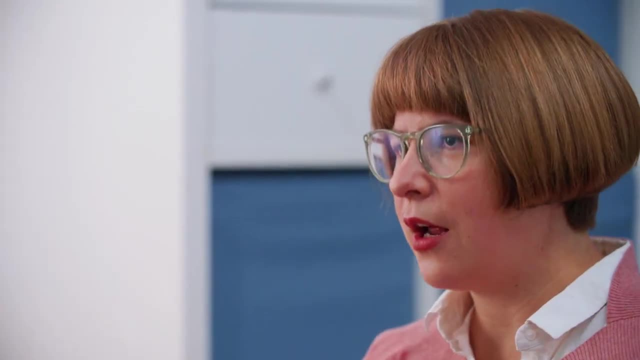 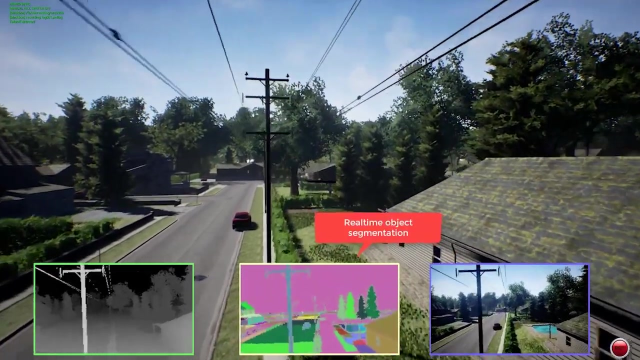 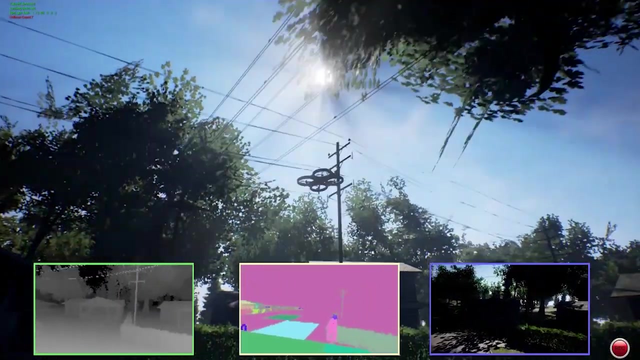 We're creating synthetic data. currently, People are creating training self-driving cars in environments that have no avatars, So you basically have no representation of humans there. In many cases, we're just training. you know, can you stop at this sign? 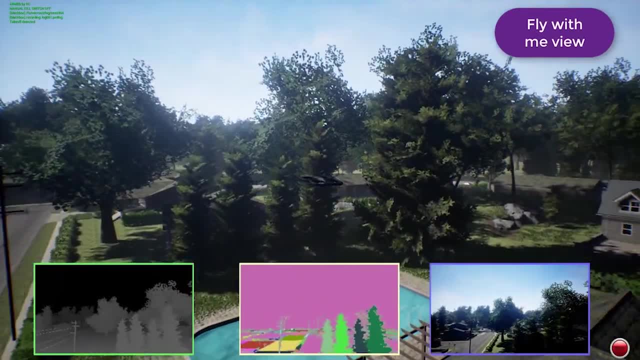 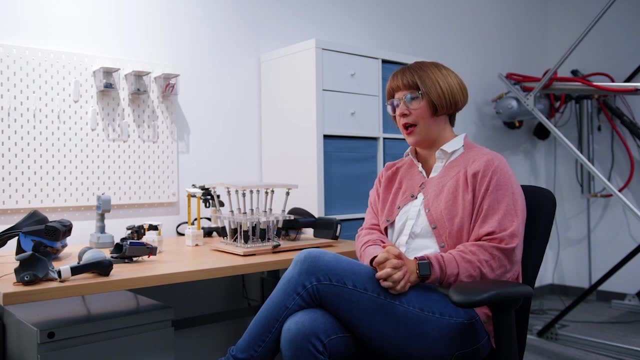 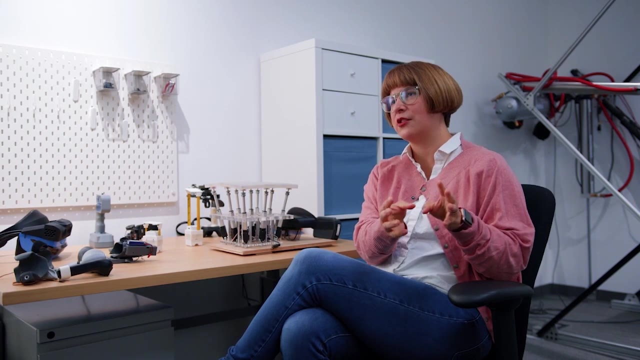 And we need to have the random behavior of humans also inside there to really have a good digital substitute of real life scenarios. And it's even more interesting because once you have humans in there you can trigger actions that would happen very rarely in real life. 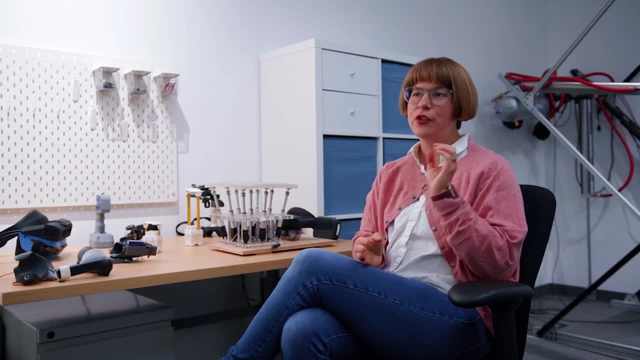 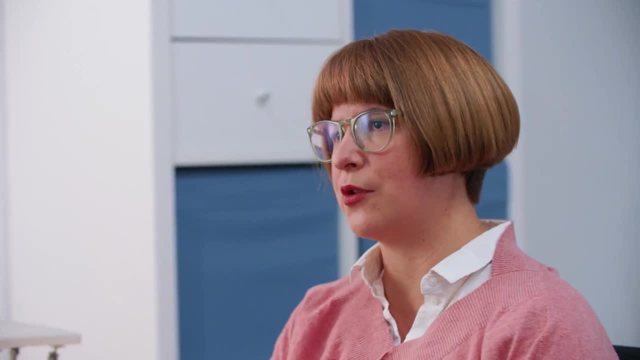 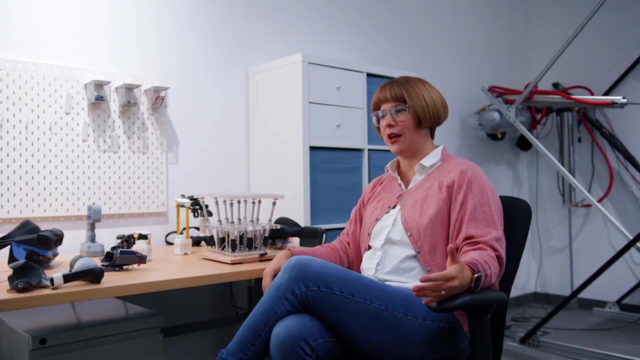 So you can cover many more scenarios than if you were to record real footage. So synthetic training: I think it's something that is of particular interest for AI and the merge of these avatars. So we have been very strong at releasing libraries for everyone to use, like the Microsoft Rocketbox. 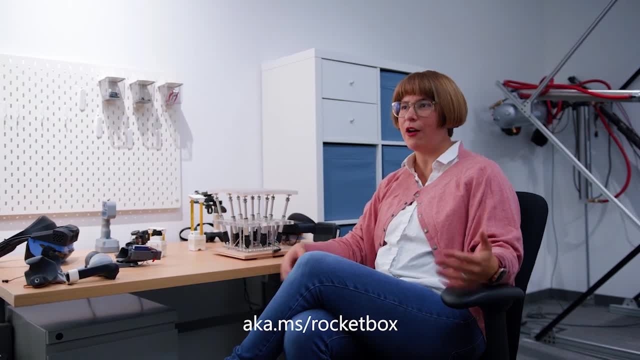 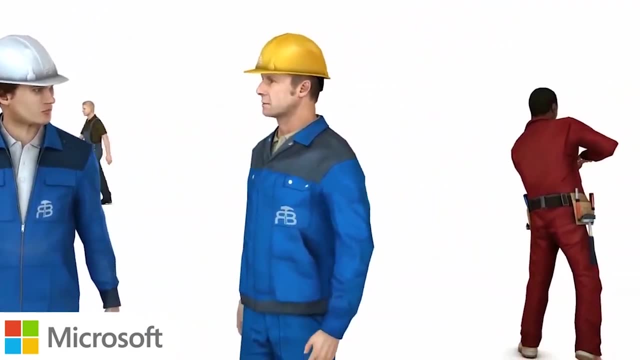 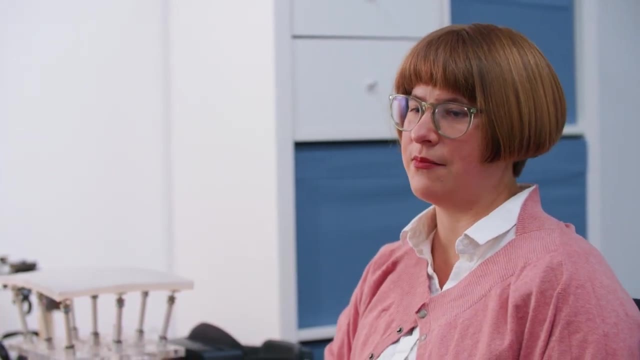 avatar library. So people around the world are also exploring these ideas of how you interact with this digital content and avatars in this case, And we have people in the NIH studying psychological responses in Stanford, UCL, you know you have universities around the world are using our avatars. 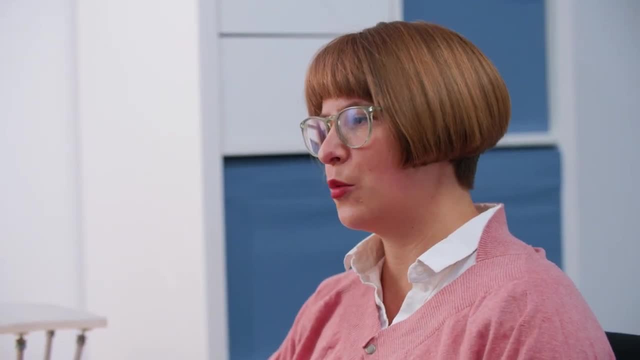 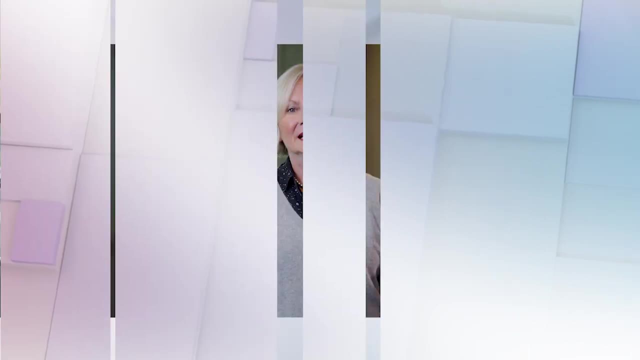 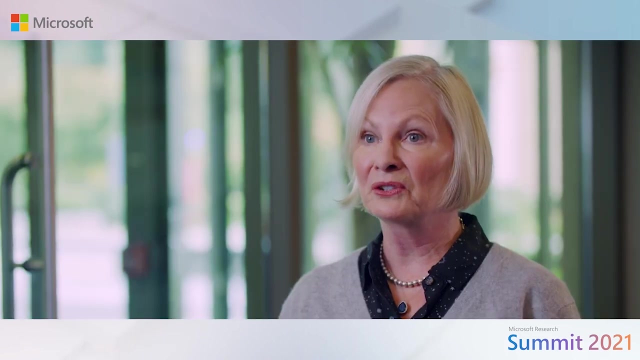 So there are, you know, all sorts of applications and we're trying to see where it goes, also by providing means for everyone to do research in this area. Let's move on to hear from Teddy Sayed. Teddy's a senior researcher in the RISE group at Microsoft Research and also leads the Future. 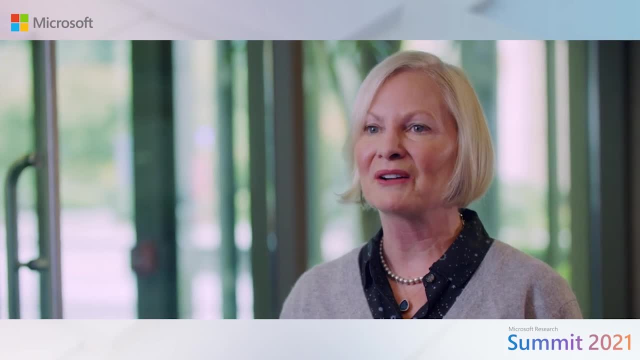 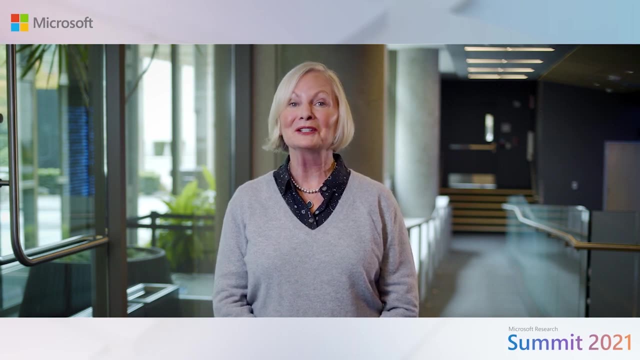 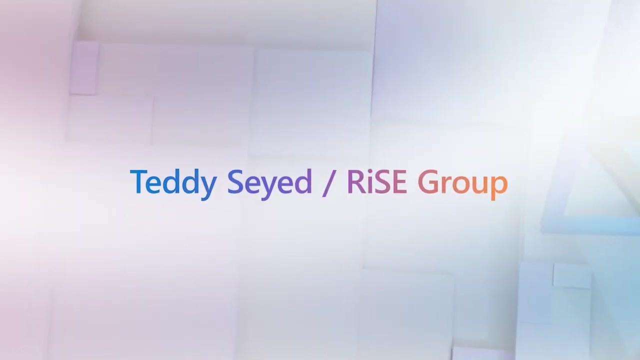 of Wearables team. He looks into the question of how technology allows us to express our identity. We'll join Teddy now to hear more about how smart fabrics and wearables can be used in the future. My name is Teddy Sayed and I'm a senior researcher at Microsoft Research. I'm in the RISE group. 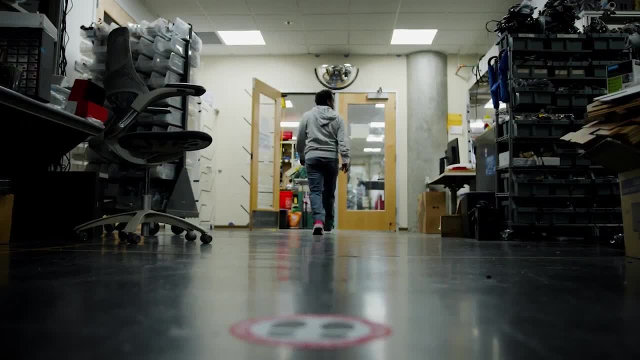 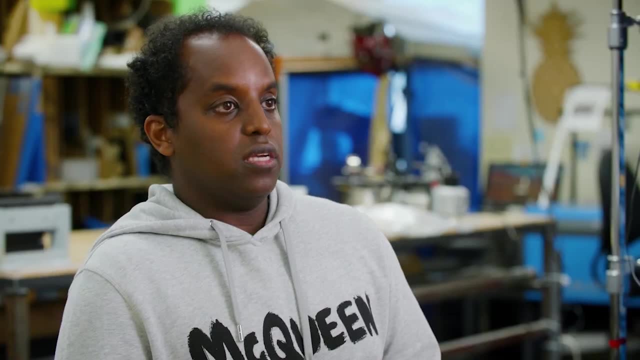 and I lead the Future of Wearables team, And so what I work on is really about connected textiles, intelligent textiles, wearables and really anything in between that involves textiles in general. So, speaking of textiles, you can think of textiles as you know, stuff that's around. 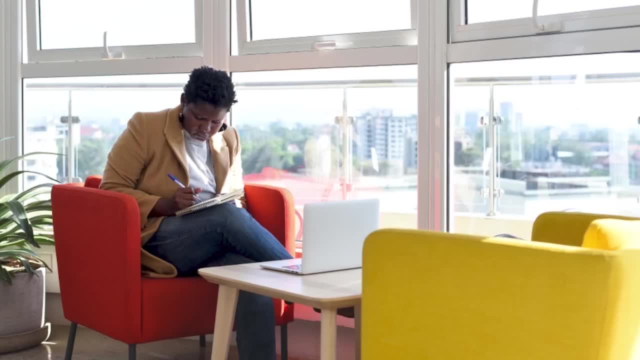 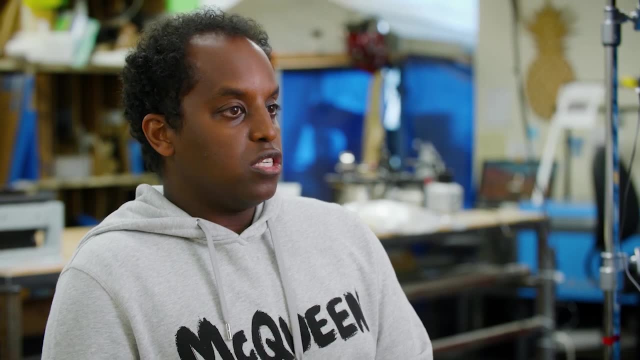 you every day. It's in your clothing, It's on the couch you sit on, It's in your gym bag. Really, it's woven into the fabric of everything and everything we do every day. So you can imagine being at home or working from home: you're sitting on a couch, you're 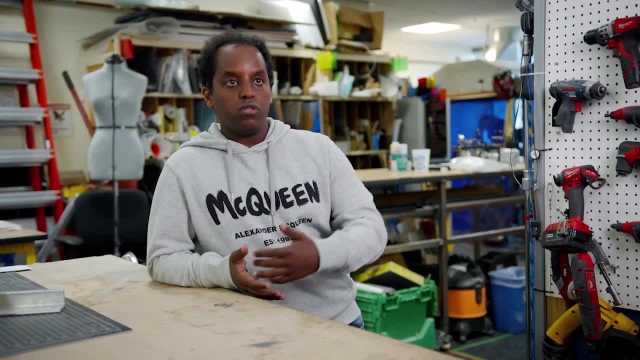 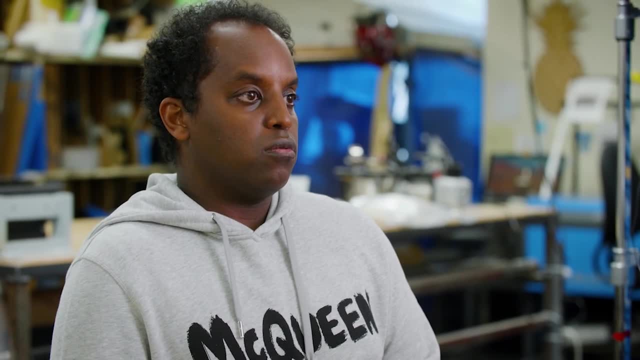 using your laptop, you know you're wearing clothing. there's, you know, the couch. All those things have fabric embedded in them and they're all really woven around what we do today. And then, when we think of, you know the textile experiences, there's also the social experiences. 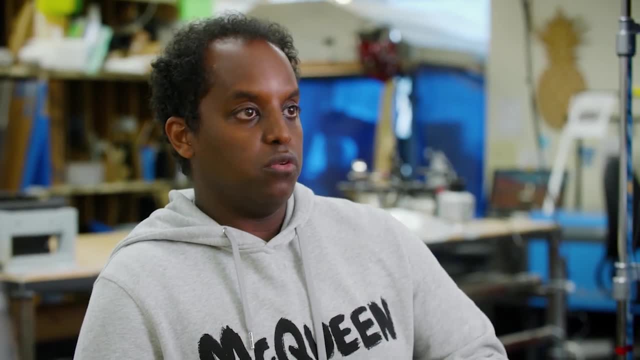 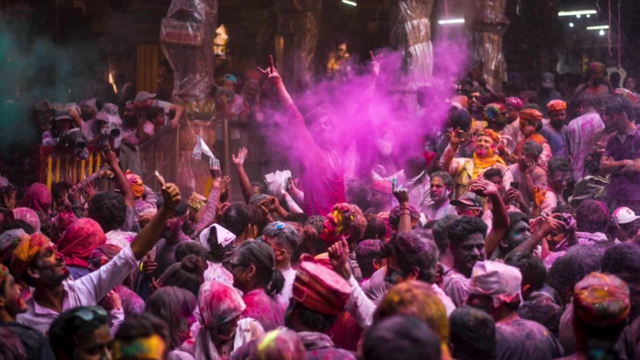 right, There's the aspect of creativity and expression in the clothing that we wear, the activities that we go to. You can imagine being at a large concert Or some really interesting event out in public. But the whole point of this is a lot of it. you know, clothing and textiles is a part. 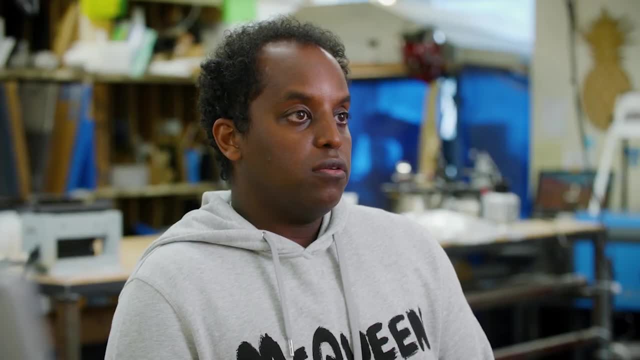 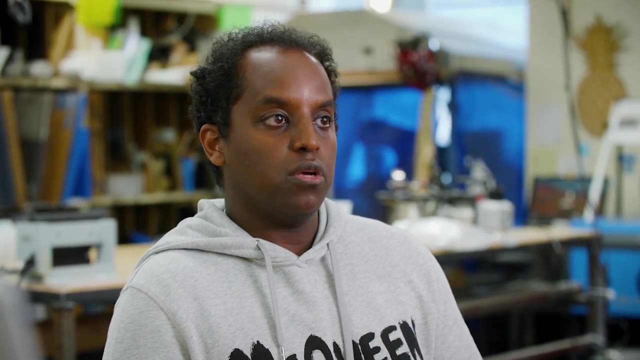 of what we do and it's really woven into what we do every day. So when I talk about smart textiles and intelligent textiles and the connected experiences, what I'm really meaning here is: imagine there's some sort of intelligence, some type of sensing. 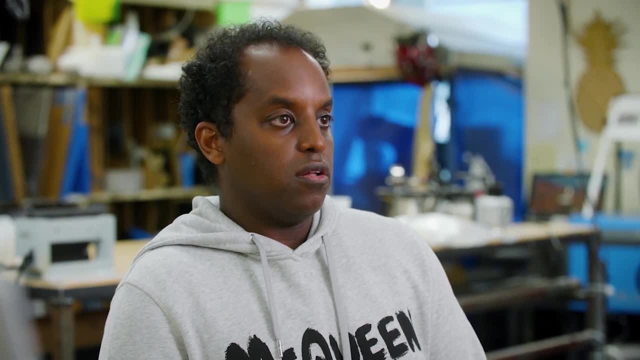 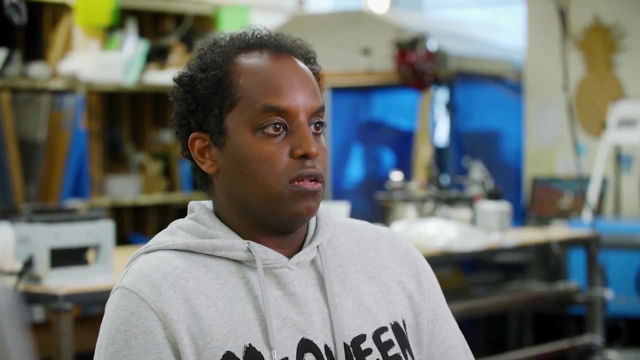 some type of interesting interaction enabled by a textile. So when I think of this entire space of textiles that I've mentioned, you know, I like to think of it as an ocean, right, And there's this whole ocean and we're moving across this ocean. 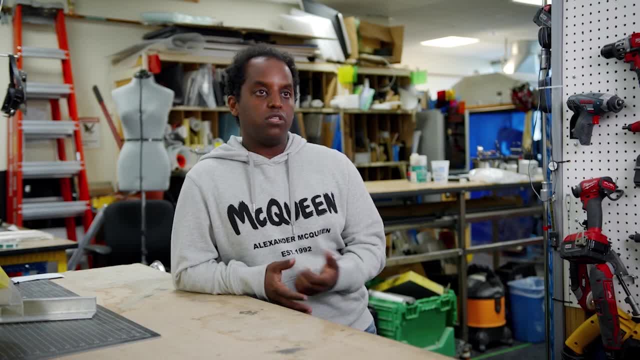 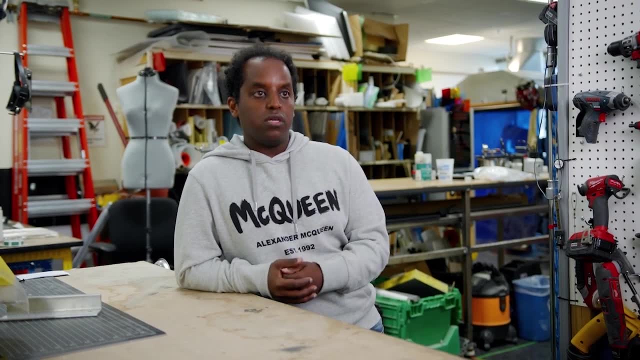 You know, there's many companies: Microsoft, Apple, Google, et cetera, et cetera. We're all trying to move in this ocean, But the problem here is that you know the vehicle in which we're moving on this ocean. 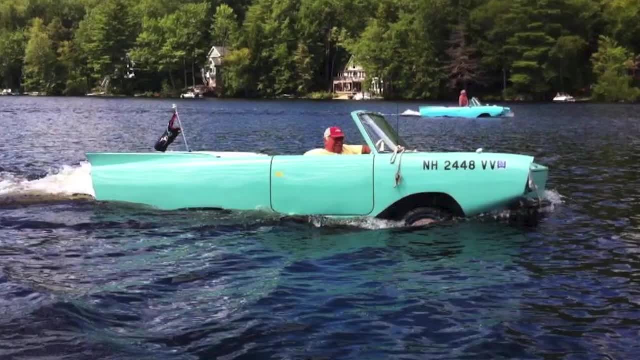 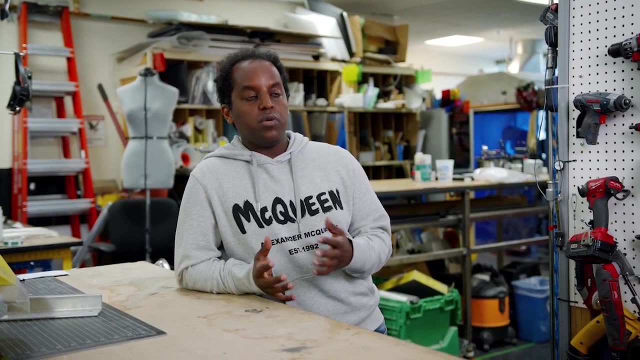 is really a boat, but it's a boat made of car parts. We're using really chunky hardware. We're using, you know, maybe not the most optimized software or hardware experiences. It's really chunky, And so I like to think of this space as moving forward with a boat made of car parts. 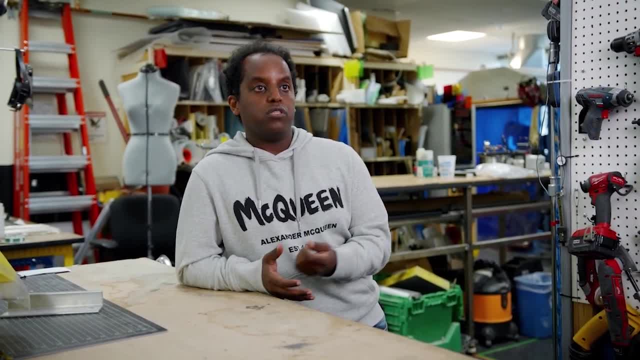 But what we're really looking for is moving this space, And I think that's really important. We want to move this space forward with boat parts, So we need stuff to be integrated into the fabric. We need gestures to be integrated into the fabric. 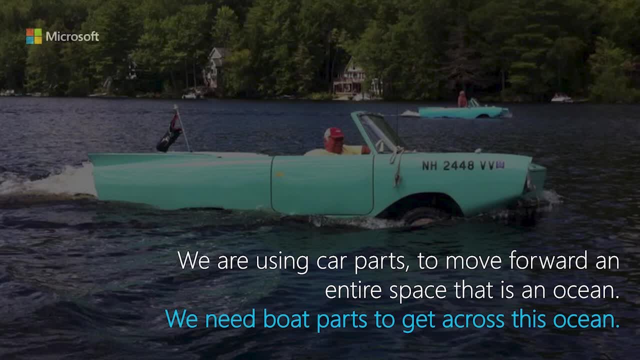 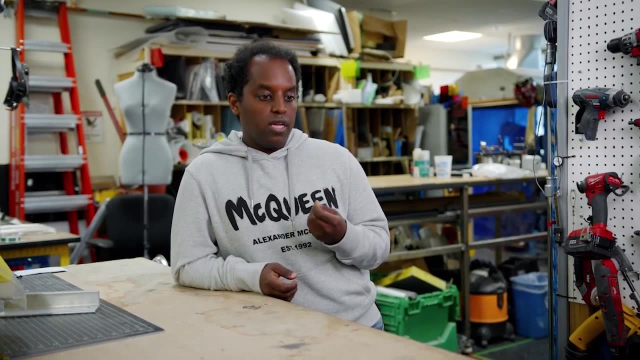 We need technology really to be woven into what we do in everyday life, which I had mentioned earlier, And this really ties back to Mark Weiser's vision of ubiquitous computing, where, you know, computing is woven into the fabric of everyday life. 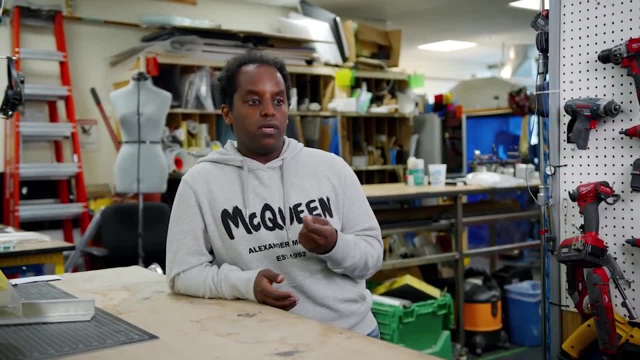 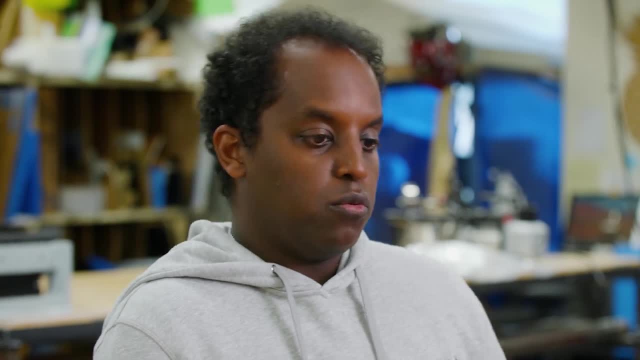 So this is really what I mean about smart textiles experiences. We want to do is make the technology, make that boat better. So how are we going to do that? As I mentioned before, you know we're in this ocean space And we want to do a lot of work that moves it forward. 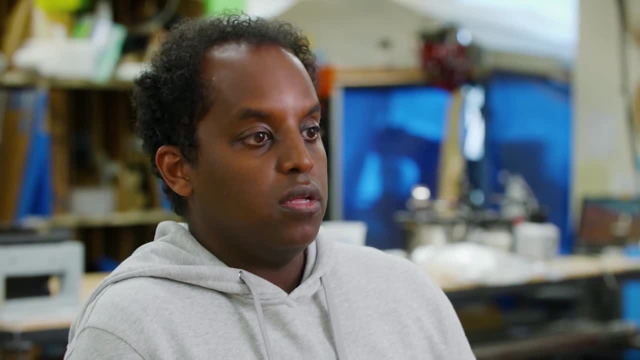 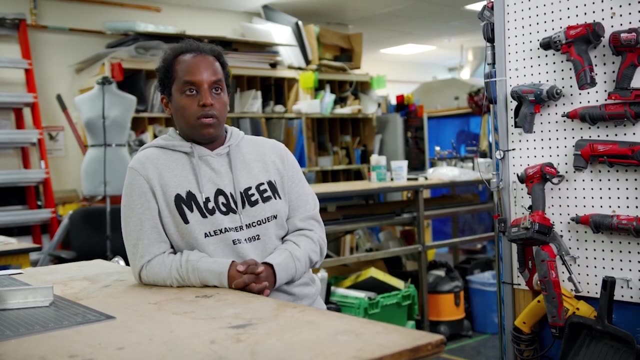 We want technology to be integrated into the fabric. We want it to be part of the textile. So you can imagine how we actually can integrate sensing into fabric, Because you can imagine there's not going to be cameras available all the time. If we're sitting on a couch at home watching a sports game or a movie and our hands are. 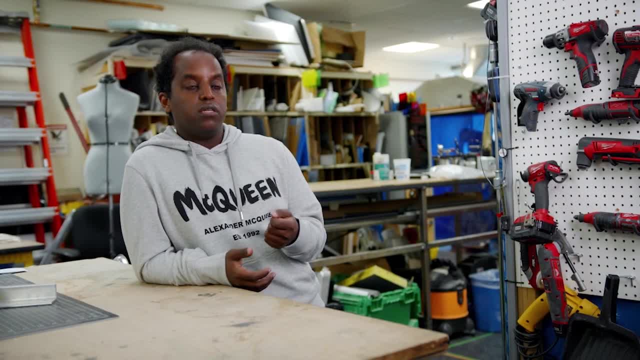 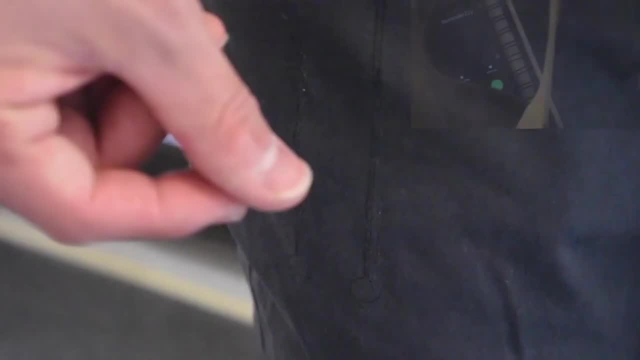 dirty. what are we going to do? Well, here would be a nice use case of actually having textile sensing integrated, And in Forbitria we looked at how do we actually integrate sensing into the fabric, And we came up with a pretty clever way of using machine learning to do that. 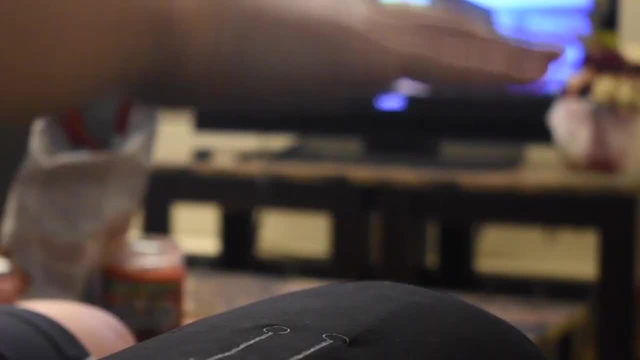 So that's what we're going to do, Thank you. So we have a lot of different ways to detect different gestures, whether it's tap or click or even wave. So traditional techniques that you see with camera we can actually do directly with fabric. 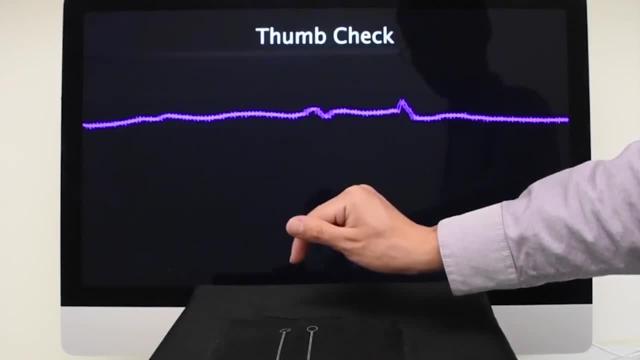 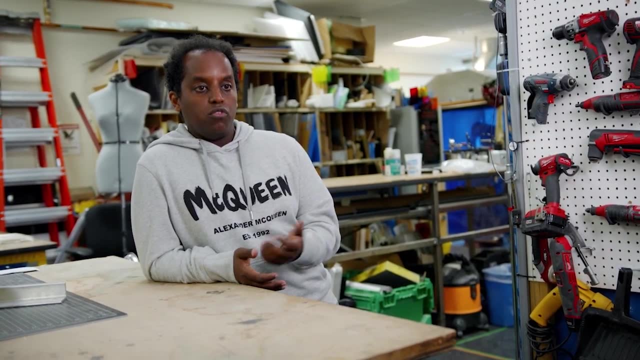 which I think is really, really cool. But moving beyond just sensing, one of the other challenges that we have with textiles is that textiles deform And there's a challenge of deformation, And so what I mean by deformation is: imagine you have a sensor directly on your shirt. 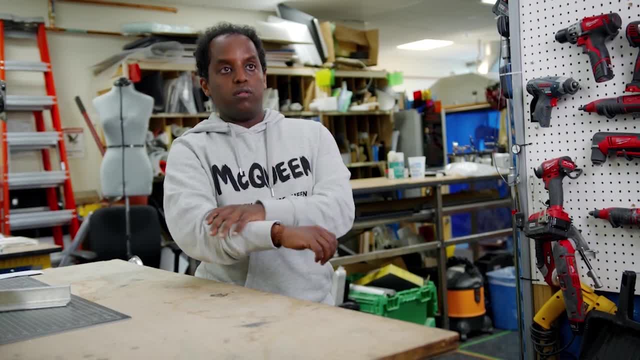 And if I scrunch it up, the sensor is probably not going to work. So how do we solve that? This is what I mean by deformation. So in this next project you're going to see here, we're actually trying to solve. 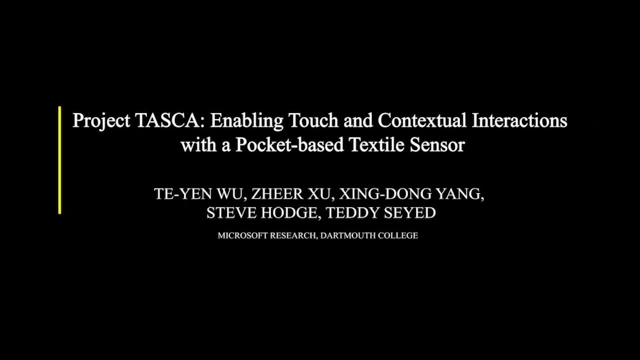 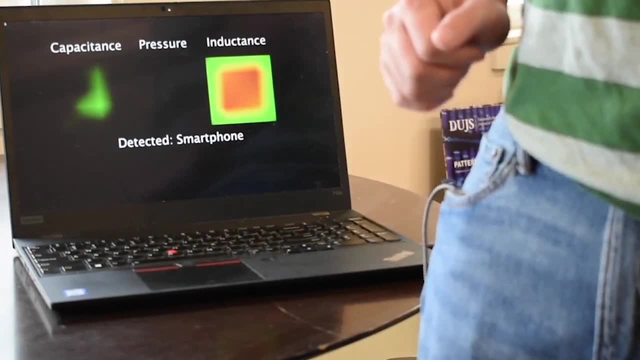 for deformation, And so the first place we solved this for was the pocket, Because the pocket is one place where you can put objects in. it deforms quite heavily, And if you can solve for a pocket, you can most likely solve for the shirt in your gym. 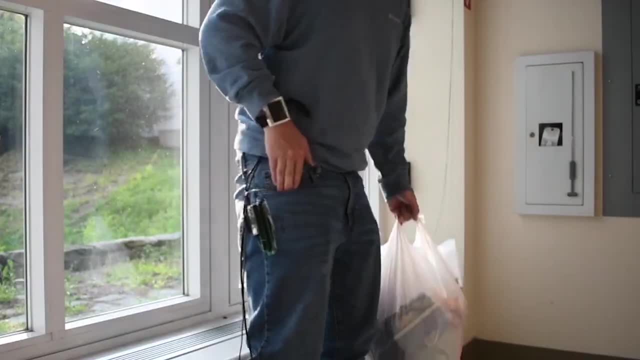 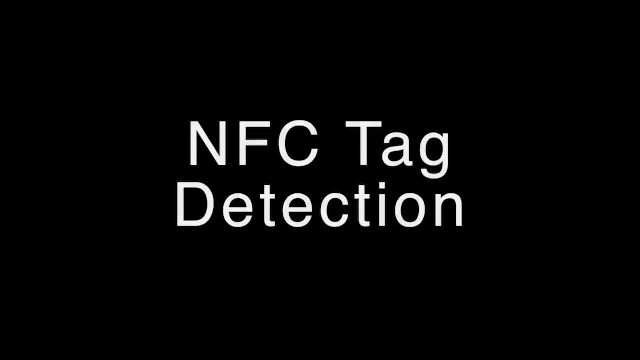 bag that you take out and you put on. So here we're actually using some pretty clever- again clever- techniques with machine learning to detect different objects that go into your pocket, And not just objects but also gestures as well, which is again going back. 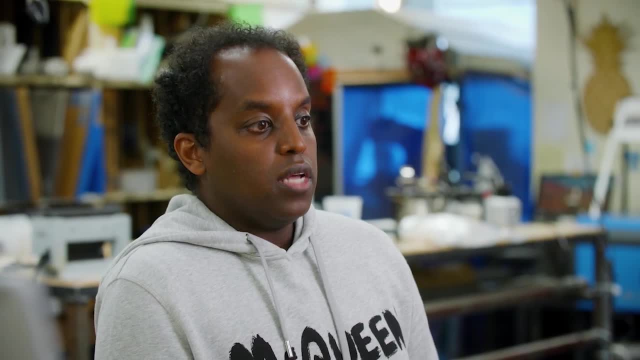 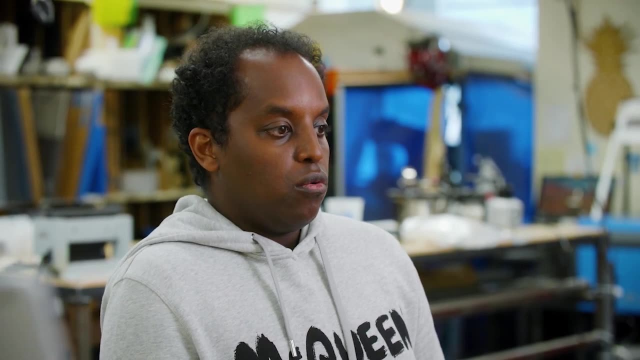 to the areas of focus for HCI. And, last but not least, I haven't really touched upon in the previous two projects- the human side. If you think of this whole space as an ecosystem, right now this ocean is really being pulled by technology companies, which is something I am not really passionate about. 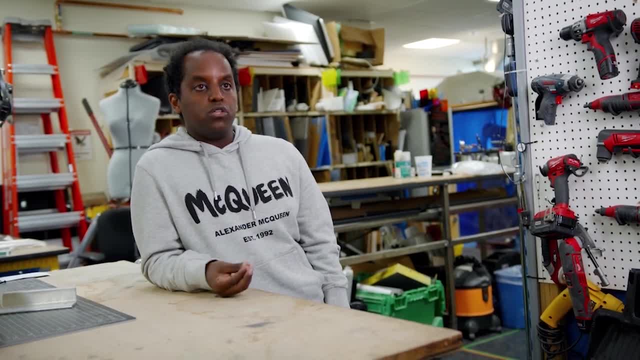 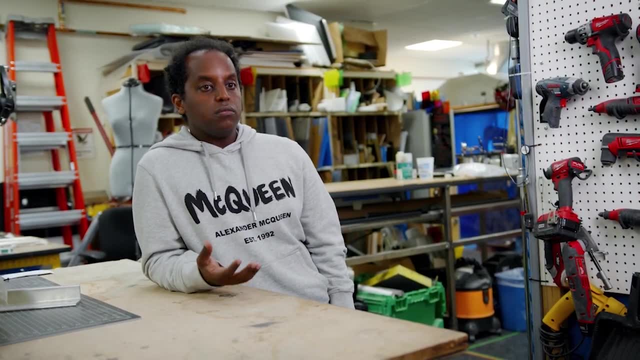 I am passionate about wearables and we are as well at Microsoft. But this space should be really led by designers, by apparel brands, by the people that actually understand and have history with apparels and textiles. So the idea here with Project Brookdale is: can we empower that community? 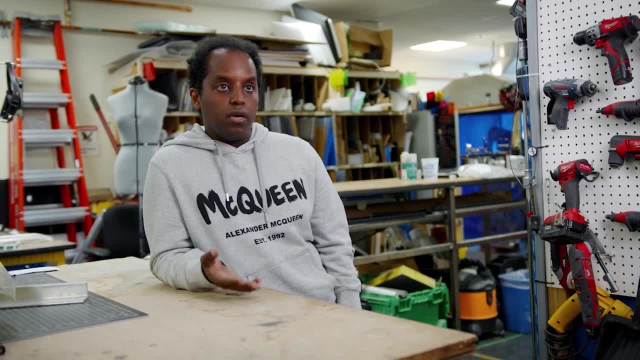 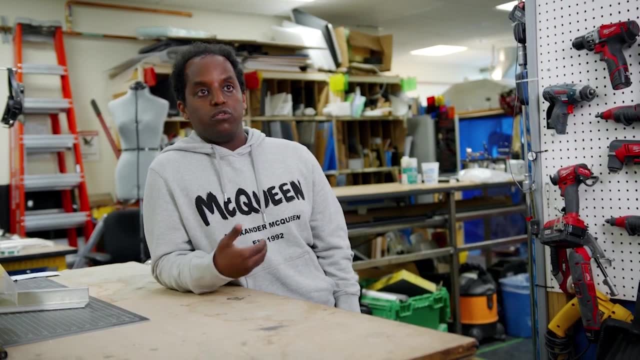 to have that experience. Can we create textiles? Can we create APIs, Can we create hardware, software experiences that enable them to then design the experiences that we want in the future? For myself, I don't want to be creating the next wearable textile or the next wearable. 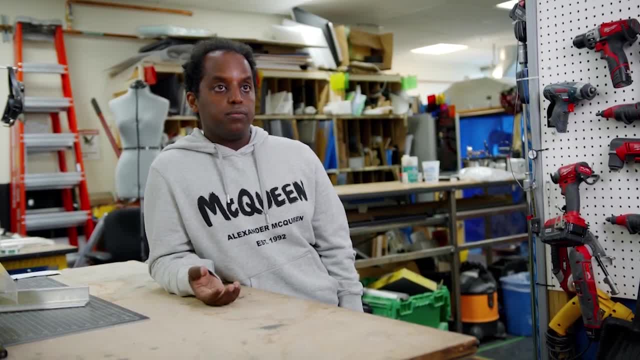 but I want them to be empowered by the work that we do at Microsoft, which is our goal here And in Project Brookdale. we ended up going to New York, And the reason why we went to New York is obviously New York is a global fashion hub. 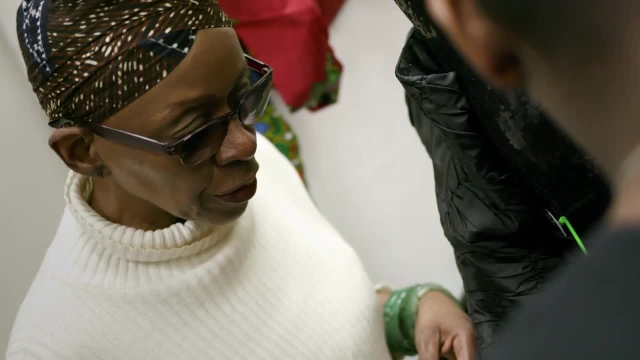 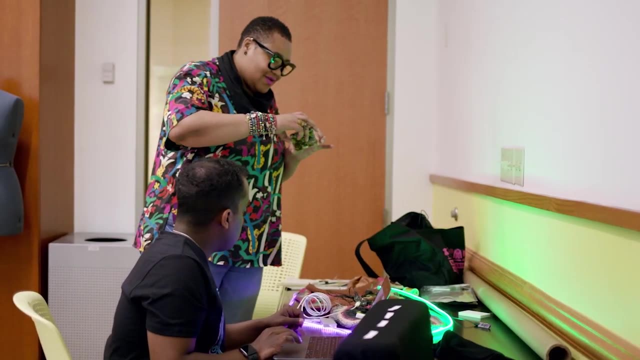 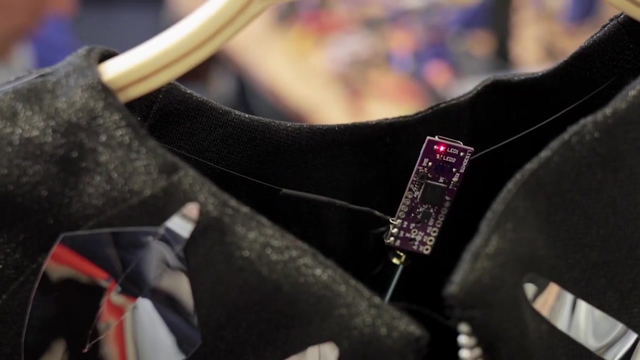 and a lot of interesting creative designers live there and work there, And so by going there, we want to actually explore what is it like to empower a set of designers with tools, hardware, software- To create interesting wearable experiences, And by this I mean using tattoo sensors, using motion sensors, using lights, all the things. 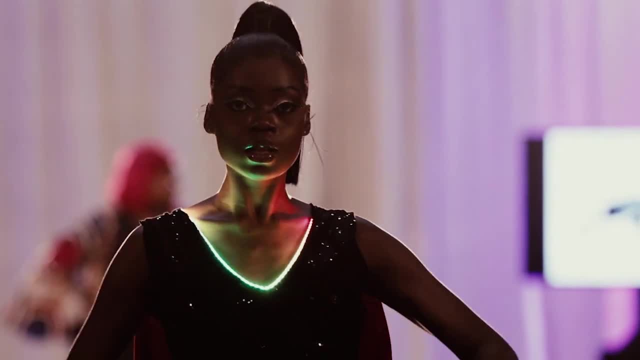 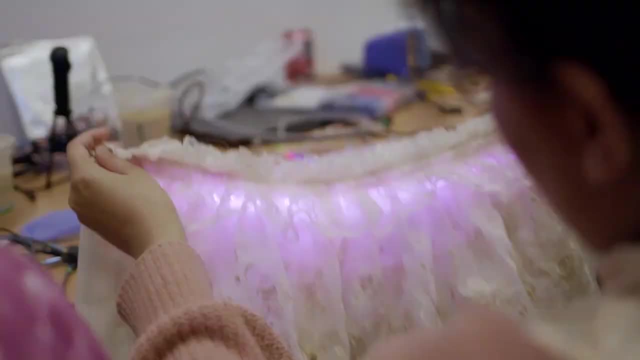 that kind of exist today in the space of wearables, Can we design tools for them to empower them? The idea here being, if we want this space to be led by that industry, we need to work with them side by side. HCI: we really focus on the human side as well as the computer side. 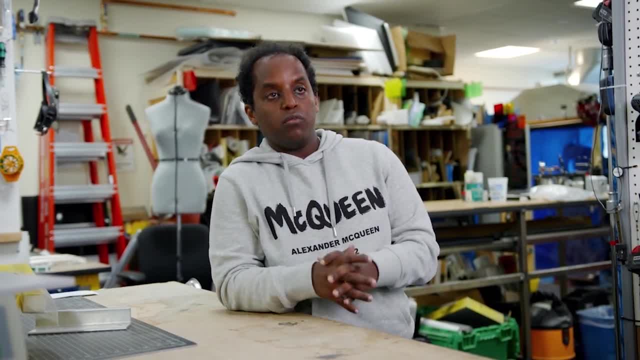 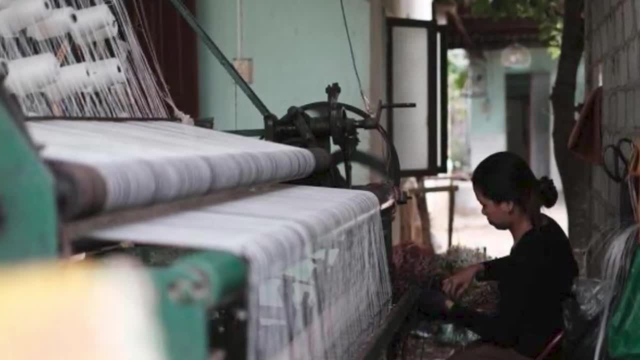 But when you think of the space of textiles and really the broad space in general, it's really about the people that are working in it and the impact that it has on the environment. In the case of textiles, there's a huge environmental impact on the type of textiles we use. 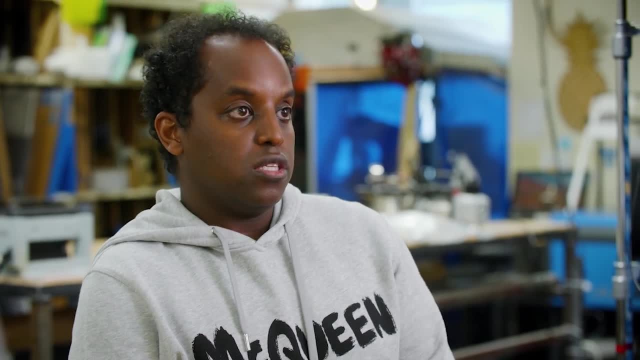 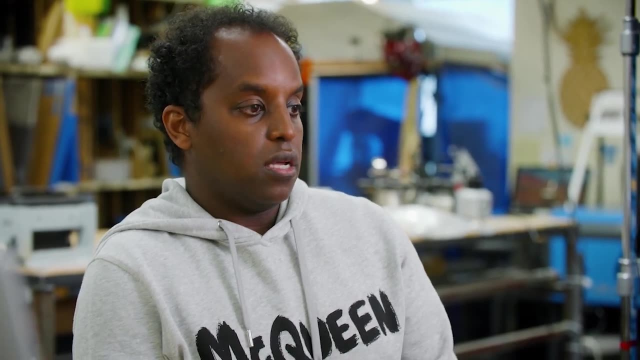 the waste, how it's manufactured. Now you're adding an element of intelligence. right Now there's hardware, there's software involved that does all the computation. So really there's a whole ecosystem that's evolved in this space. And because we're at such a point now where everything is really new, 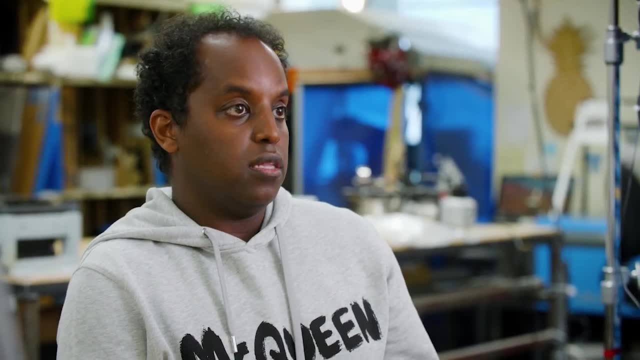 we can actually define and design for sustainability in mind in the space of intelligent textiles. So, whether it's the case of the factory worker who's trying to integrate smart textiles at the apparel HCI, we need to think about that. So whether it's the case of the factory worker who's trying to integrate smart textiles at the apparel, 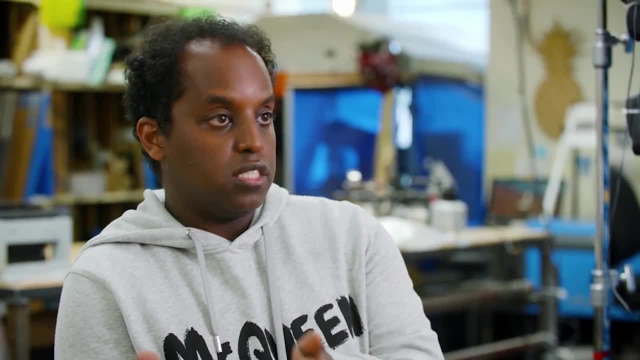 we need to think about that. So, whether it's the case of the factory worker who's trying to integrate smart textiles at the apparel to the brand, that's actually making it to the end customer as well. So we can design for sustainability in mind. 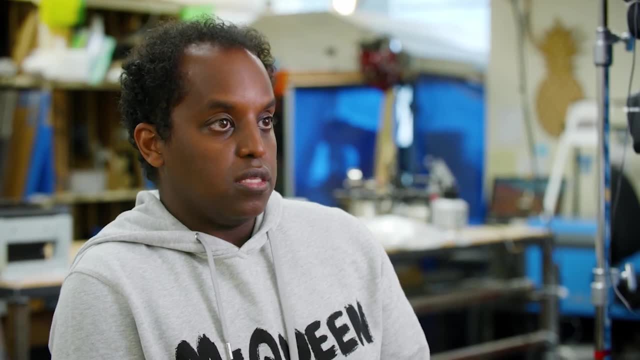 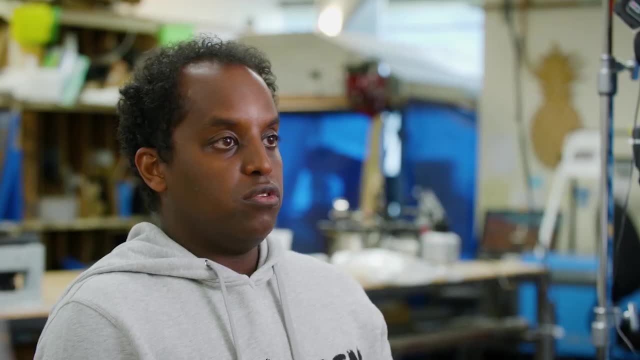 which is one of the really unique aspects about the space that we're working in at Microsoft Research. And so, coming back to that analogy I described earlier with the boat parts and the car parts, what we're trying to do today is really emphasize building out that better boat. 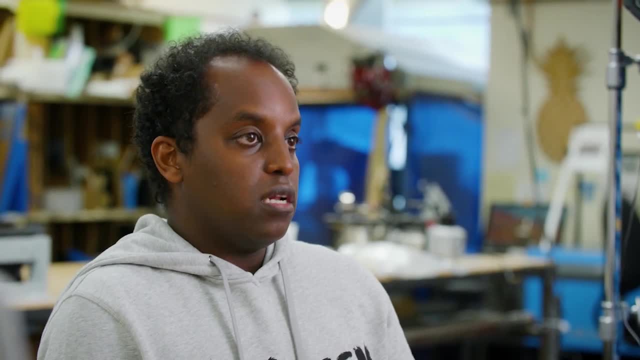 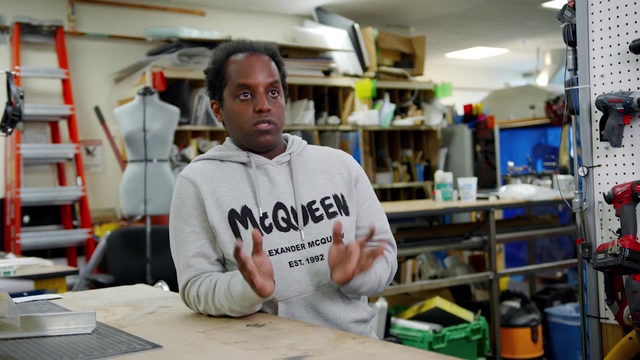 whether it's better sensing through the fabrics- sustainable fabrics that are also intelligent- to designing better back-end systems that take into account the environmental impact. it's really all about the ecosystem in moving forward in this ocean, And that is one of the things I'm really excited about here at Microsoft Research. 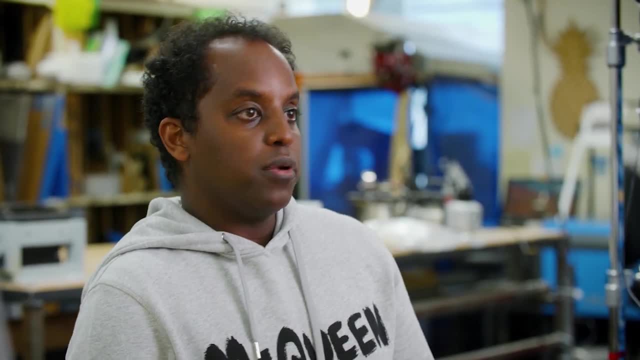 So obviously this insane vision we have here at Microsoft Research is not just myself, but it's a whole team of us at the Future of Wearables Lab. First off, it's led by Evelina Barhudran, who is a co-innovator. 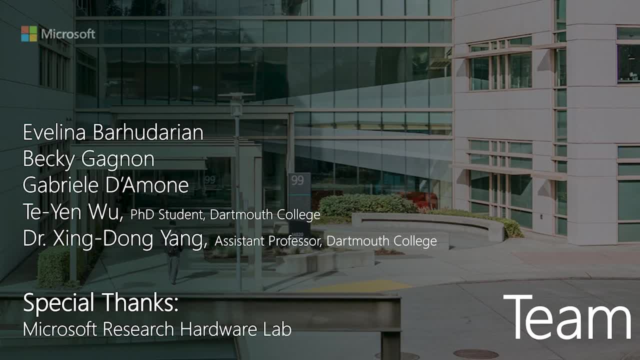 as well as the leader of business development and strategy for myself and the team, as well as Becky Gangnon and Gabriel Dumont, who handle a lot of the engineering, as well as industrial design As well. I have some amazing academic collaborators. 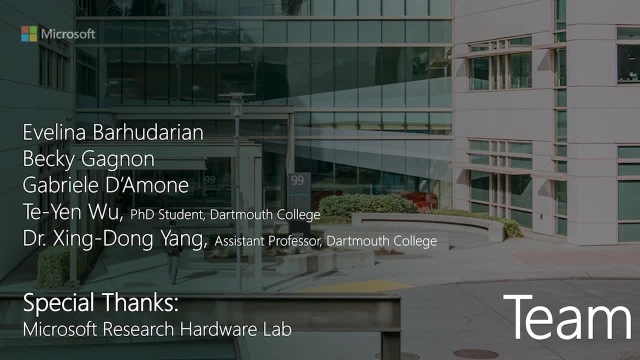 Taeyun Wu, who's a PhD student out of Dartmouth College, as well as a supervisor and a colleague of mine and close friend, Dr Zingdong Yang, also out of Dartmouth College. I also wanted to give a quick shout out to the Microsoft Research Hardware Lab. 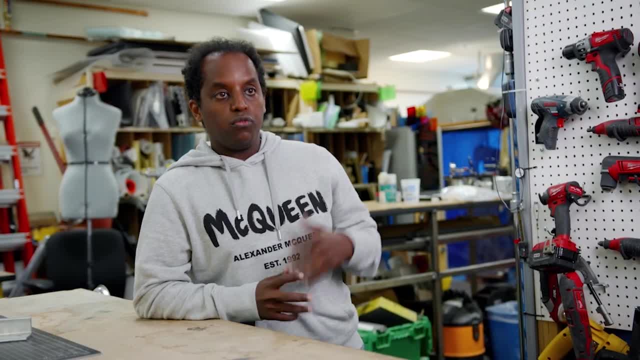 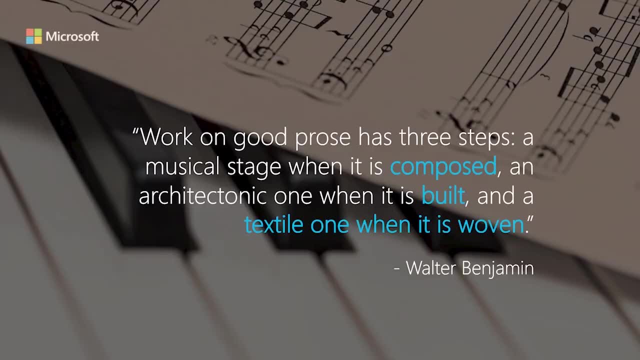 who does amazing, amazing work here, moving this vision forward. So before I leave you today, I kind of want to leave you with a nice quote from Walter Benjamin, who was a personal favorite of mine. Work on good prose has three steps. a musical stage when it is composed. 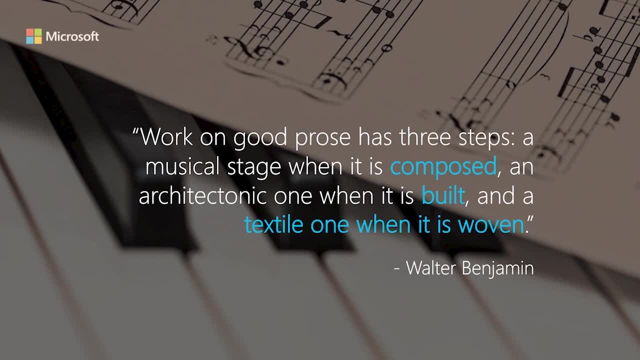 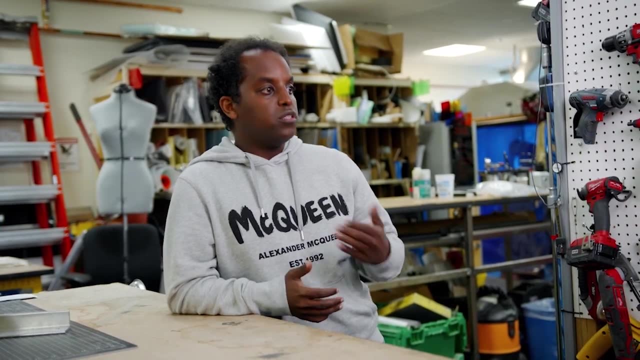 an architronic one when it is built and a textile one when it is woven. So at Microsoft Research we're composing a lot of the components you've seen today. You know we're trying to make that boat better. We're building all the necessary software and infrastructure for it. 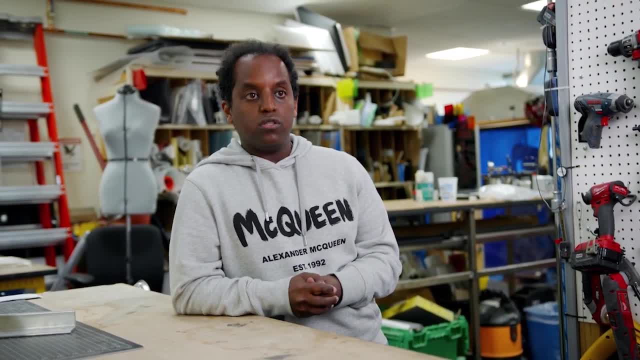 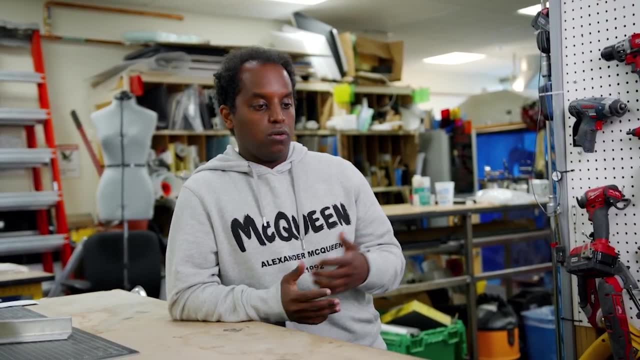 But really what it comes down to- especially you as the audience and looking for collaborators as well- is weaving this all together through textiles. So if you're someone who's interested in smart textiles, connected experiences through you know, jerseys or areas like that, or even really just interested. 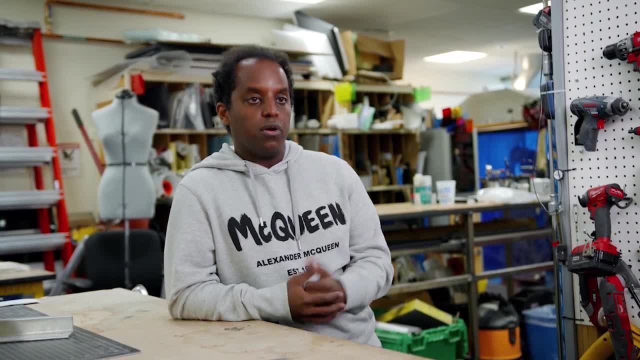 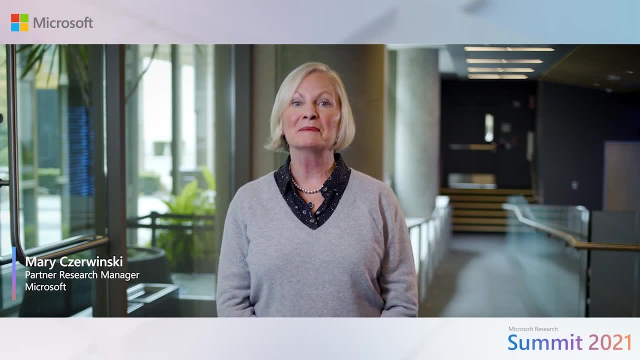 in wearables in general. please get in touch and let's collaborate, because that's really what we're all about at Microsoft Research. Up next, you're going to meet Anne Paradiso. Anne is a principal research designer in the Enable Group here at Microsoft Research. 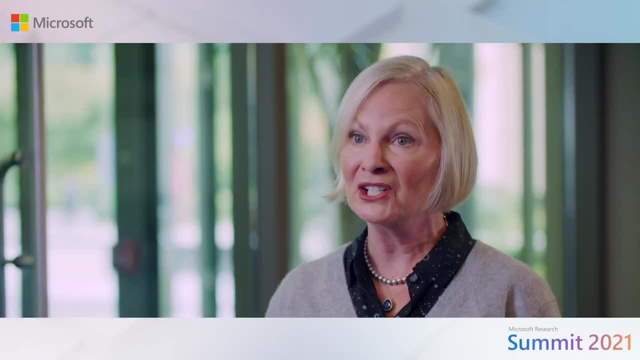 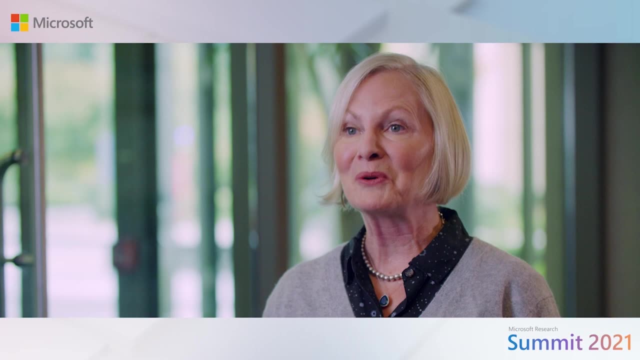 and she works to pair human-centered design and technology to enable expression and creativity. The Enable Group creates technologies that improve the lives of people with disabilities. Community is one important aspect to the group's work, so they design new technology with users, not just for users. 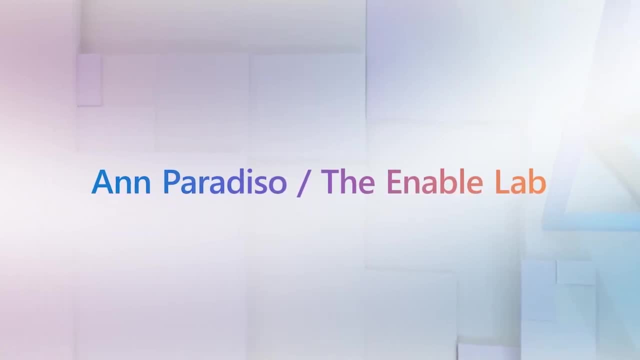 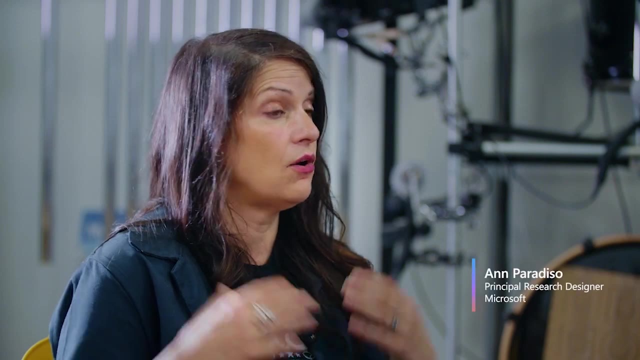 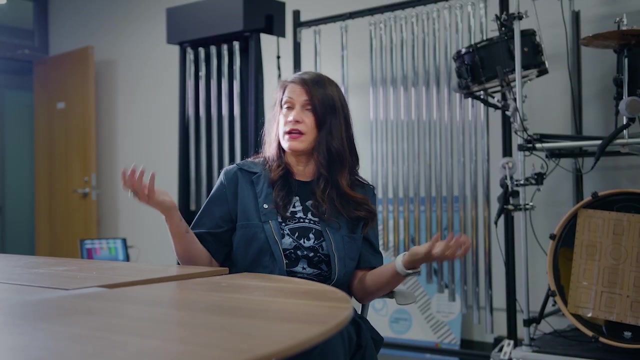 I'm Anne Paradiso and I am a research designer at MSR and I'm sitting here in the Enable Lab in Redmond. One of the things that I care deeply about, and that I know all of my collaborators care deeply about, is that gap between what happens in a research lab or in this lab. 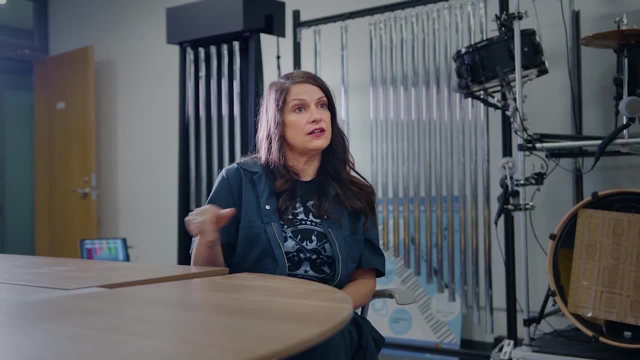 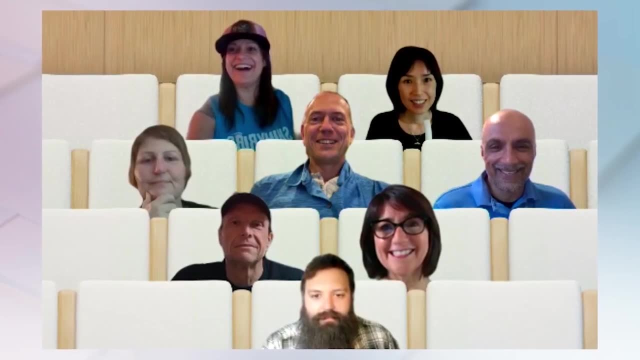 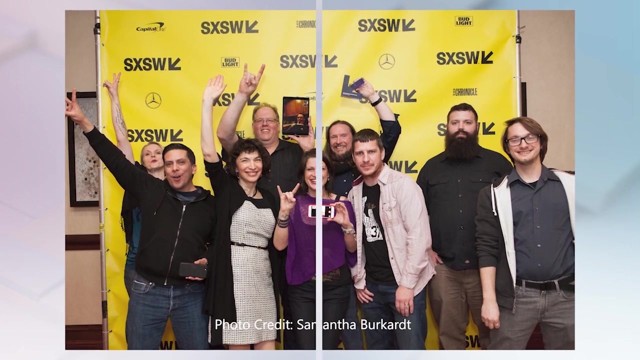 or in a development environment, and getting technologies that are critical into the hands of users who can use them and benefit from them. We have several collaborators inside of Microsoft who have different skill sets that when we combine them together, we find we can be more effective as a team. 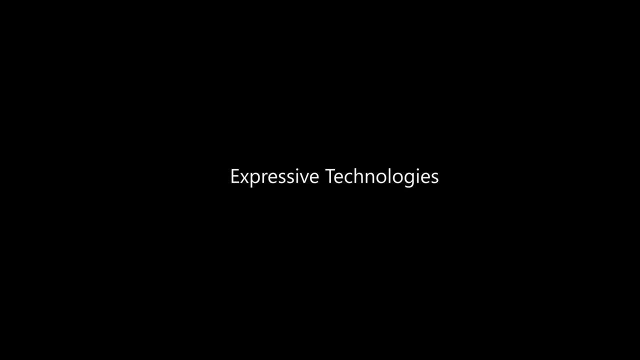 Expressive Pixels is a technology that allows us to be more effective as a team. Expressive Pixels is a technology that allows us to be more effective as a team. It's a technology-mediated creativity toolkit. It's the result of a longstanding collaboration among the Enable Group and central engineering teams. 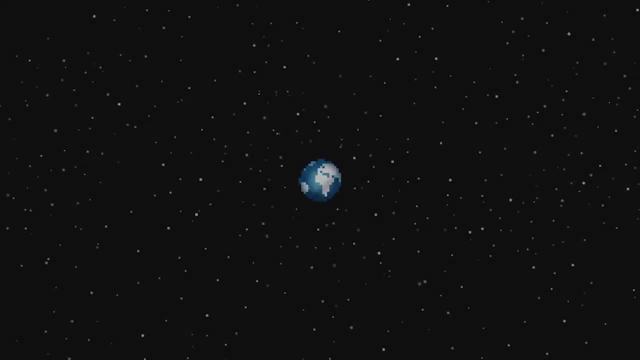 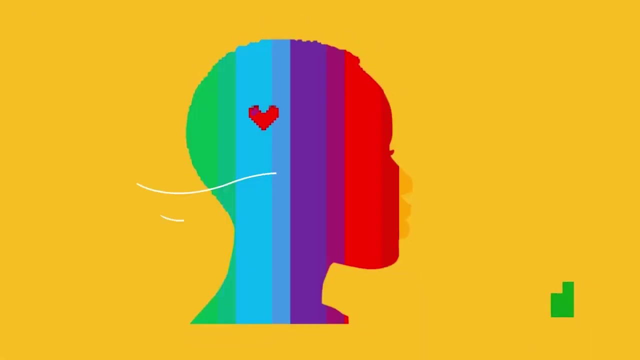 at MSR Redmond and the Microsoft small, medium and corporate business team. The platform embodies our shared belief that expression through technology, art and communication should be an empowering experience for all. Expressive Pixels can be paired with a variety of inclusive inputs and LED displays. 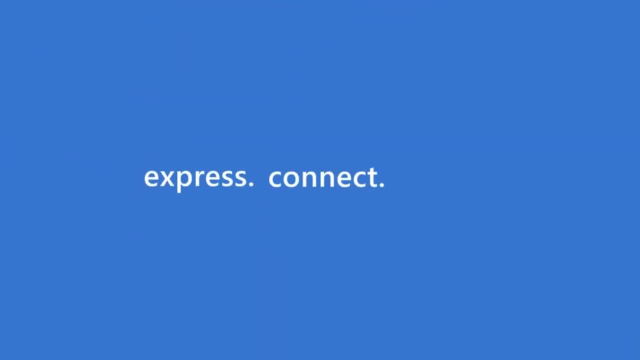 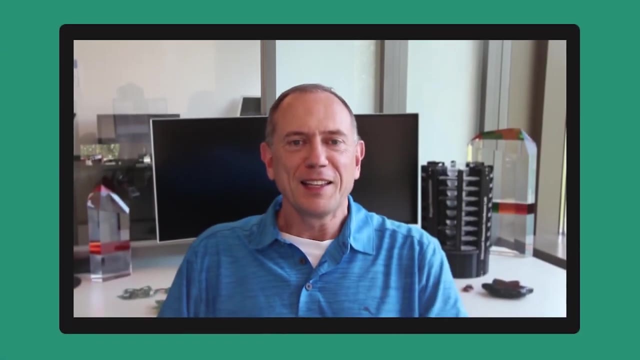 to enable all sorts of novel, alternative avenues for creative expression and communication. Here's a short introduction to the platform by Expressive Pixels co-creator, Gavin Janke. Hi, I'm Gavin, and I'm excited to share with you Microsoft Expressive Pixels. 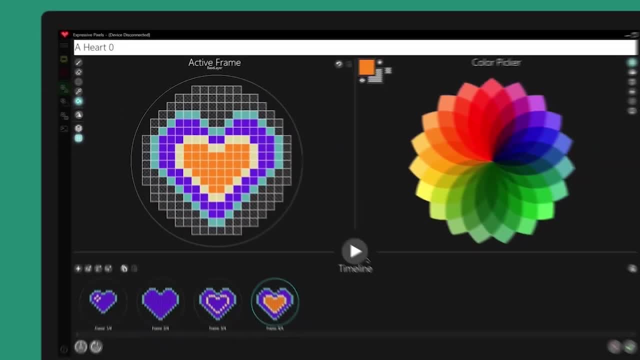 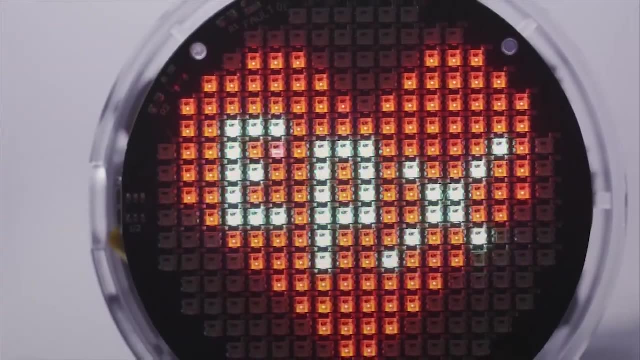 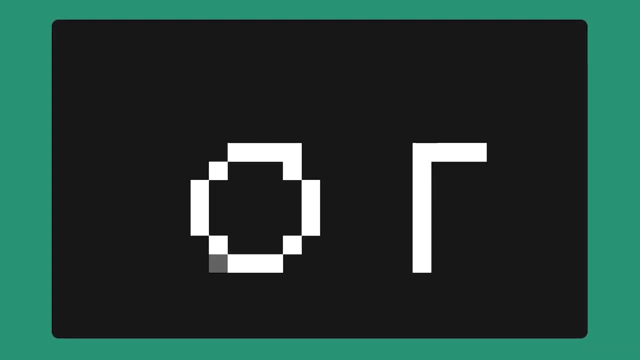 a fun new app that provides an inclusive experience for people with all abilities to express, connect and share with others. Expressive Pixels originally came about from a desire to provide a means of expression. For some people, verbal expressions may be challenging, whether because of speech disabilities. 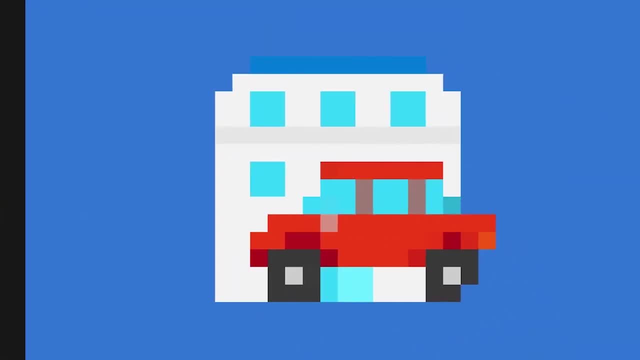 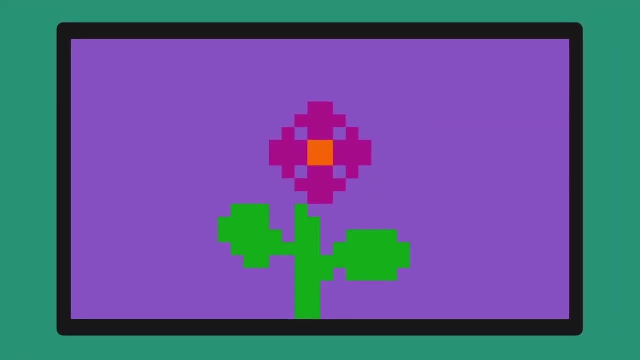 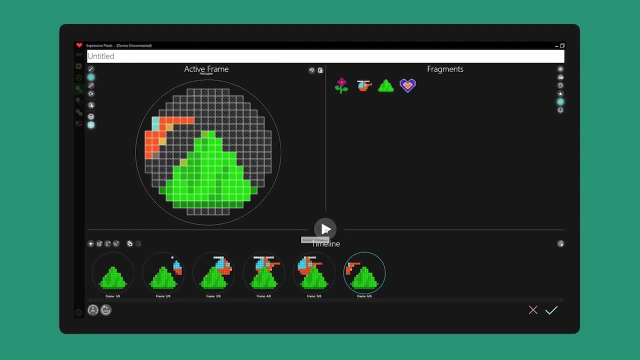 or they are just less comfortable with it. Often a visual statement, through creative and artistic expression, can communicate as much or more than words can ever say. The result takes into account neurodiversity in lowering barriers. With Expressive Pixels, you can create your own animations. 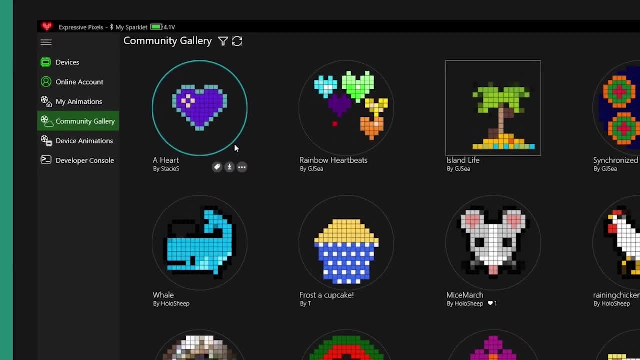 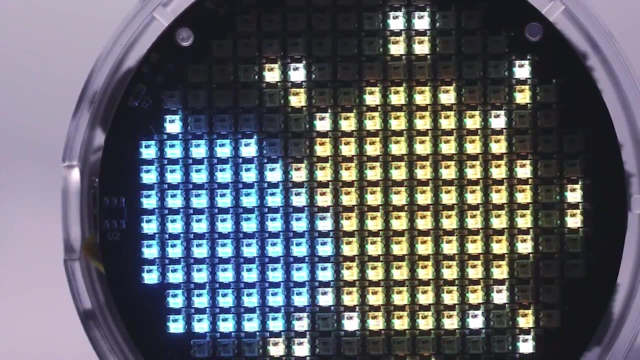 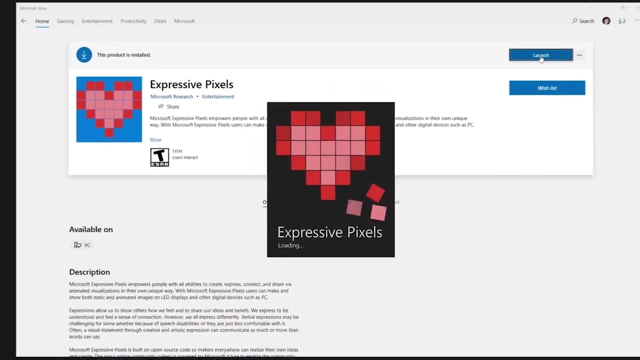 or use animations from our online community gallery and make them come alive on simple LED display. devices can be downloaded for free from the Microsoft Store on your PC. Download the app today. Start creating and expressing yourself. You can learn more by watching the tutorial videos on our website. 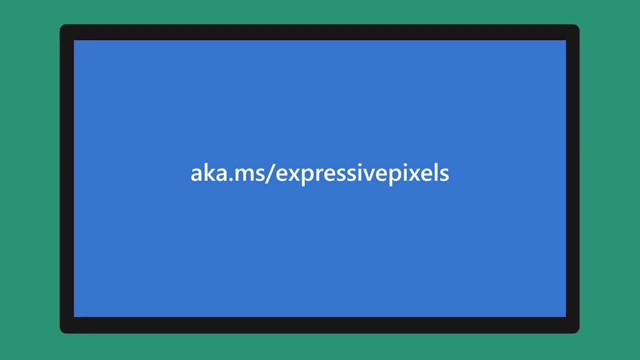 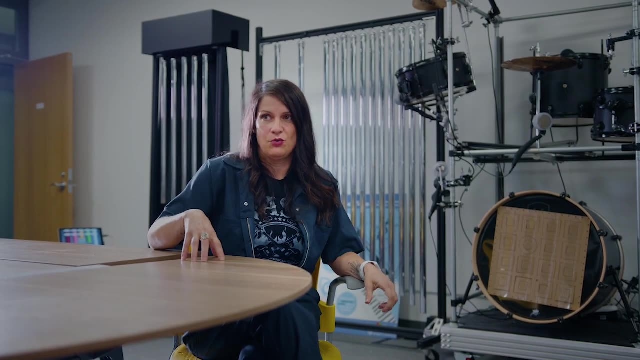 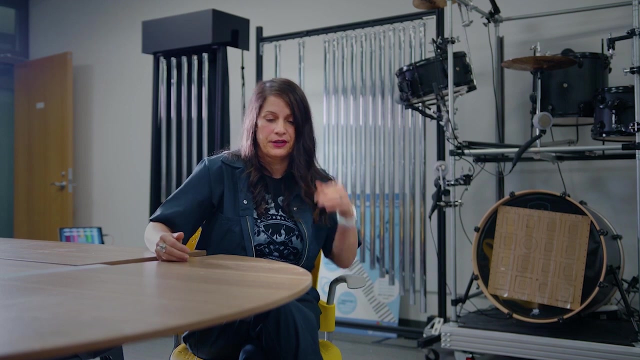 akams//expressivepixel. You'd think it would be obvious, if you were going to do design work or R&D, incubation work, innovation work or whatever, that you would understand the community that you're designing for. It's not always obvious. 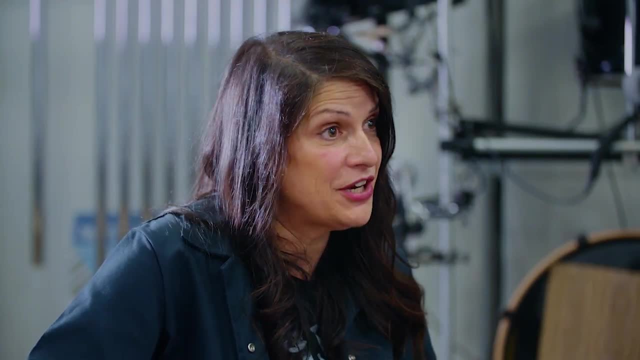 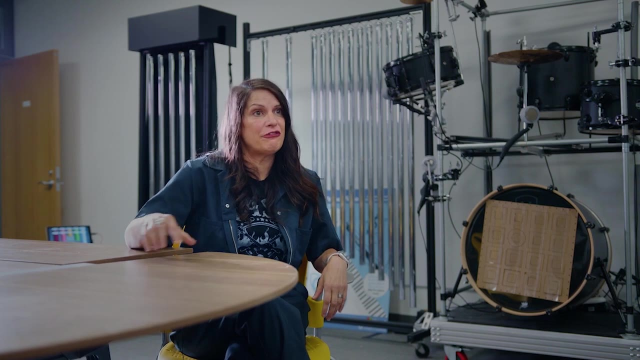 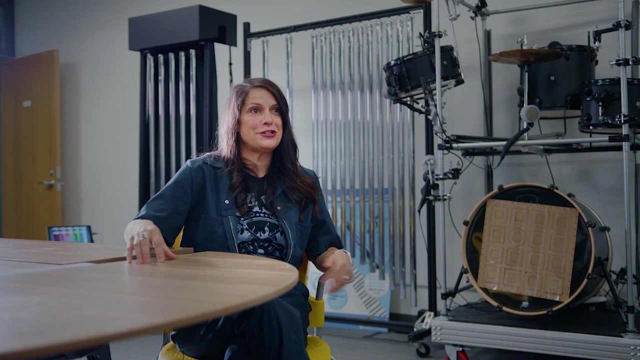 Our mission at Microsoft is to empower every human and organization on the planet to achieve more, So that word every is really where we focus. That means every human, Not just humans who don't have hard problems to solve When you build relationships like we do with our creative collaborators. 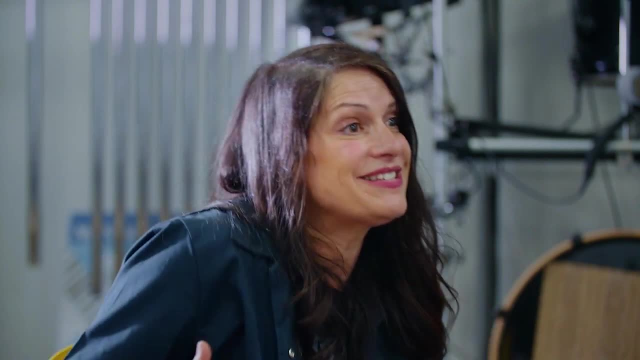 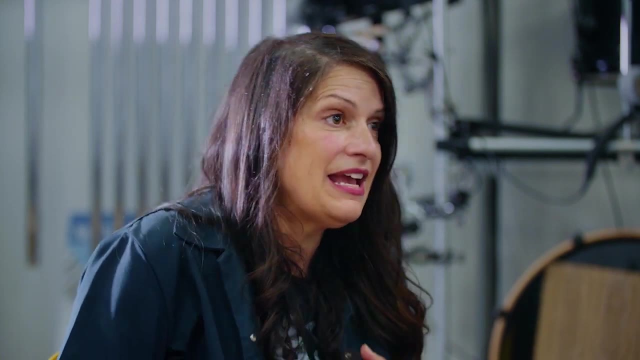 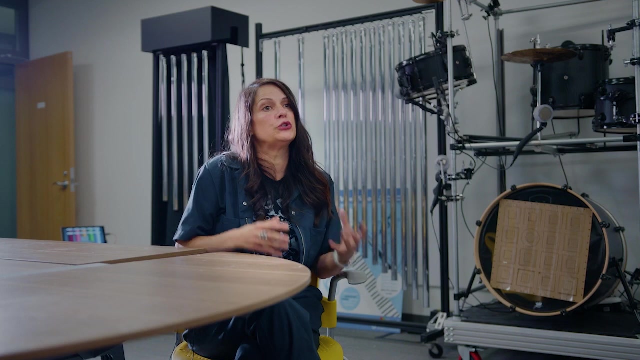 and with our community, you're invested. You're deeply, deeply invested in their well-being as your friend, your collaborator and your fellow human being. And so that sense of investment, purpose and empathy is what keeps everybody. That's the glue. 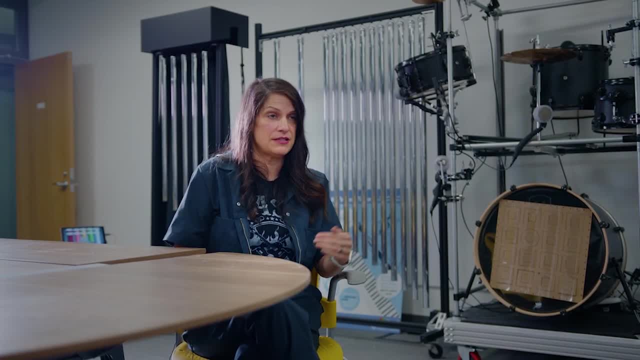 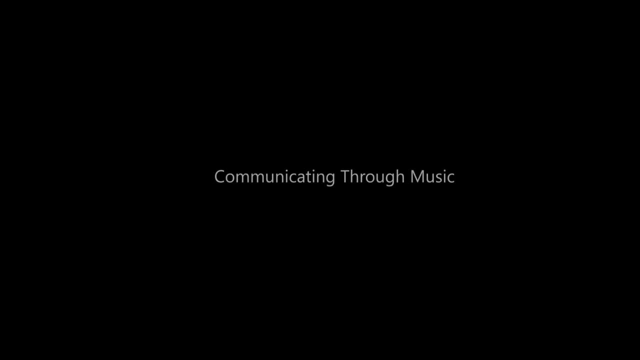 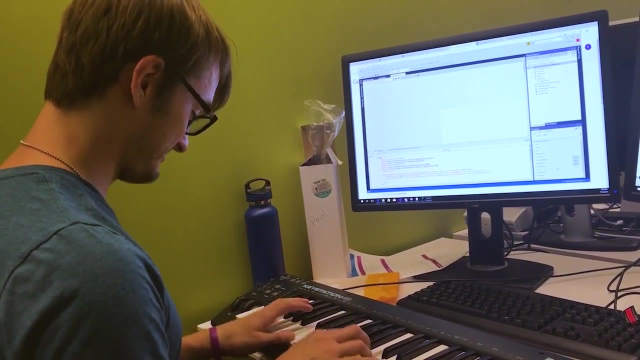 That sense of purpose, that sense of common purpose, is the connective tissue for all of us working in this space. Music is a primitive and powerful means of human communication and expression. Through it, we can share emotions, experiences and meanings with people across cultures and languages, and even across time. 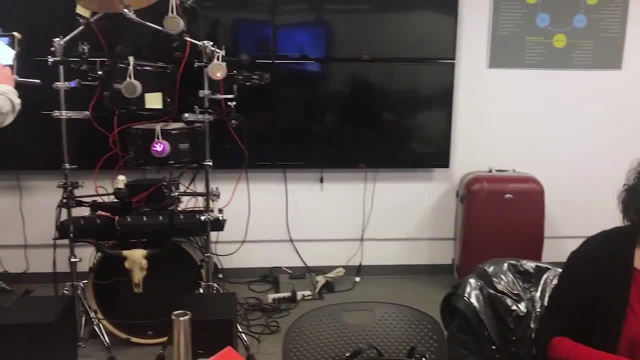 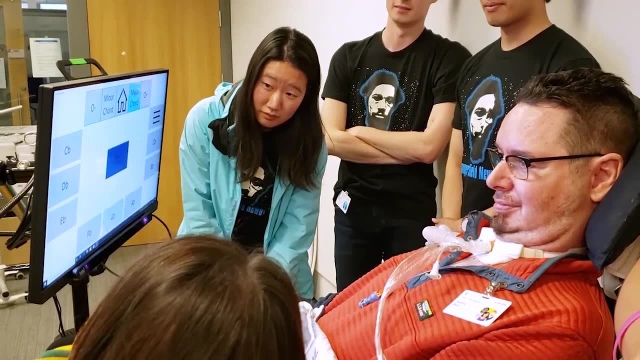 For the last five years, we've been experimenting with a number of approaches to inclusive music in support of people with little to no motor ability who may also be experiencing speech loss. The projects I'm going to show you next share one primary input constraint. 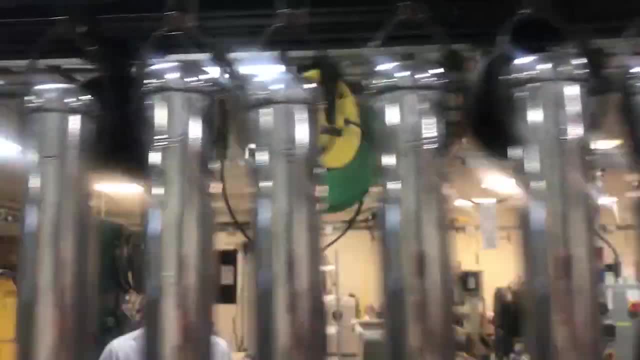 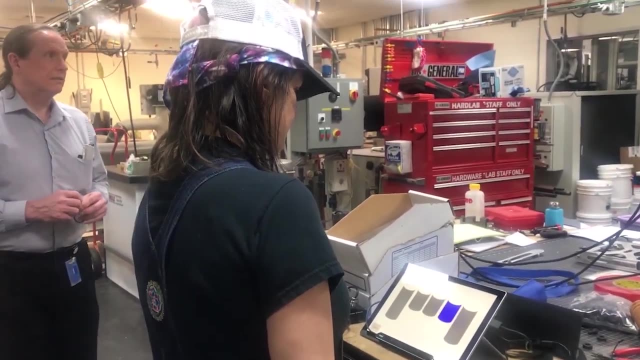 They have to be able to be played using just the eyes. That is no speech, no other movement. The Hands Free Music Project is an ongoing collaboration between Microsoft, local musicians and the ALS community. It includes a suite of eye-controlled instruments and playing interfaces. 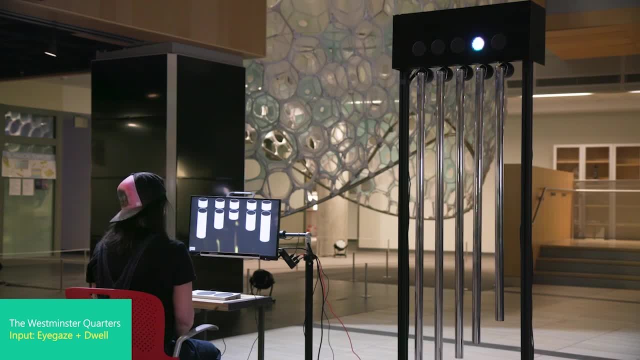 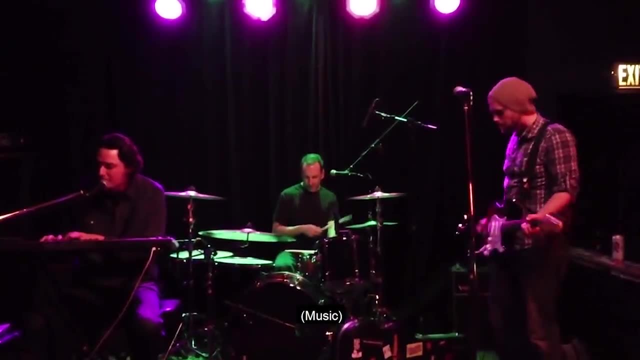 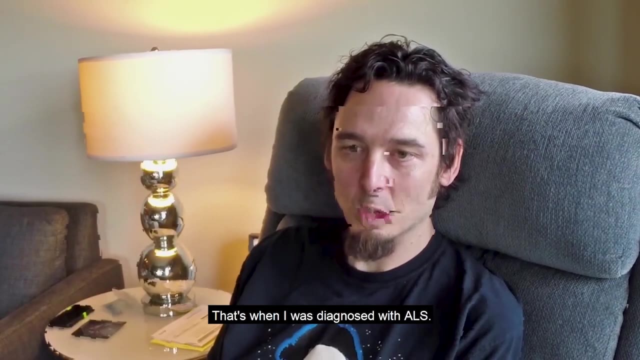 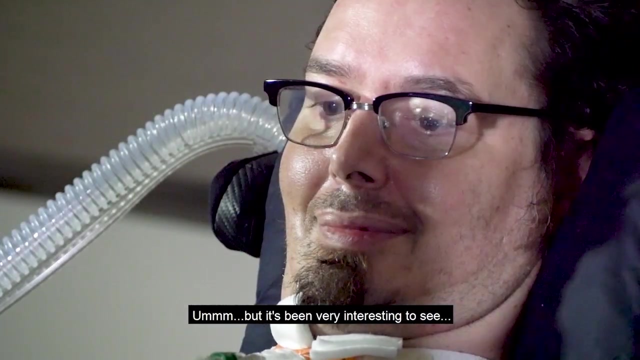 to support composition, performance and live collaborations. We are Dangerfield newbie. That was the day my world was turned upside down. That was when I was diagnosed with ALS. Obviously a lot of negatives here, but it's been very interesting to see. 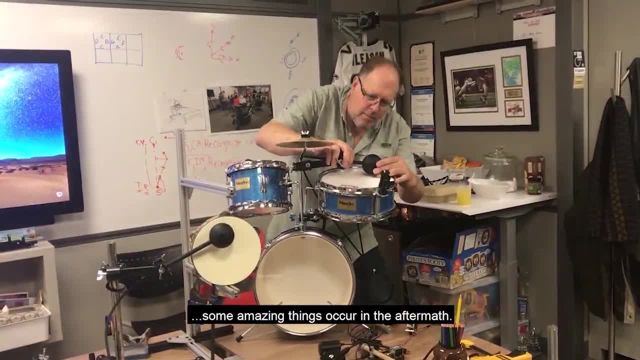 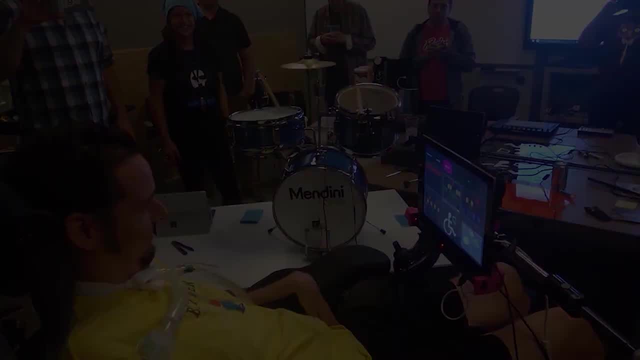 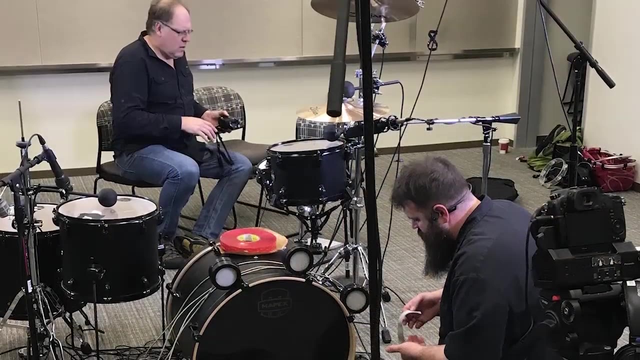 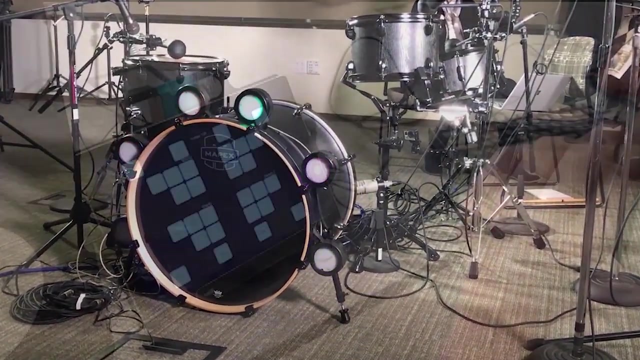 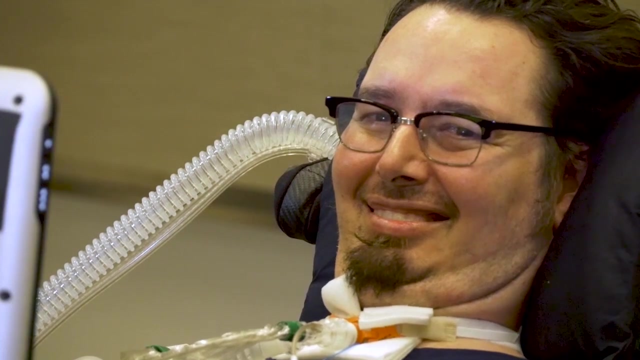 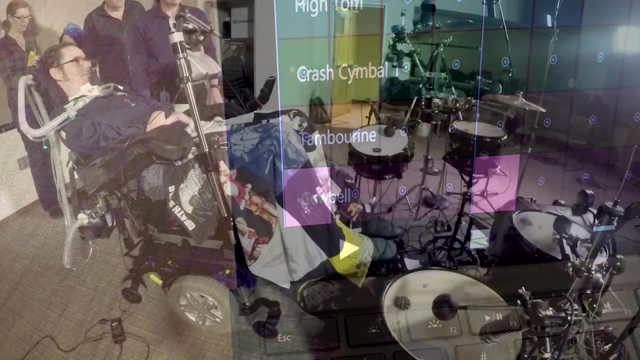 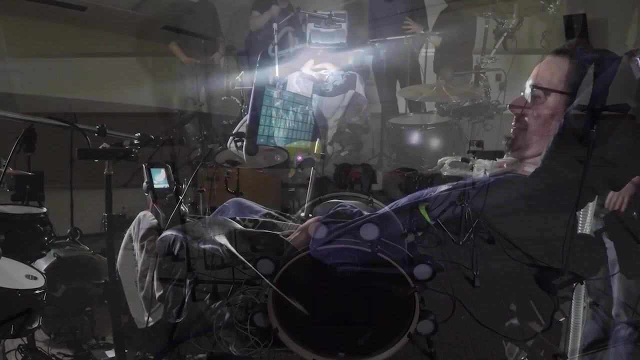 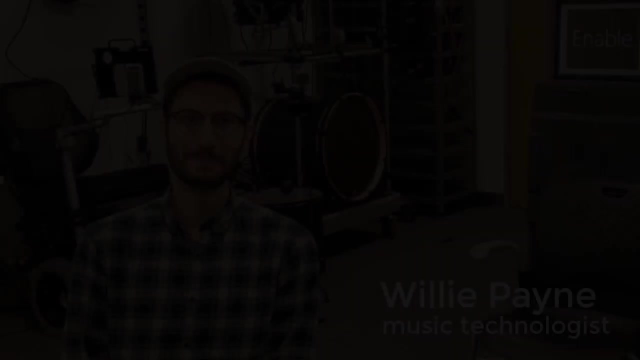 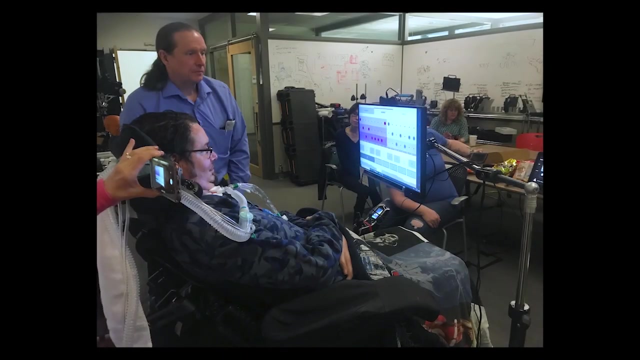 some amazing things occur in the aftermath. Do you enjoy listening to the music of the world? The Cyclops is an eye-controlled instrument designed by music technologist Willie Payne during his summer internship with the Enable Experiences group here in MSR. Willie built the Cyclops to support improvisation and performance scenarios for musicians who 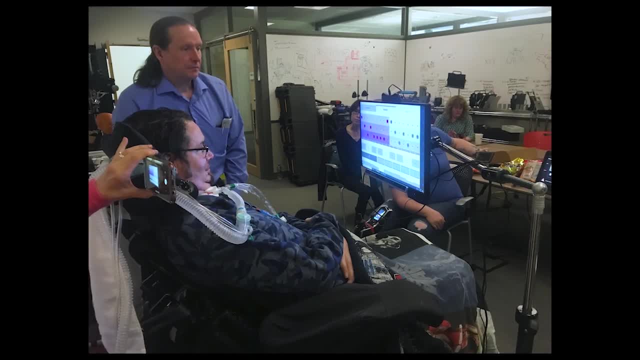 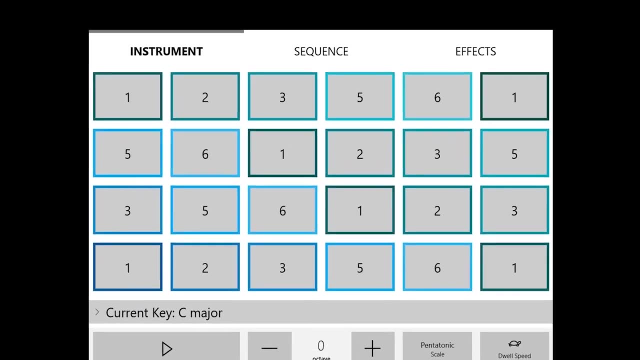 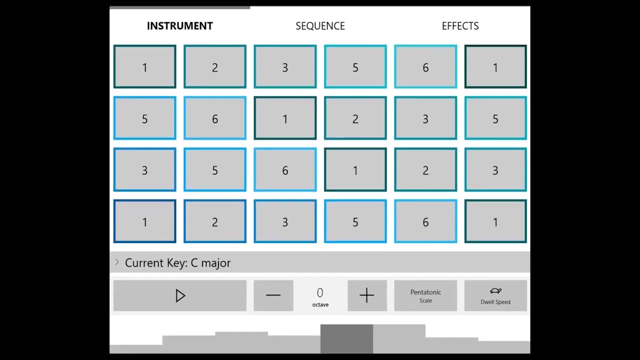 only have control over their eyes And yes, Willie is doing his entire demo using just his eyes. The Cyclops has three main screens: instrument sequence and audio effects. The instrument page is the primary page for producing sounds. The tiny red dot is where the eye tracker detects my eye gaze. 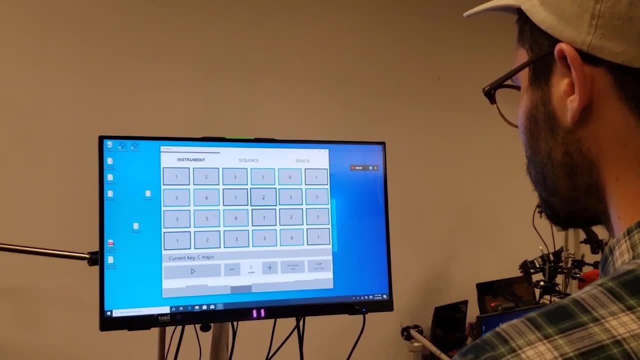 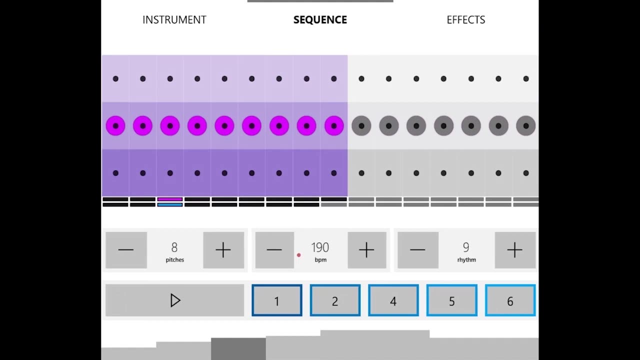 When I stare long enough at a button on the screen, it will cause it to press playing a sound. The sequence tab contains extra controls for playing with the loop. We can change the tempo to affect the speed of the music. We can add accents to increase the volume of individual notes, or rests to silence portions. 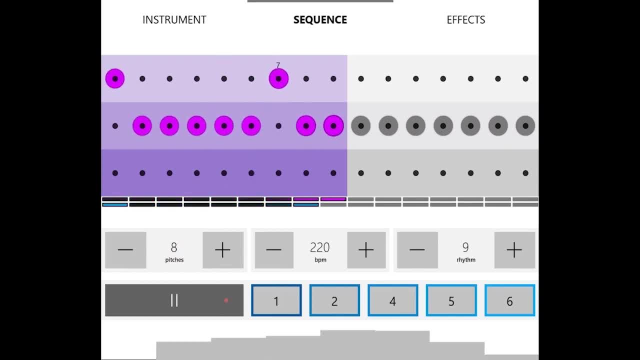 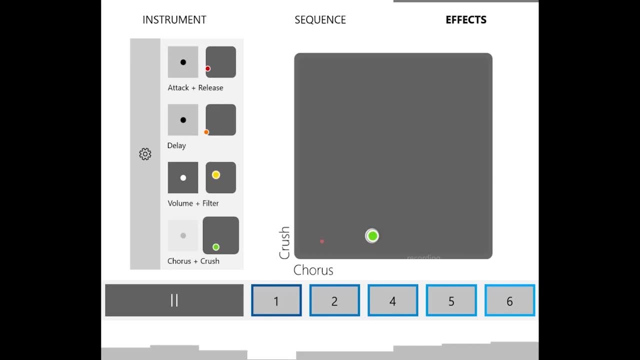 of the loop. On the effects page, we can fine tune how our sound actually sounds With just a few controls. the Cyclops is able to control the speed of the music. We can change the tempo to affect the speed of the music. 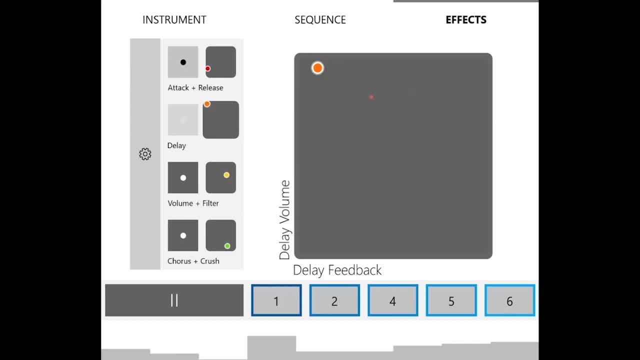 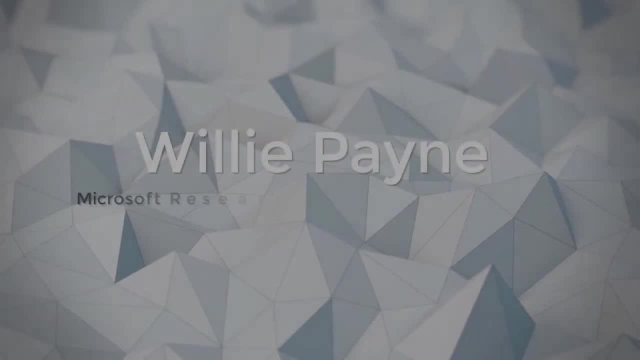 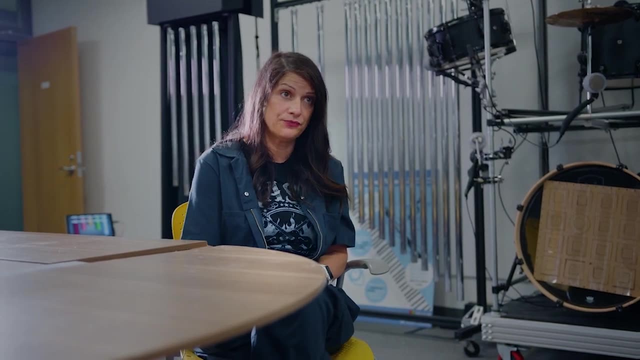 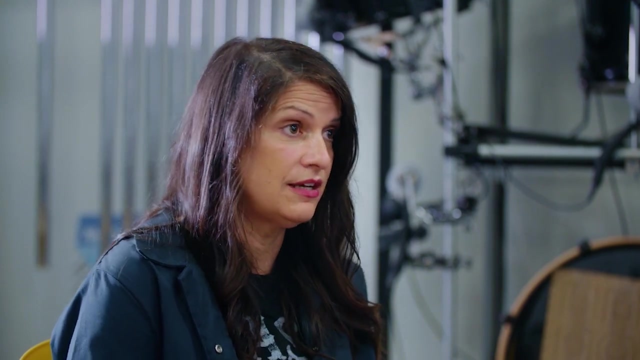 We can add accents to affect the speed of the music. The Cyclops is an expressive instrument capable of a wide range of sounds, all controlled and triggered just with your eyes. To me, one of the best ways to learn is to do And the way that you learn how you can best serve a user community who is facing profound 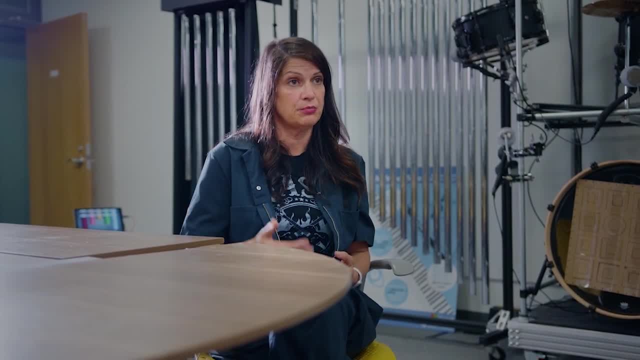 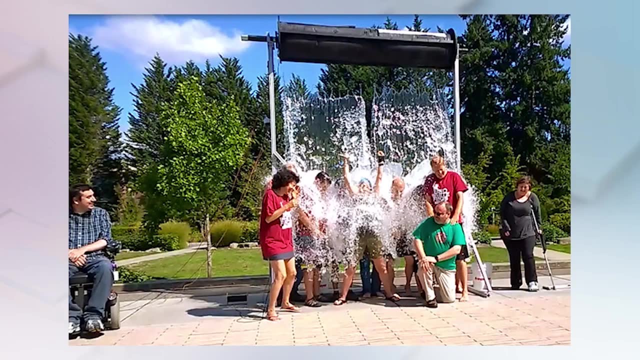 constraints due to ability loss because of disease progression. the Cyclops program is the best way to learn And it's just a great tool to use. progression is to meet them, listen to them, observe them and take part in as many activities. 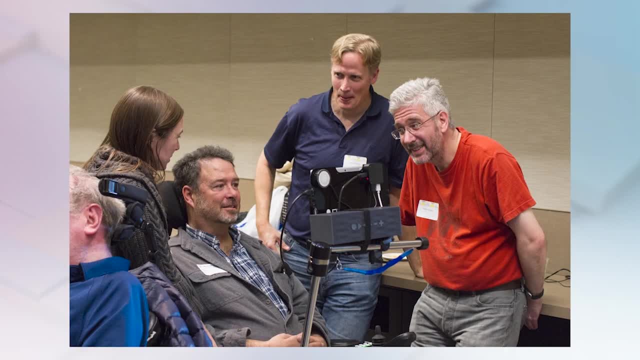 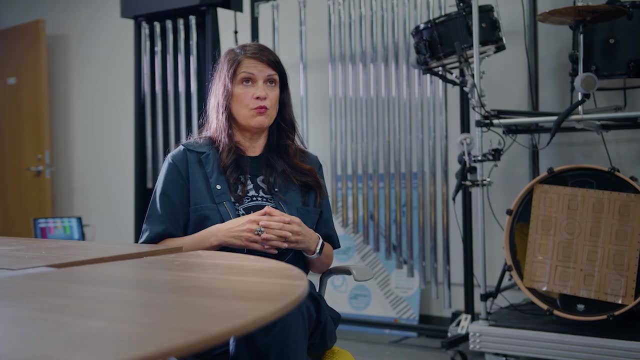 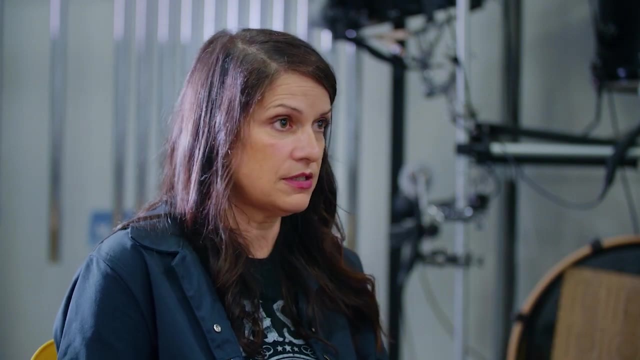 as we can, because experiential observation is super critical, especially when you're trying to decide where you're going to focus your efforts. Our space in general. we do a combination of things. We do formal fundamental research in computer science, write papers, conduct studies, create. 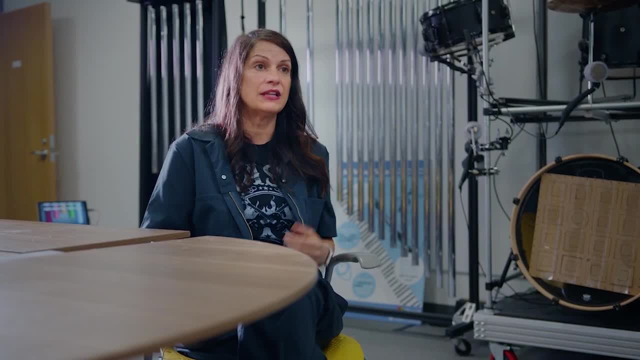 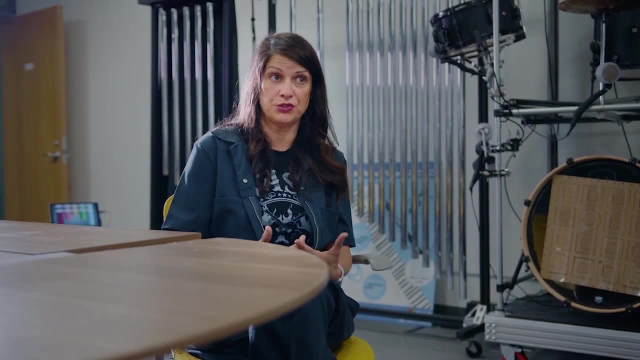 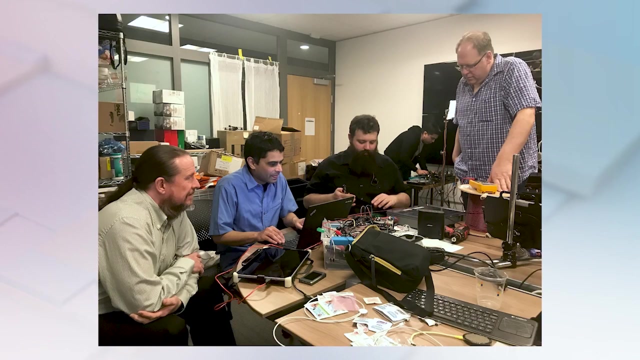 prototypes, proofs of concepts, evaluate them and release those findings into the world so that we can better inform the design of assistive and expressive technologies in the future. We also incubate our own designs and technologies, and we work iteratively and collaboratively. 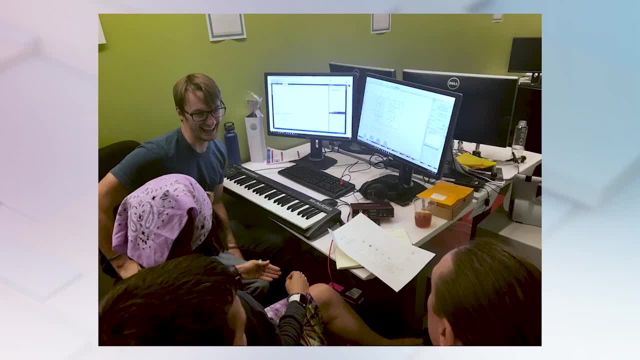 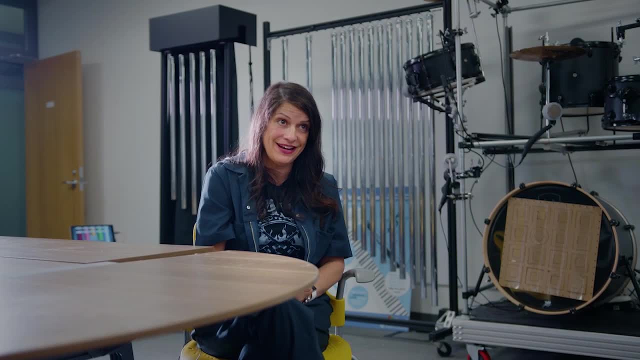 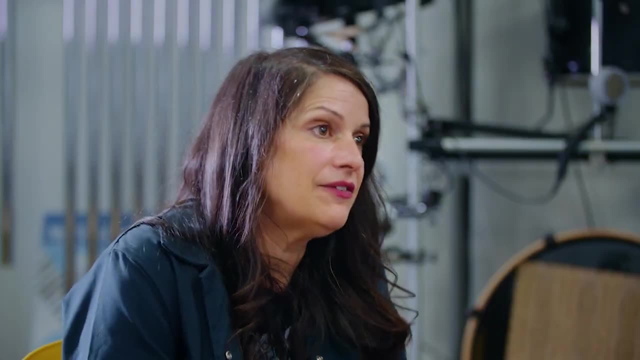 with our user community to direct those activities. We are honest about what we learn. We put everything out in the open source or in the public domain. We share, We mentor students, We mentor talent. We do all of those activities because that is how the progress is going to happen. 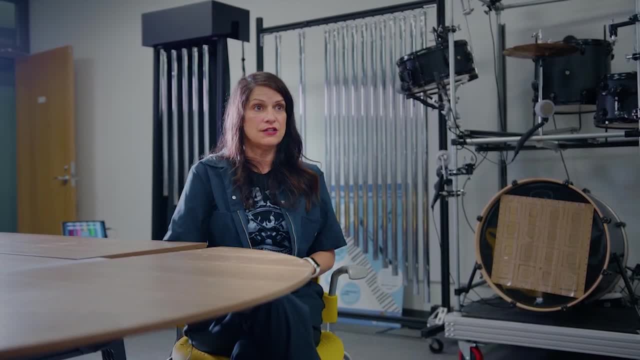 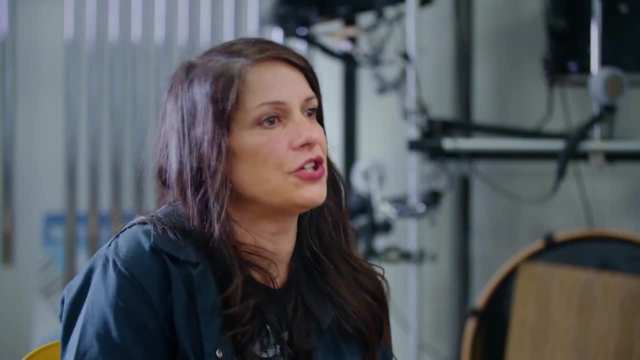 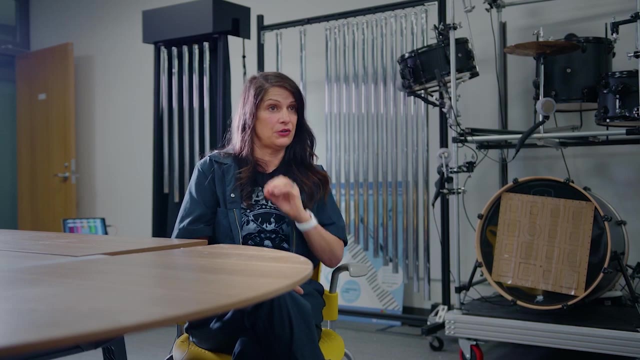 What way can we use technology in service to our goal of restoring or reinventing lost capability If you don't center your user community in every single activity, every single research, design or development or innovation activity that you have? We're not going to do that. 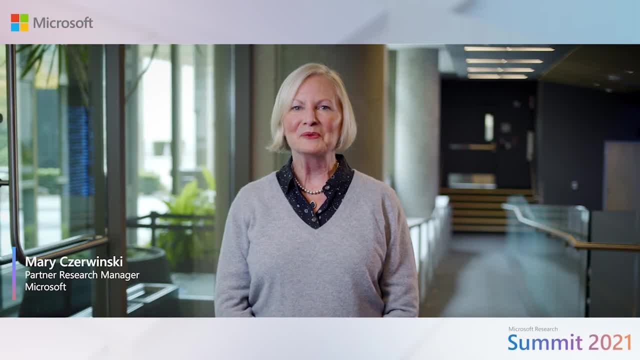 You will not be successful. Finally, we'll hear from Ken Hinckley, a senior principal researcher who's also from the EPIC group. Ken is going to talk with us about how devices can help to make sense out of our increasingly complex work lives and interactions with others. 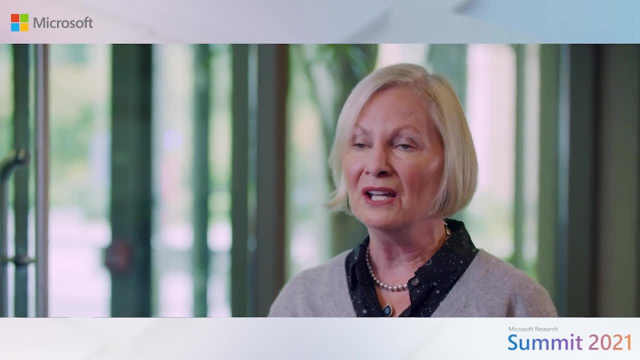 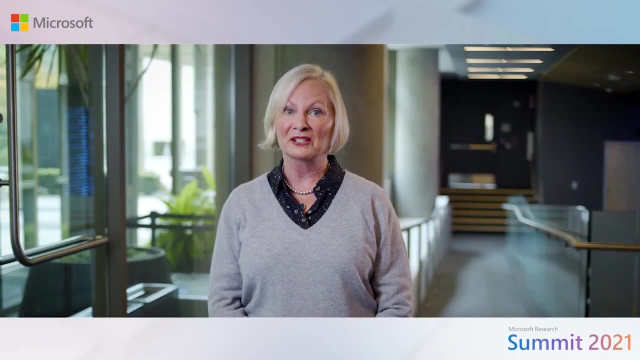 He's worked on everything from sensing techniques, cross-device interaction to novel device form factors. Today he's going to tell you a little bit about Surface Fleet. This technology has implications for something many of us can relate to these days: the home. 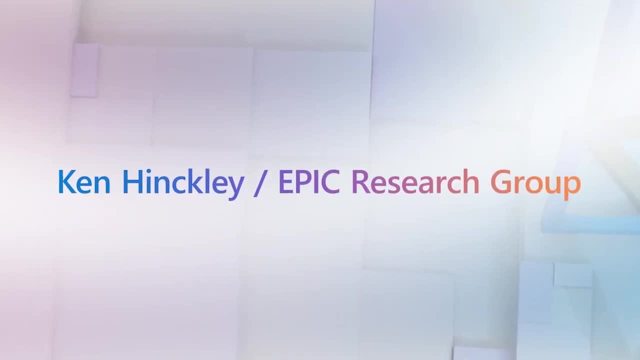 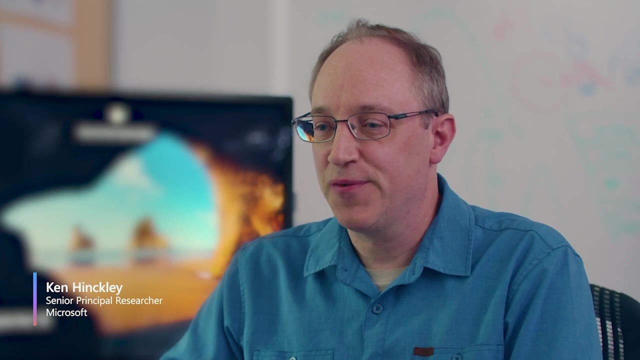 workspace. I'm Ken Hinckley. I work here at the lab at Microsoft Research. We innovate across hardware, software and the human experience. We do all kinds of cool research in terms of interaction with devices and also studying how people use devices and also interact with one another. 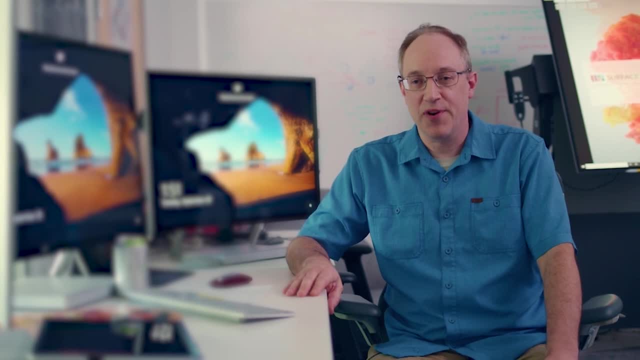 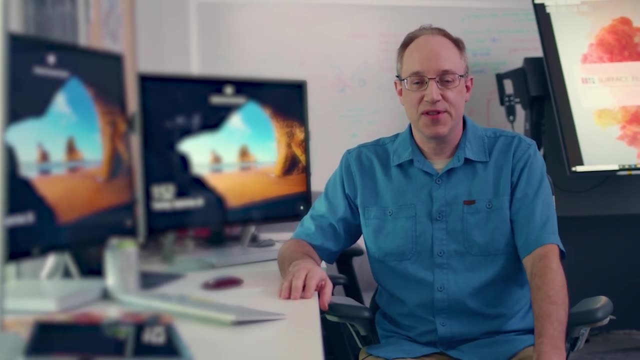 So we study collaboration, We study how people work in productivity, We study how they actually use their devices in terms of just picking things up, looking at them, moving them around, all this kind of stuff. So we have lots of very fun things that we do. 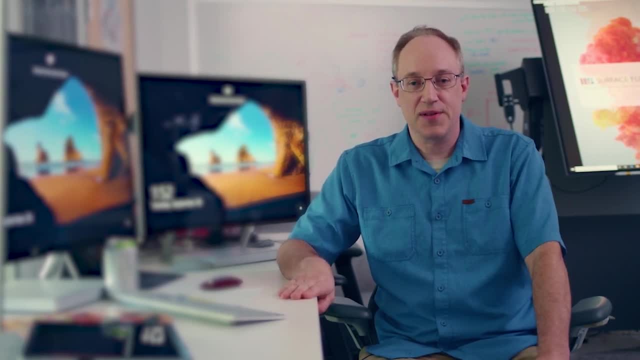 One of the things that we do is we do a lot of research. One of the exciting areas that we work in a lot is sort of figuring out how to leverage smarts about the world around us, so bringing in things like sensors or sort of unusual. 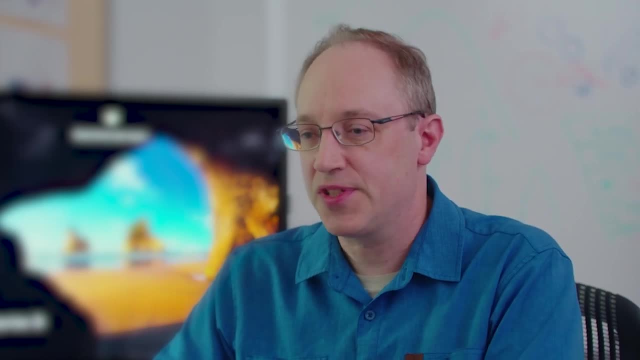 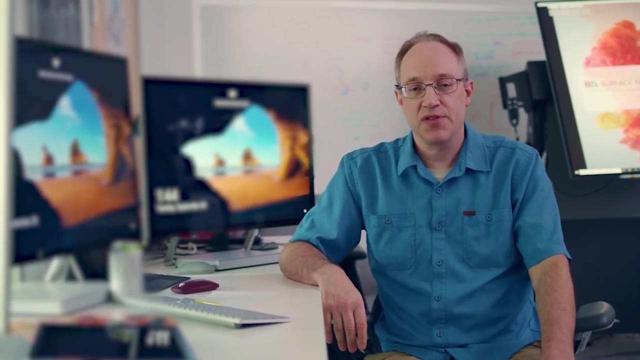 inputs like speech or gaze or camera inputs, that kind of thing, to have a more natural way of working with our devices. The actual name, EPIC, is an acronym, so it stands for Extended Perception, Interaction and Cognition. So we work across all these topics. 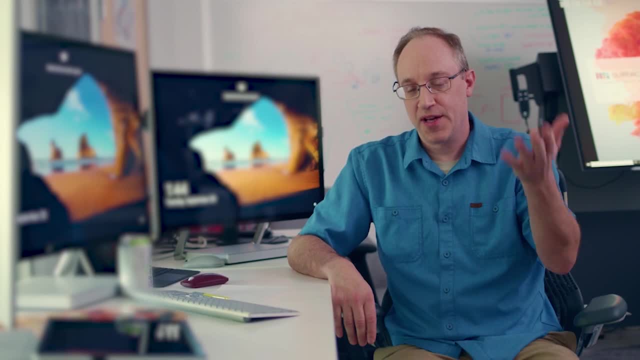 So the perception is the human perception of how they see the world, how they feel the world, how they hear the world. The interaction, of course, is the human perception of how they see the world, how they feel the world, how they hear the world. 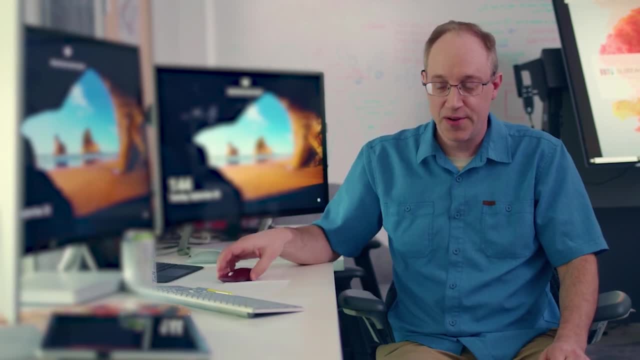 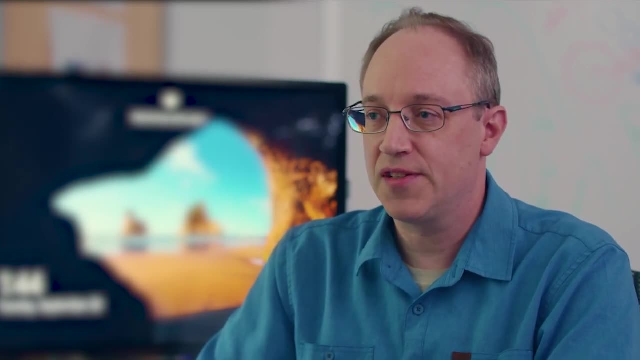 The interaction, of course, is interacting with things around you. moving things like even just a simple mouse or picking up a device, that's an interaction. Looking at someone: that's an interaction. You might not think of it that way, but if our computers and devices can sense these, 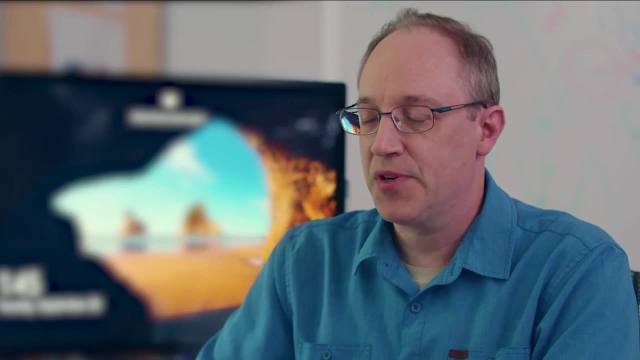 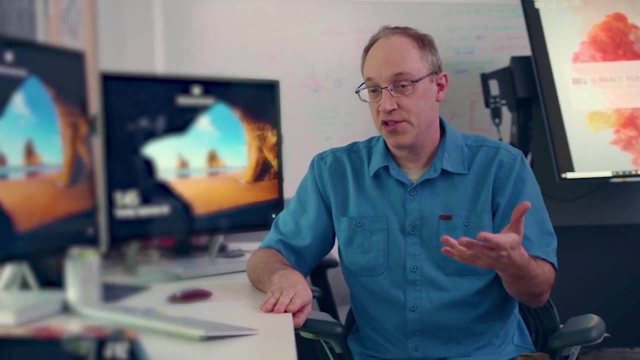 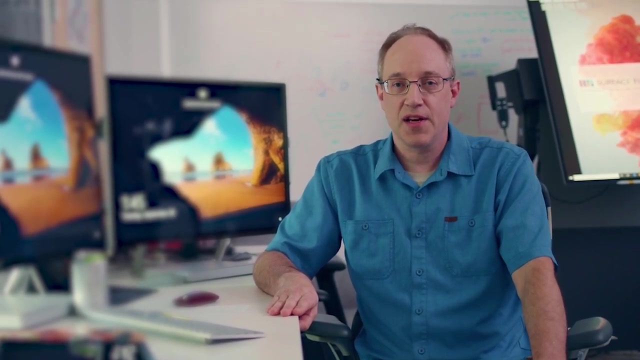 things and respond to them appropriately. it makes it so they can be much smarter about how they interpret what we're doing in the world. And then the cognition part ties into not so much artificial intelligence but actual human, genuine intelligence. right, And how people think about the world, their tasks, how they think about interacting with. 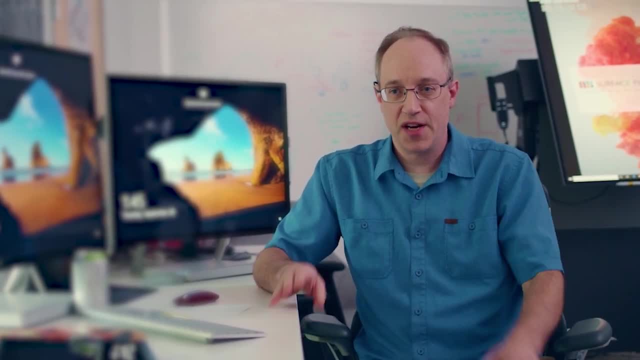 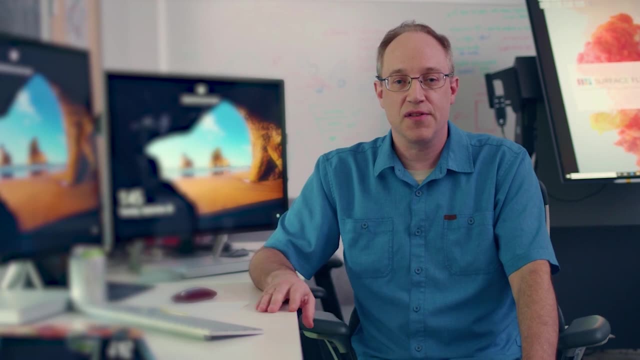 one another And a lot of this it's not just in your brain, but it's actually externalized to the world. So the E in EPIC stands for this externalization, or this extended nature of intelligence, where your artifacts in the world actually encode information. so you don't have to remember. 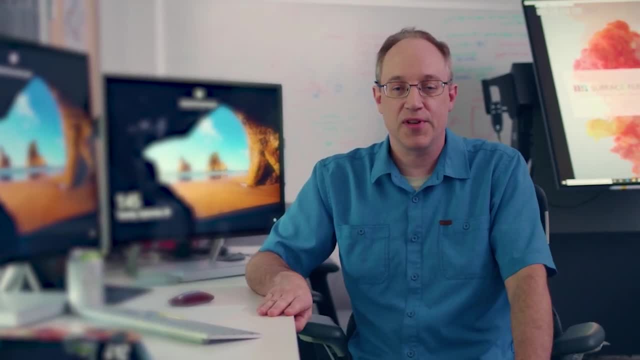 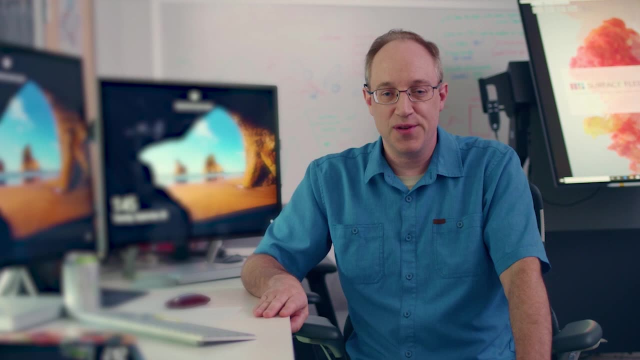 something. You just stick it on a Post-it note and you stick it on your monitor and that's externalizing that reminder. So that's sort of the whole scope of the research in the group. So, for example, we've contributed to the New Future work in terms of studying what people 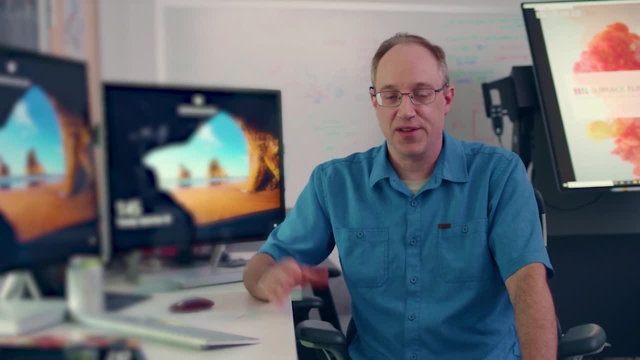 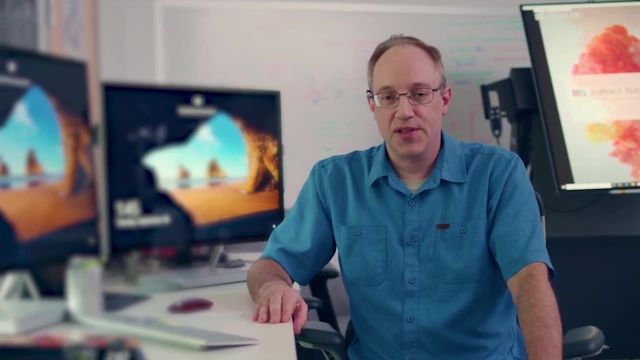 do with their devices while they're working at home. What kind of tasks are they doing? How are they juggling tasks with their kids and their families and their multiple clients and all these things? We work across things like haptic feedback, for example. 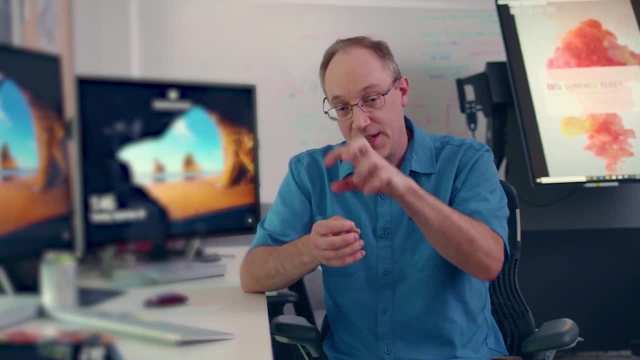 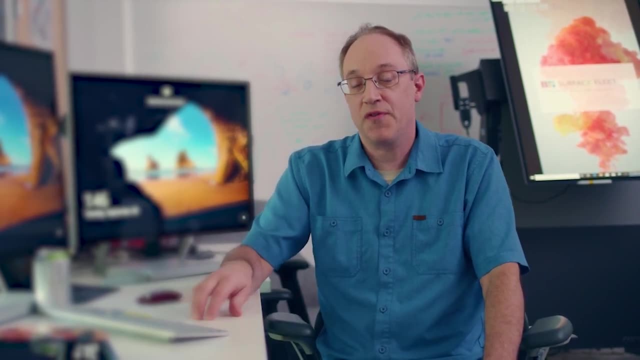 So devices that can actually respond to you, with you can feel tactilely what's going on in terms of if you're interacting with a virtual reality. you can feel objects in the world, You can feel the shape of things, maybe if you're a person who's not sighted, 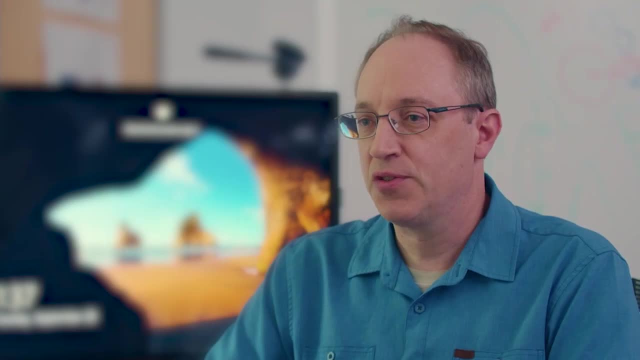 So we do all kinds of things along those lines. So we're kind of hurtling towards this future where everyone has these multiple devices and we're trying to figure out what's going on in the future. So we're kind of hurtling towards this future where everyone has these multiple devices. 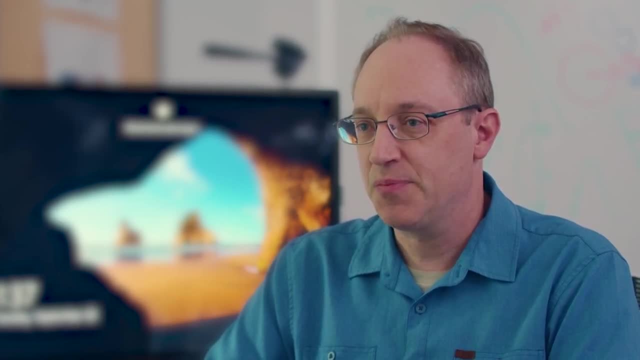 and we're trying to figure out what's going on in the future. So we're kind of hurtling towards this future where everyone has these multiple devices and we're trying to figure out what's going on in the future, And this is a trend that's been particularly aggravated by this new future of work that 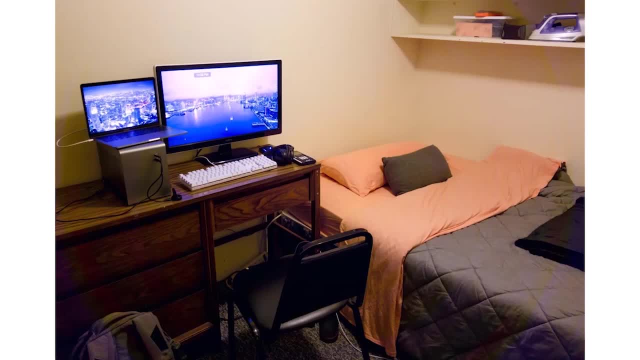 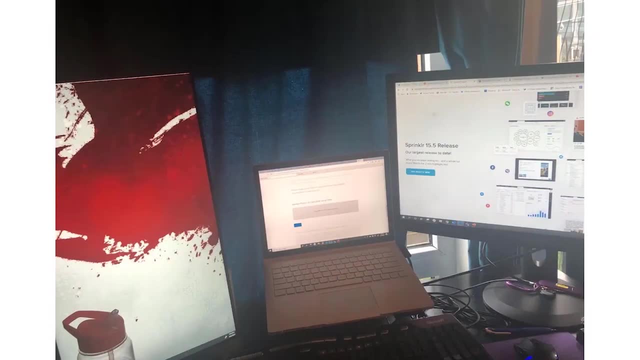 we find ourselves in where, suddenly, we're working at home. You've got your screen there, maybe you've got your kid's iPad there, Maybe you've got another computer at the ready and you're just trying to get your work done across all these devices. 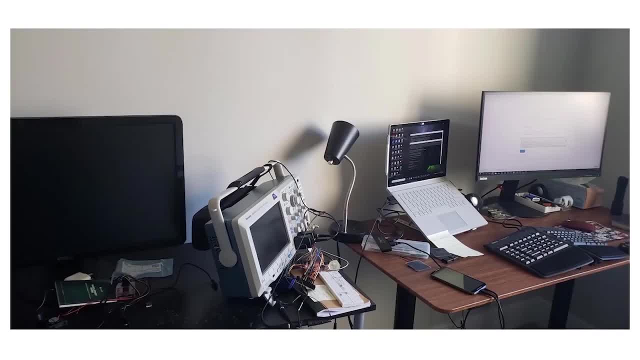 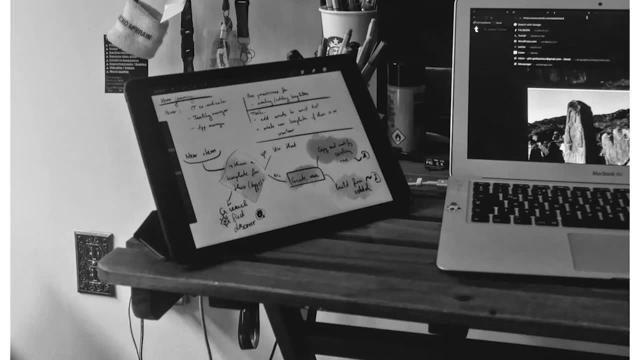 And it's not unlike how people might work in an office space where they're spreading out information across multiple pieces of paper. They're trying to lay out their thoughts, organize things and kind of this informal way of putting things in space. and so multiple devices. 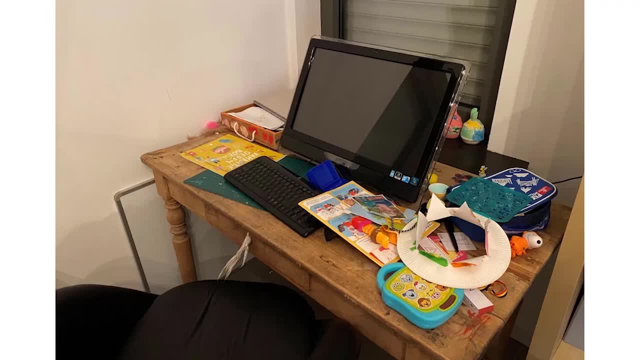 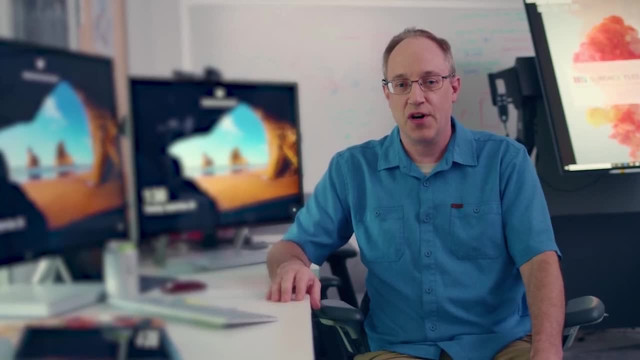 can serve this same role. so, in a sense, people you know they like to use space to think, so we like to think of ways to do that in the digital world as well. the main idea of surface fleet is to make it easy to work across these multiple 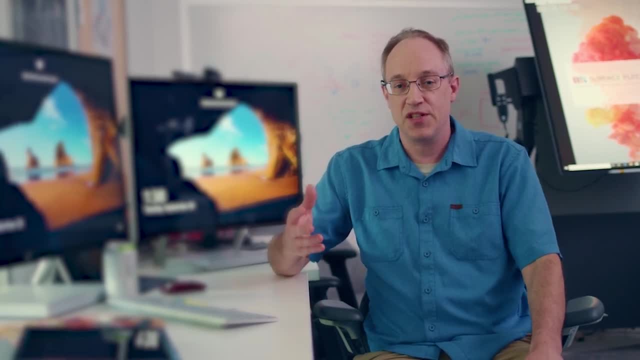 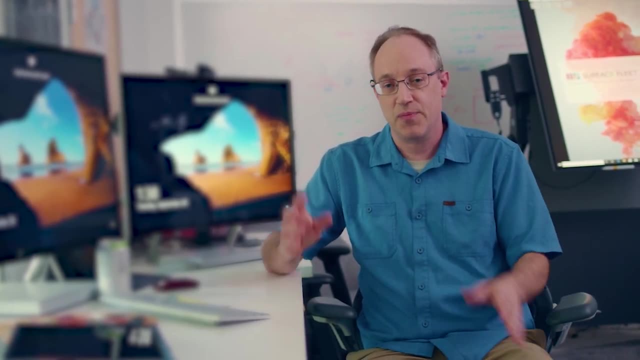 devices and sort of. the objective is to make it easy to transition, you know, whatever activity you're working on, from one device to another, or from one location to another, or even to pass it off to another person or to defer it to a future time when you're actually ready to work on it. so having both 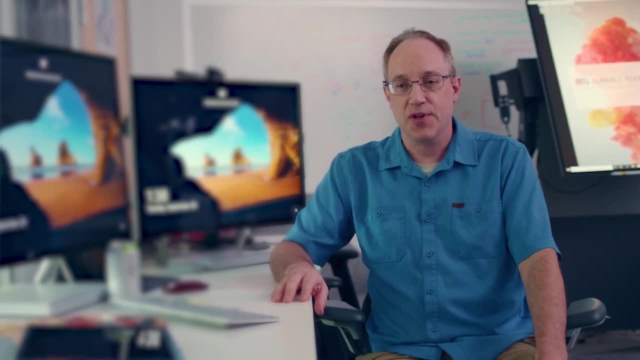 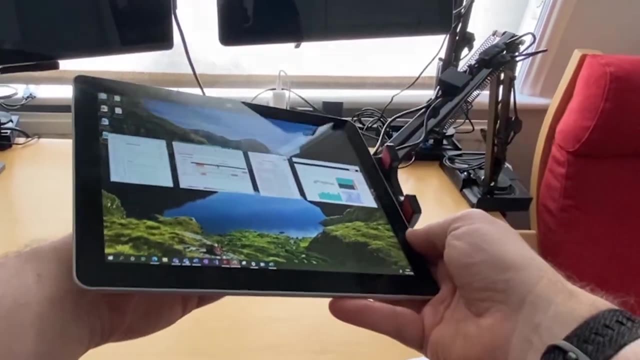 technologies and user experiences that speak to. that is something that we're looking at very closely. so, in particular today, I can talk a bit about something we're doing called the ultimate flexible workspace, which is a device concept we've been exploring which makes us: you can just walk up to your, your, your. 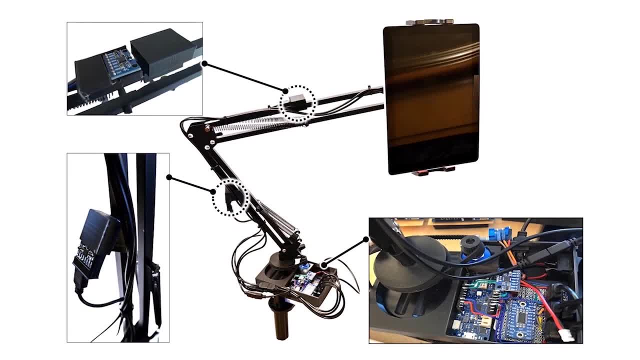 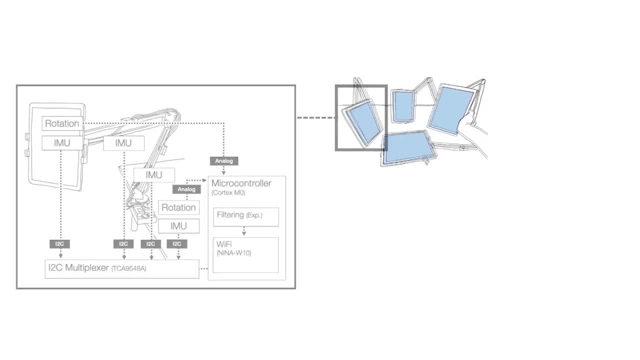 workstation at home with your tablet. you just plop it into this armature- that's kind of like an articulated lamp, and then you can kind of posture your tablet anywhere in space. and then the really cool thing is when you have multiple these they're all aware of one another and they're all aware of one another. and 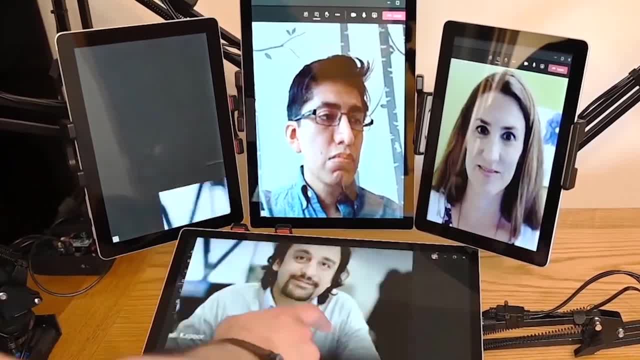 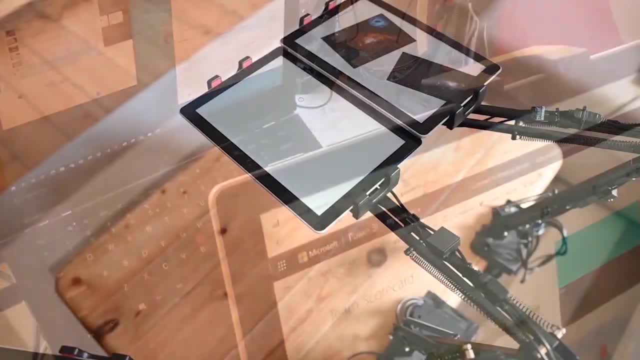 you can sort of juxtapose them, you can split them apart, you can put one down, one up, so you know, just depending on your task and what you're trying to do and what information you want to see side by side. it makes it super easy to dynamically create these formations of devices, because it also senses these. 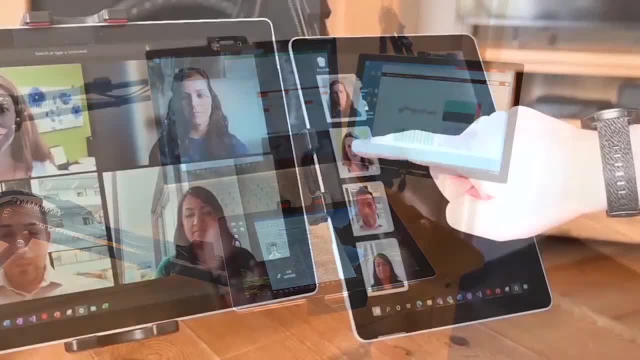 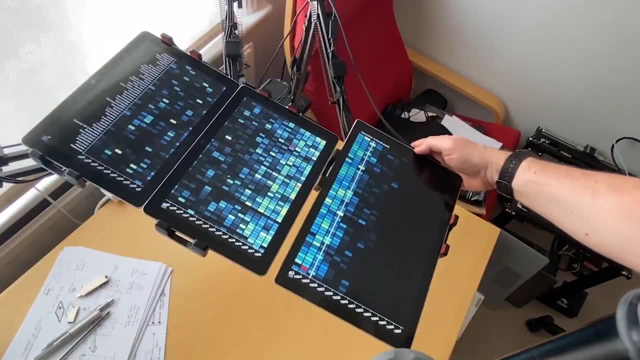 transitions. all you have to do is put the device next to another one and it says like: hey, you want your document here, and then you can just drag it over or you know whatever you want to do, so it it makes it really easy to work in these kind of ad hoc workspaces that we have in our homes, where often you know. 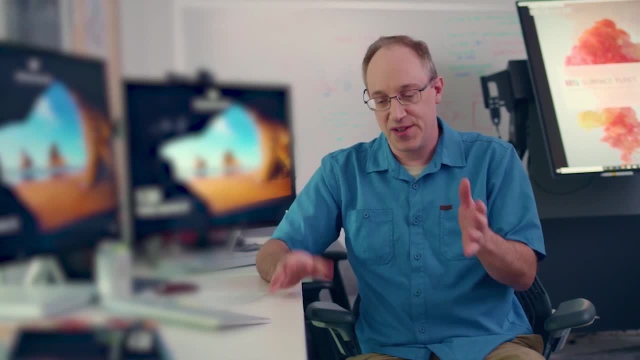 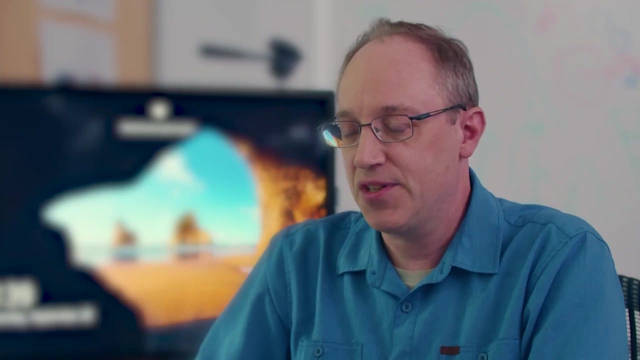 spaces are very limited. you might want multiple screens, but you're just, you're in this little you know sort of improvised desks in the corner of your living room somewhere, right. so, and making it really easy to work in those kind of spaces, which you know also can translate to the future when we get back. 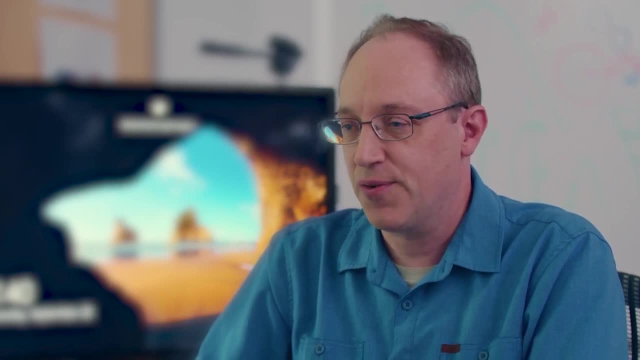 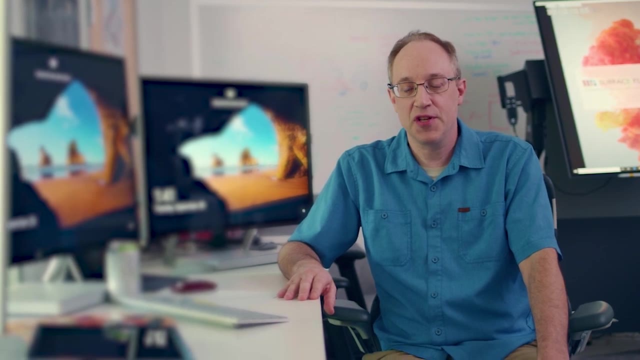 to the office and we're sharing spaces and in conference rooms and so forth. so in particular last year- which is actually during this, you know, pandemic remote work time- we had a visiting researcher by the name of Nick Marquardt, who's a professor at University College London- also happens to be a 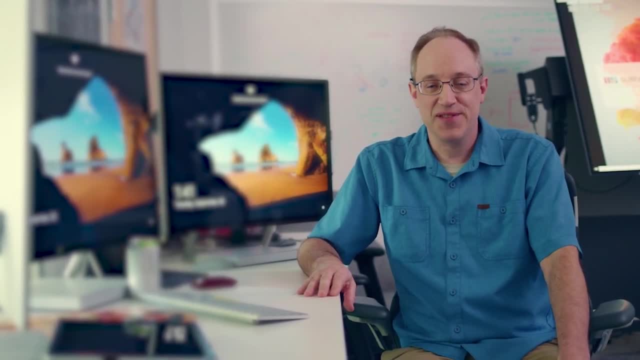 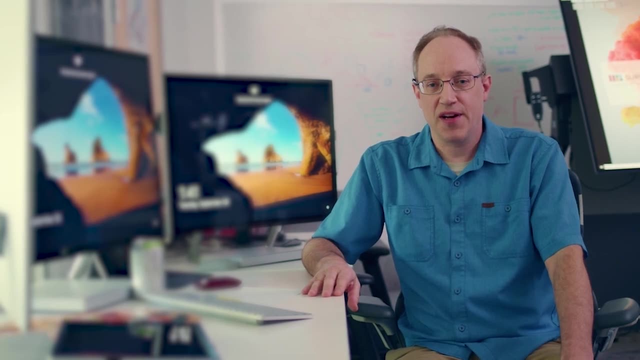 former intern who worked with me, you know, over ten years ago now, and so Nick and I have sort of done a number of projects over the year and he had this brainstorm about, you know, basically repurposing articulated lamps as a smart appliance- you know, desk appliance, you know- for the, for the work. 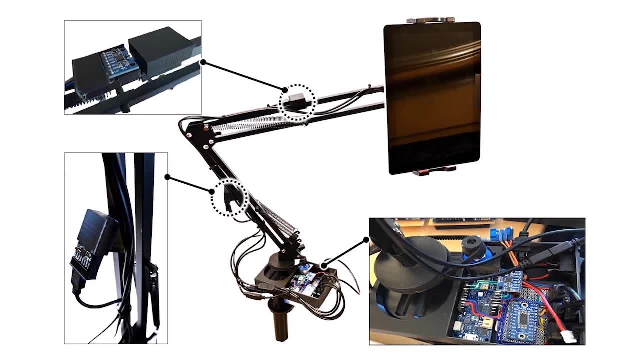 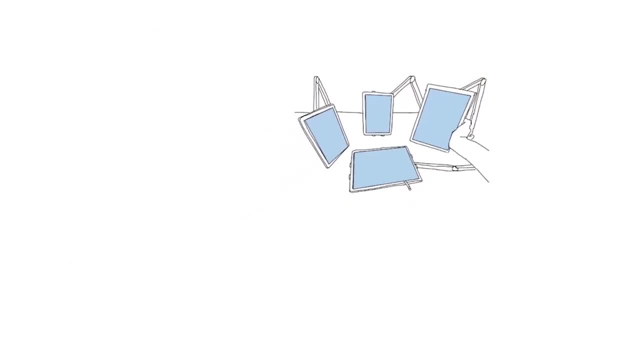 at home situation. so the idea is that you basically take. you know, we literally ordered these armatures off of Amazon, I think right, so they're like 20 bucks. just added some sensors to them which are just. you know, they're basically just simple motion sensors. it's the same as you would have in your smartphone, or 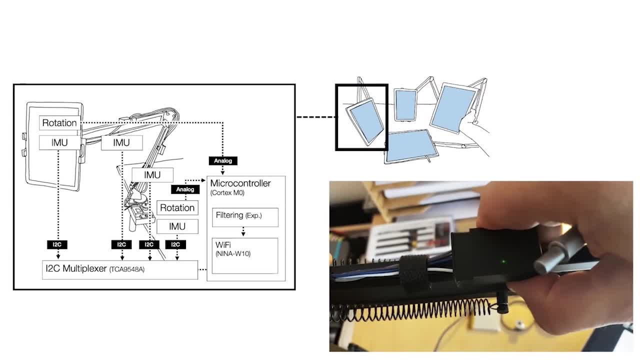 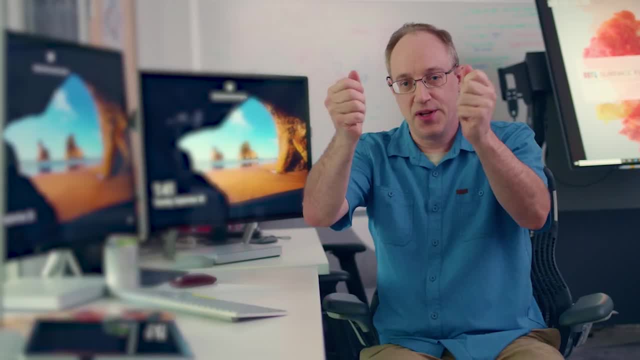 tablet already put a bunch of those on the. you know the different armature link there and then we can actually sense where the tablet is in space. so, as you, you know position it, you can let go of it. it just stays there. it knows this angle, it knows this position, it knows how it's postured relative to you, you. 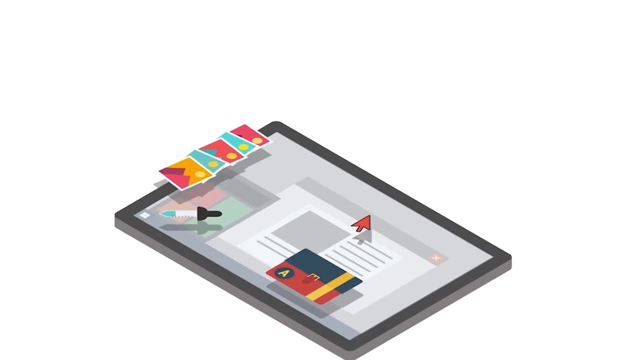 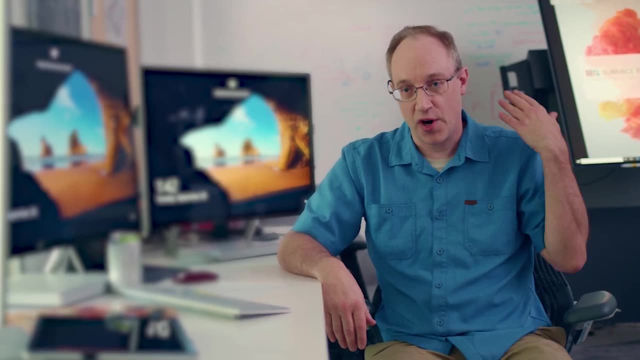 can put it over next to another device. if that one also has an armature, then that one also can know where it is relative to the other. so they have this kind of spatial sense of like who's nearby, just like you would be aware of if someone walked up behind you or next to you. you can collaborate with them. so